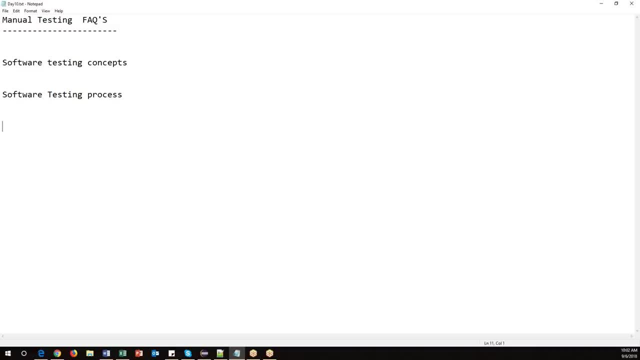 process wise, and then concepts and process and then project and project related questions. So first we will discuss about what are the different questions you will get in interview from testing. concepts and testing process means STLC, and then project related questions. Now let's go by one by one. So here I just write all the questions here, but I'm not going. 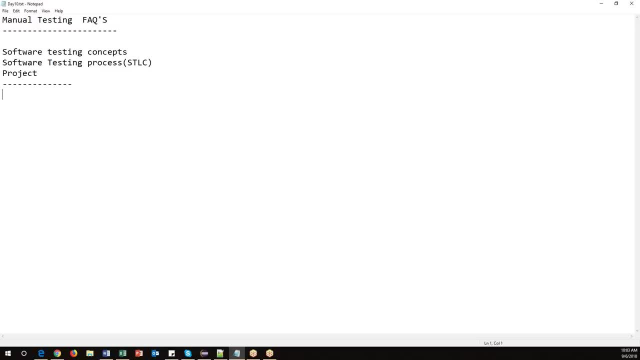 to write all the questions here. I'm just going to write all the questions here, but I'm not going to write all the questions here. but I'm not going to write any answers, but I'll explain that one, okay. So if you want to make a notes, you can just 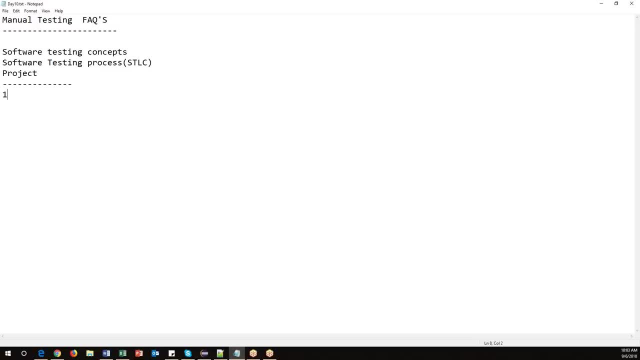 make it notes. Anyway, I will provide those questions in the documentation format. Okay, now let's see what are all questions I will get in interview. So first let us discuss about testing concept related questions. Okay, so the first question will be: what is the difference between SDLC and SDLC? What is the difference between SDLC and SDLC? SDLC- 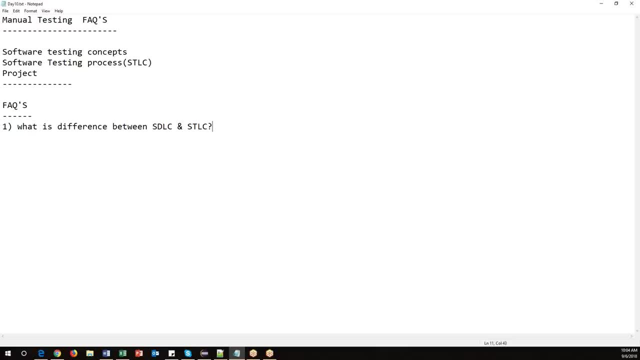 means software development lifecycle. SDLC means software testing lifecycle. So SDLC is talking about the complete software development process from the beginning to end: like requirement, understanding, designing, coding, testing, maintenance, deployment- Everything will be part of software development lifecycle. but SDLC is a part of the testing, like software testing lifecycle. What are 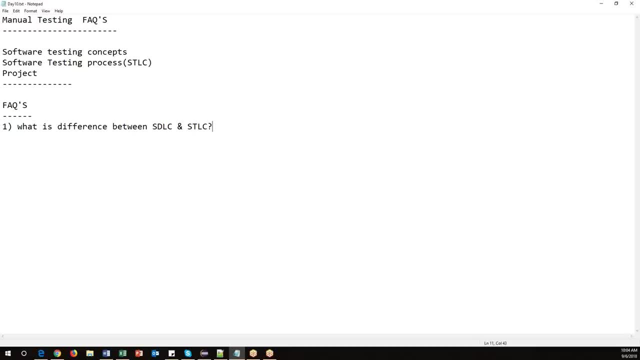 the different activities we perform as part of testing will be part of SDLC, like test planning, test designing, test cases design, execution of test cases, defect reporting. Okay, all these things comes under the SDLC process. So SDLC is talking about overall process of software development. 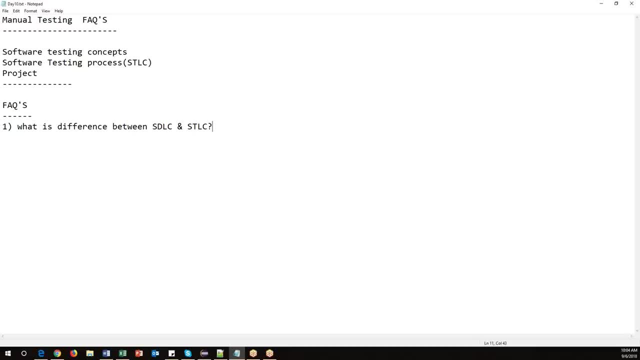 whereas SDLC will talk about the testing process in SDLC. So that is the difference between SDLC, SDLC and SDLC. Now the next question. So what is the difference between? what is the difference between? let me just write what is the difference between project and product. So what is the? 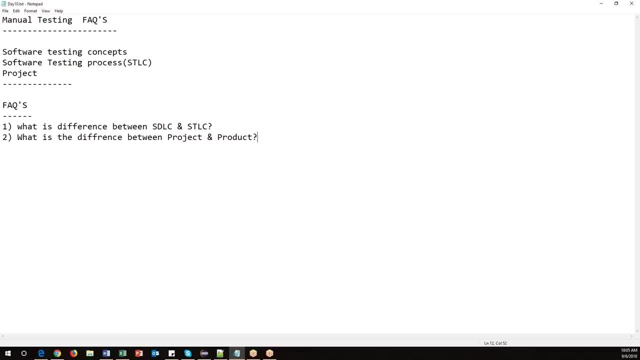 difference between project and product. So project is developed based upon customer requirement, specific to customer, whereas product is developed based upon the market requirement. So the first: we need to capture all the market requirements or user requirements, and then we'll prepare the product. So the company is also that two types of companies: service-based. 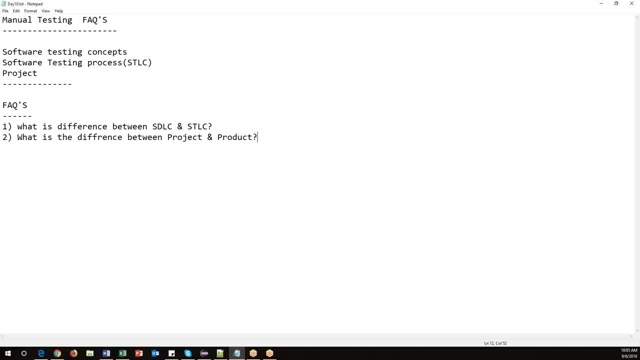 companies and product-based companies, and especially product-based companies like Microsoft, Google, IBM. So these are all developed, the products based upon the market requirements. and there is some other call, something called So project is nothing but the requirements we will capture from the specific customer and then we'll develop the software for that particular customer. That's called as a project, Project versus product. And then the next question is: what is vModel? 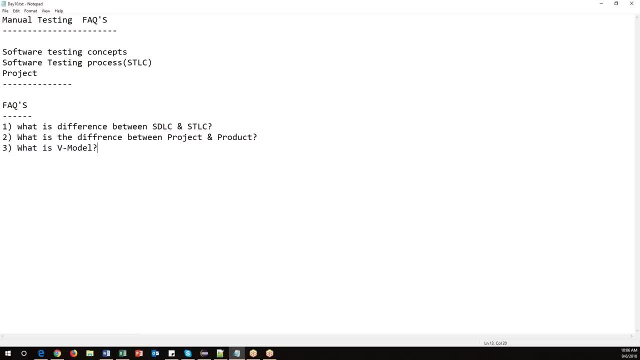 What is vModel? So in the previous sessions we discussed about software development lifecycle models. as part of this, waterfall model is one of the model And then, by overcoming the disadvantages, we have a vModel also. Before Agile came into the picture, the market was there in the vModel. 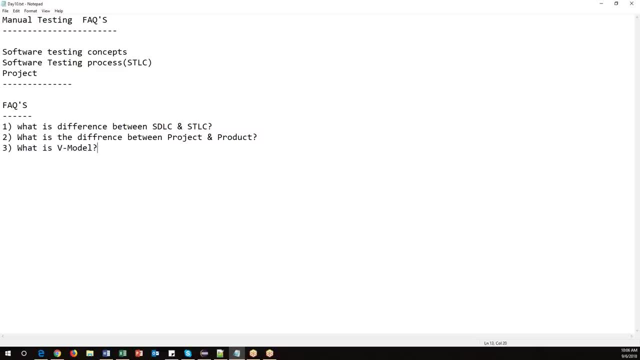 So what is vModel? In the vModel, development and testing activities will go parallel. So from the development perspective, they do Understanding the requirements, they will develop the code, they will do any testing, integration testing And before delivering the bill to QA, so the QA or testing people will prepare test plans and test cases and test environment setup. All these things will be connected. 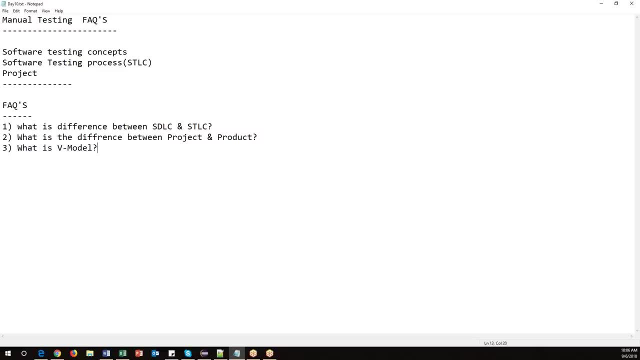 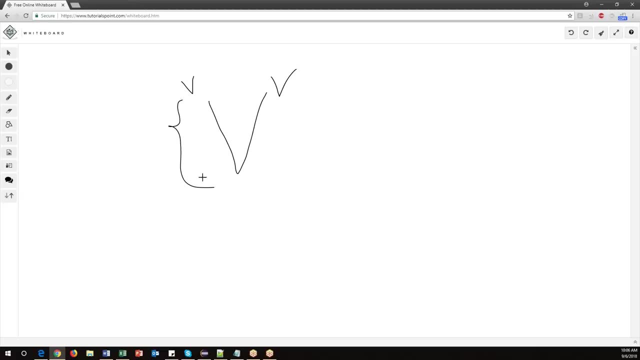 So these are two are part of the vModel. So one side we have verification part, the other side is a validation part. So in the vModel so verification and the validation, So in the verification side all the development activities will going on. 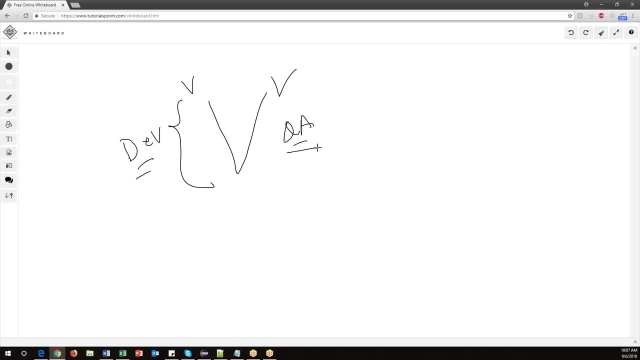 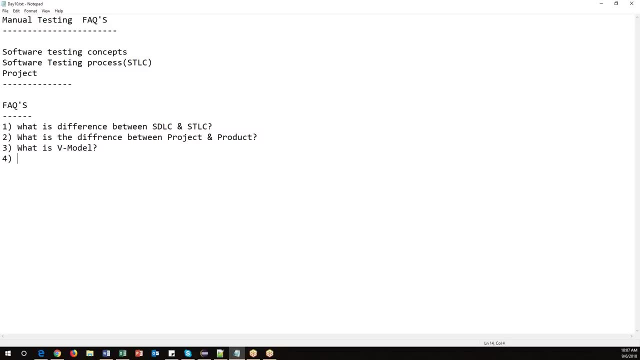 And the validation side, QA activities- will going on. Okay, this is a vModel And the next question is: what is the difference between QA and QC, Difference between QA and QC? So QA means quality assurance and QC means quality control. 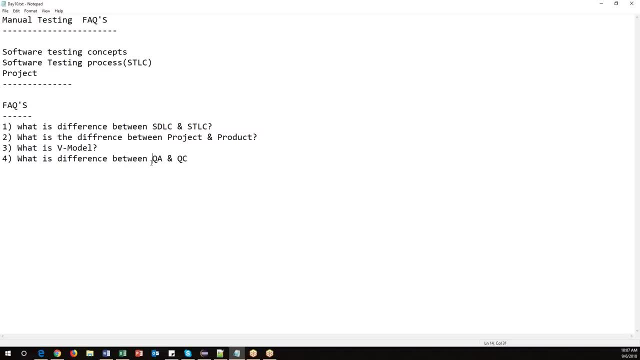 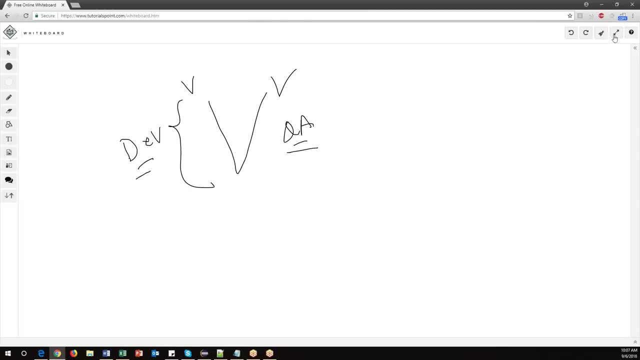 So quality assurance is basically talking about the complete process. So quality assurance is basically talking about the complete process process and QC is mainly focusing on the testing activity. okay, so in company there are two different things: QA and QC. so, for example, whenever developing a software, so suppose there is a development is happening. so development. 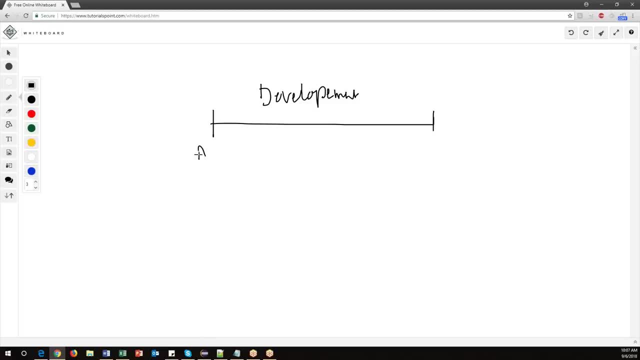 is happening and development will take certain phases, like analysis phase and design phase and coding phase and testing phase and then deployment phase. so here QC is nothing but quality control means. it will define the process, the complete process, what process we are going to follow, and this is taking care. 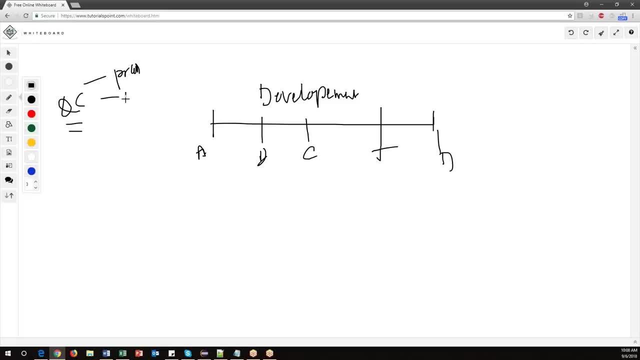 of all the activities or all the phases, and normally all the management people comes under the QC part and QA. USA QA. this is all about q, sorry. QM is quality assurance, so these people are responsible for assurance of the quality of the product and then at the кру, 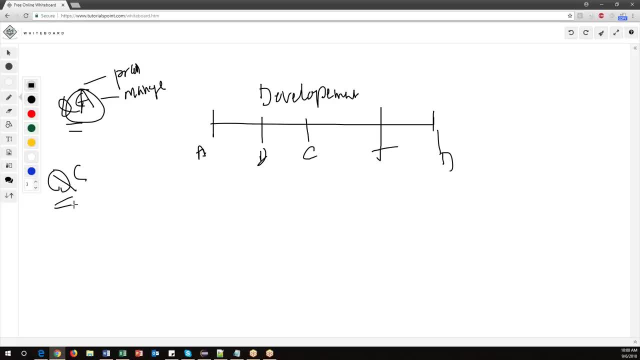 end. so there is another team called as a qct. so qc means quality control and all the testers will comes under the qc and they will take care of only the testing part. okay, product testing. so whether the product is meets the customer requirement or not, it is quality or not producing. 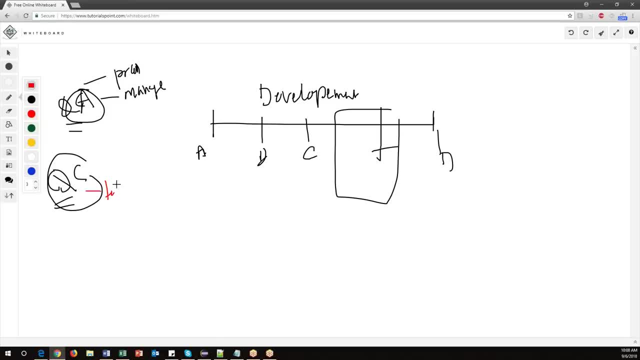 the proper quality or not and qc is for testers, so we test the product actually. but qc is a process related stuff and qas is for preventing of defects. prevention activity means we are need to make sure in future we should not get any issues. for that we need to define proper process. 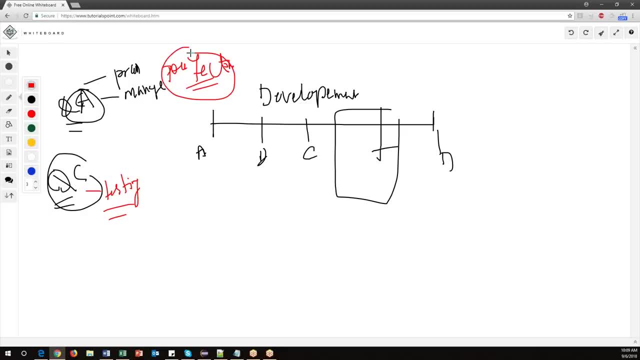 we need to go with strategy. so that is a different prevention process, whereas qc is the detection process. suppose there are some bugs or defects will be there in the application or software. we need to find out those bugs. that is called as a detection activity. so qa versus 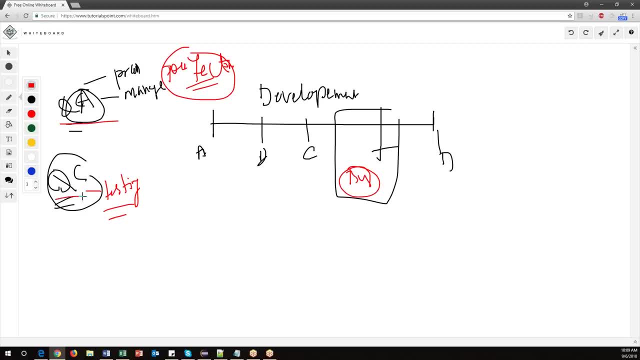 qc is a process related stuff and qa is for preventing of defects. prevention activity means qc, so qa is a process oriented, qc is testing and qa is for prevention of defects and qc is for actual testing of the defects and qa will take care of entire sdlc process, whereas qc's 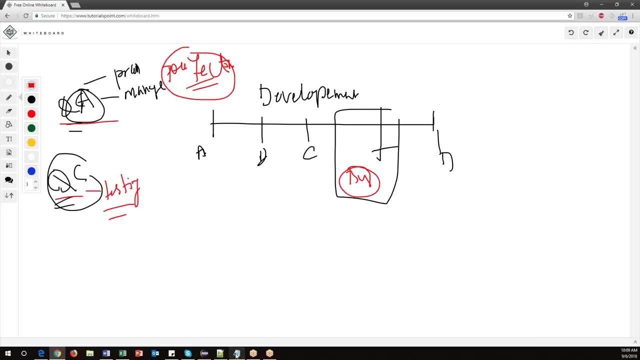 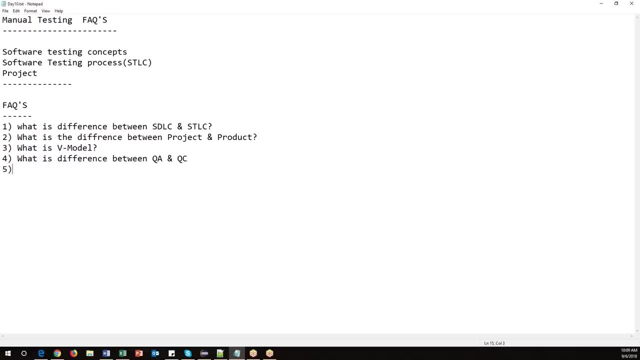 will take care about only testing process. okay, so that's the difference between qa and qc now. so the next question is: what is unit testing, what is unit testing and who will perform this testing? so what is unit testing? who will perform unit testing? so unit testing is nothing but. 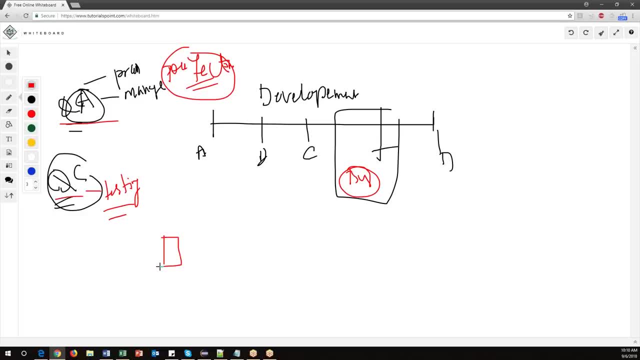 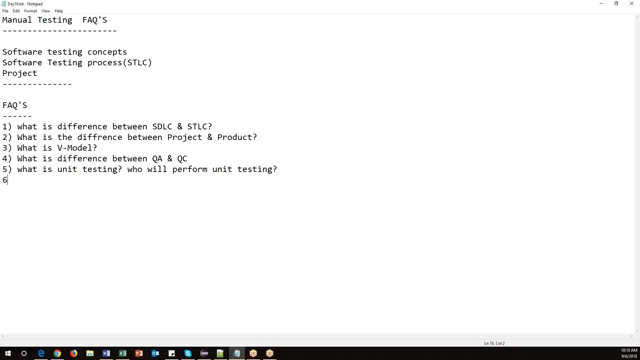 testing. a single program or single component is called as a unit testing. normally the unit testing is done by the programmer or a developer because they need to test internal logic of the program. right, that comes under the unit testing and similarly the other testing is called as a unit testing. 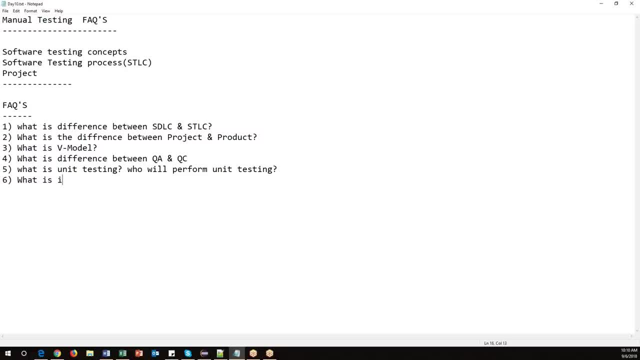 so it is here for our 2 modules. one configuration that is a unit testing. then in the other one we will have two 아나 하는 module system, so Portable module. you can search blonde or gray or red, for example. here we have a single module and we test already this particular module every. 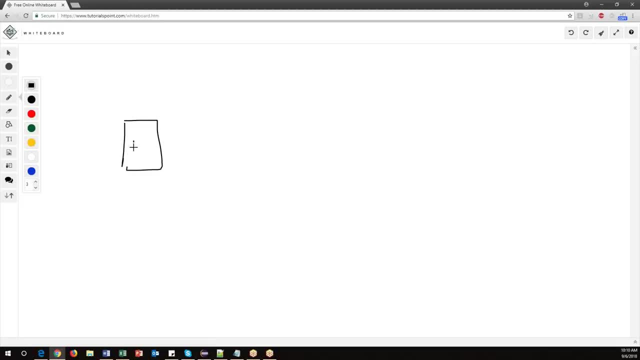 component. okay, so that we test only one module here and this is a module one, then the second partnering control module and so on, and we can determine, for example, if we want to test like one module, that it will go with a single module, that it is built possible in a single format. this part, 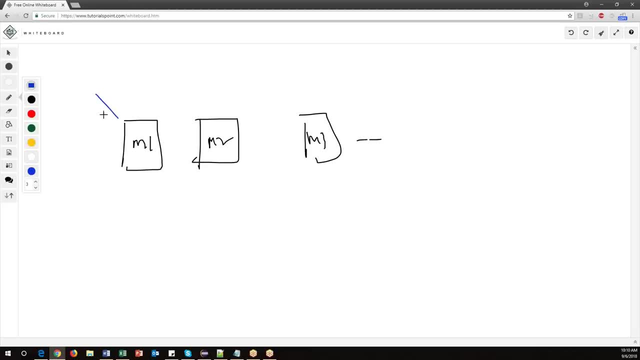 what is the Tuc Yonh row method? here we will run two modules and we will also perform on a single working module. that is what will perform this test: integration on an integration testing. so integration testing means: Hey, integration Master. integration testing means: if you want to test this module alone so we can just put some input, we can give some input and 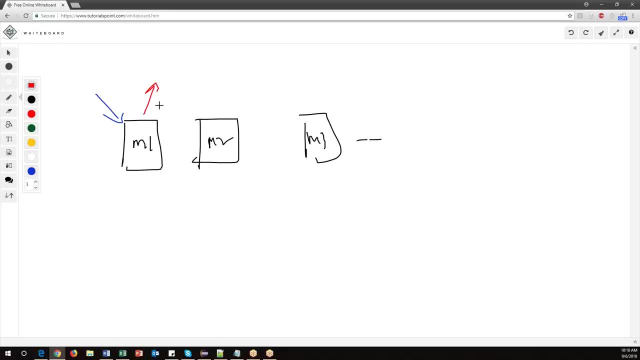 we'll get the some output from out of it, and sometimes the output of the one module becomes an input for the next module and the output of this module again input for the next module and finally we will get the final output. so if you test these components independently, that is called. 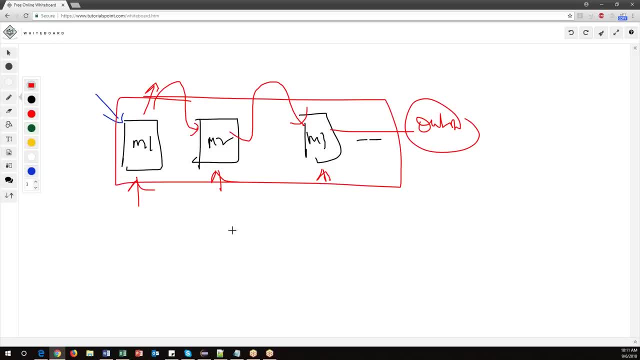 unit testing and if a combined, if a test called as integration testing. integration testing, so whether these modules are communicating properly or not, providing the expected results are not. so this is also internal testing. white box testing, okay, so, so white box testing technique. so internally the program will test the logic. so that is the integration testing developer will. 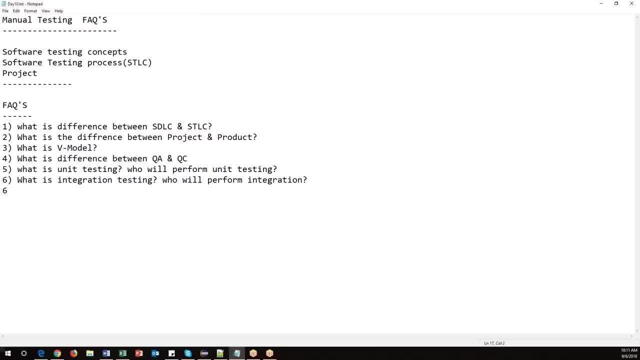 perform the testing? and next one is integration. what is integration testing? what is integration testing? what is sorry? system testing- what is system testing? and, uh, who will perform this testing? who will perform system testing? so system testing is a very important area where actual testers will be involved. so during this testing, testers will test the complete functionality of the application. 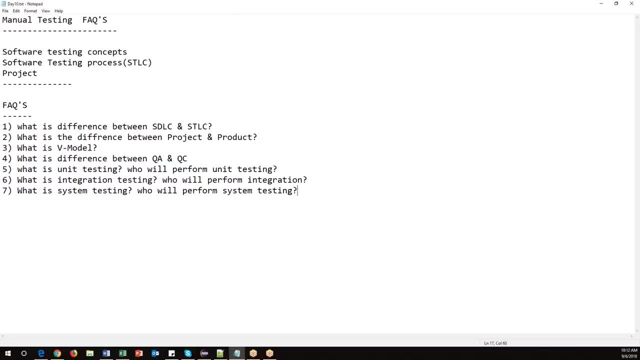 with respect to customer requirement and he will get to understand the requirements and use cases and prepare the test cases, including the test cases and reporting the defects. all these things comes under the system testing system is nothing but the complete software or complete application, so system testing is nothing. 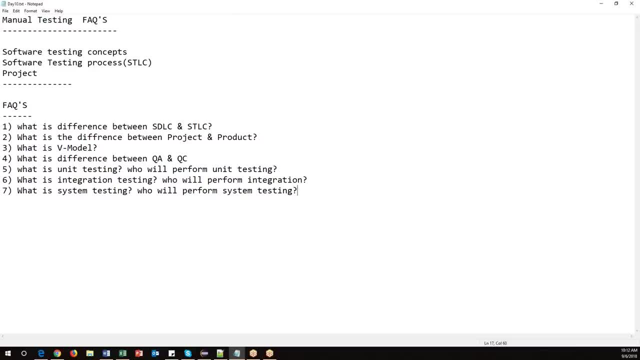 but testing the end-to-end functionality of the application with respect to customer requirement, and testers or qa team will perform the system testing. now very important. what are the uh So types of? What are the different types of system are testings? what are the different types of testing? so, if you want to practice, 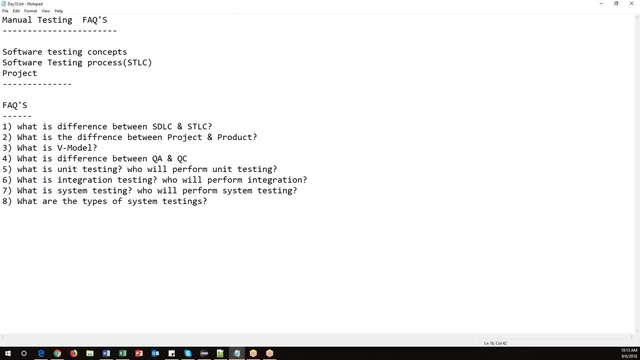 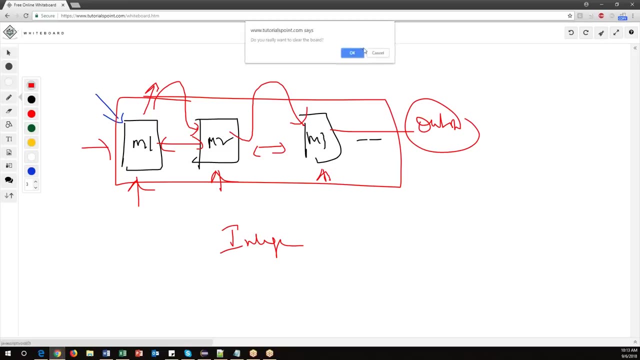 the actual이라는 anh, the cross-sectional knowledge and, if you want to practice, the successful testing. Apart from these improvements, in order to skip to the future, especially with the regulatory types- already there are other year- and the ten types of system testings, the testers will come back to work with the complete system or complete product testing will be divided into two categories. one isа functional prospective, the other one notamment. 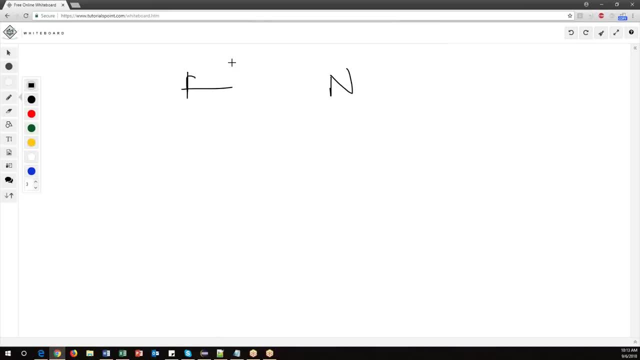 So one is functional and the other one is a lot in the functional side. the functional side, so both are comes under the system testing forms. so the functional side comes under the specific ones, so both come under. isあー similar, Sorry, Okay, you will test the application UI on the flows and navigations and database is. 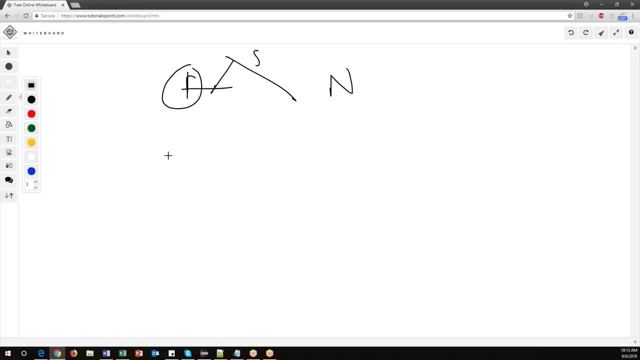 working or not, elements or displaying or not. So those things will mainly focusing on that's called functionality means the behavior of application is called as a functionality, and a non-functional testing means once the functionality is stable, and then we'll conduct the non-functional testing, like performance testing, security. 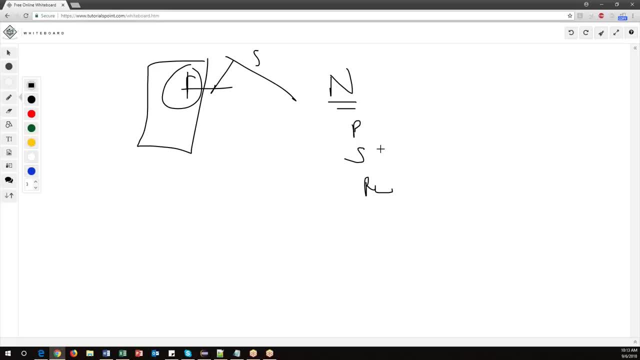 testing. Okay, and it's a reliability testing. all these things comes under the non-functional testing and this is also comes under the system testing. but these testings need a complex kind of environment and different skill set people, So these testings are not normally done by the functional testers. 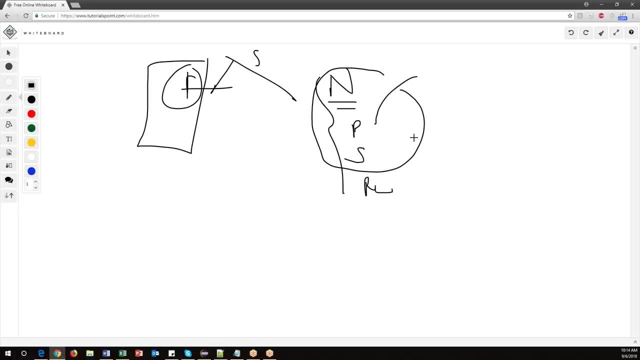 And if you want to do the performance testing, there will be different environment. a required and secure testing is a huge kind of testing. Okay, So these are the two different types of system testing: Functional and non-functional. again, in the non-functional testing we conduct input domain. 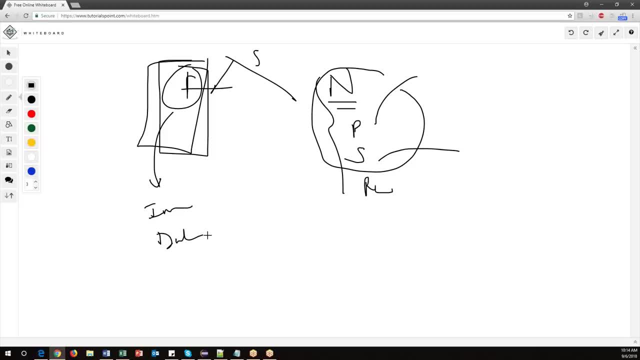 testing and then database testing, error handling testing. Okay, if it is a web-based application, we do the cookies testing, links testing. All these things will be part of functional testing. So we already discussed this in the entire session, So please go through that. 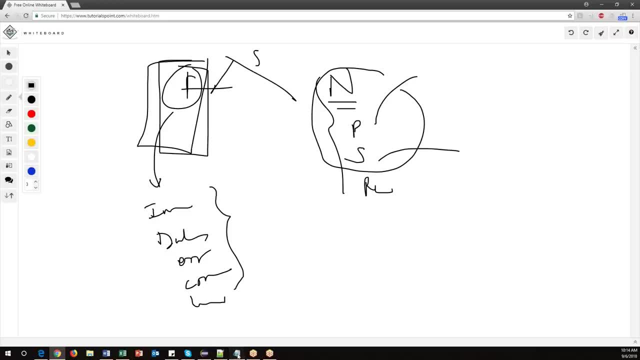 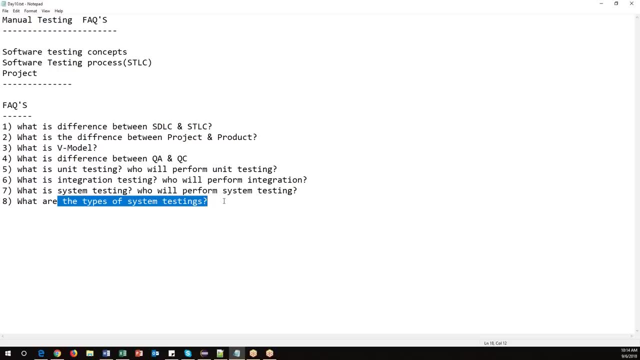 So functional testing and non-functional testing. So these type of testings we conduct as part of the system testing. So what are the types of system testing? Functional and non-functional? In the functional testing we do input domain testing, database testing, error handling testing. 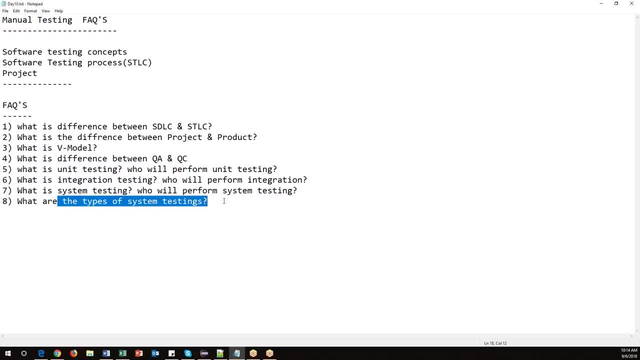 and so on. In the non-functional testing we perform performance testing, load testing, stress testing, security testing, recovery testing and so on. So these all comes under the non-functional aspect. The next question: What is difference between white box and black box testing techniques? 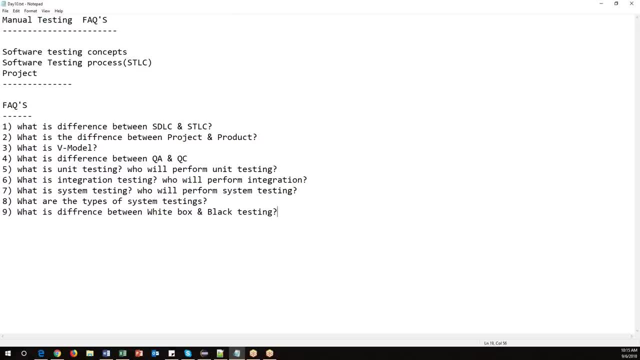 Okay, Okay. So what is the difference between white box and black box? So in the white box testing we test the internal logic of the program by developer or programmers, Whereas in black box testing we test the application functionality with respective customer requirement. We don't test the internal logic of the program. 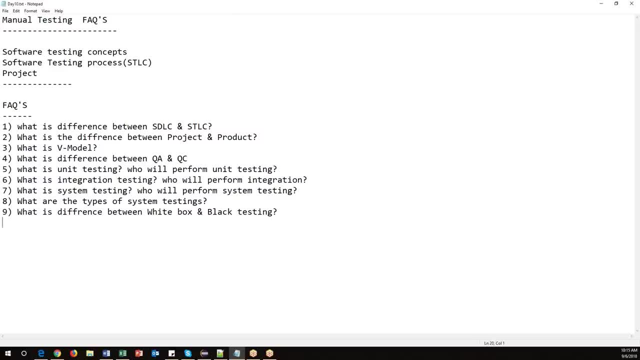 So that is the difference between white box testing and black box testing. and the next question is: What is verification and validation? What is the difference between verification and validation? Difference between verification and validation? So what is the difference between verification and validation? So verification is static testing technique. 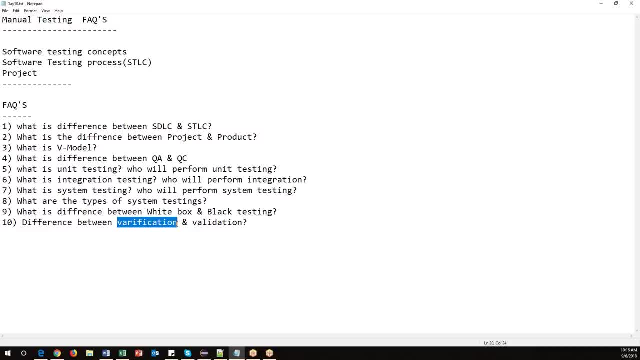 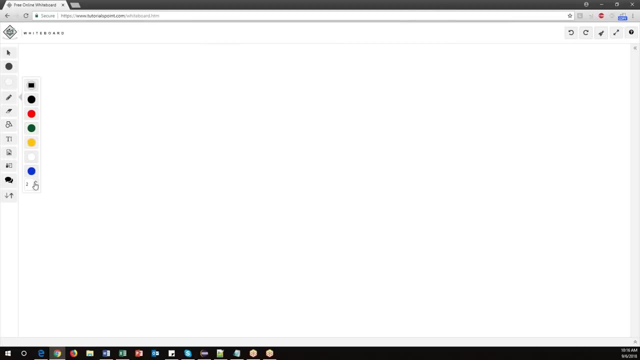 Okay, So we verify the documentation part. So, whether are we following the correct process or not? Okay, Whether the document is created properly or not, The correctness and completeness- There are two things- are very important in verification. So two things we need to focus on. 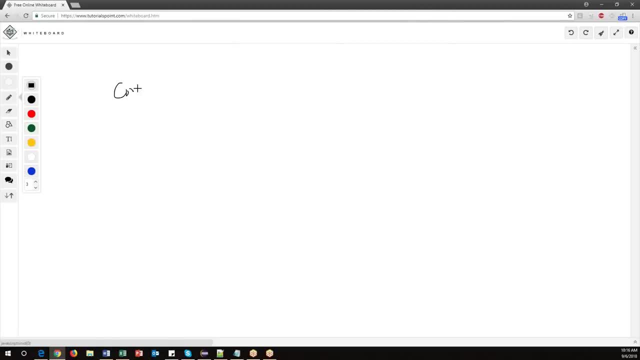 So one is correctness. Suppose somebody created some document, we need to review it. How we need to review, Why we need to review? We need to ensure the correctness of document and the data is correct and the completeness of document. if the data present in the document is completed or not, or some information is. 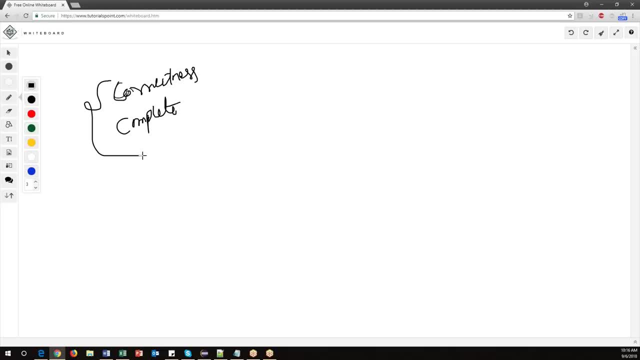 missing or not. So the correct to ensure the documents are complete or correct. So that's comes under the verification part. So verification in the sense verification means correctness and completeness of the document. to check the correctness and completeness of the document and this is also called as. 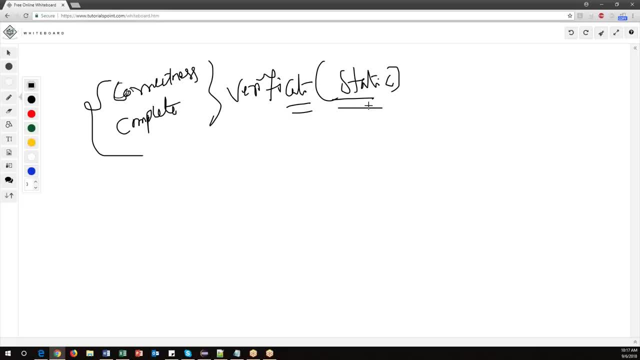 a static testing technique. So verification comes under the static testing, because we validate the documentation here, we verify the documentations here and when you come to the validation- so validation is a- comes under the testing part. So once the product or software is ready and then we'll perform the validation. 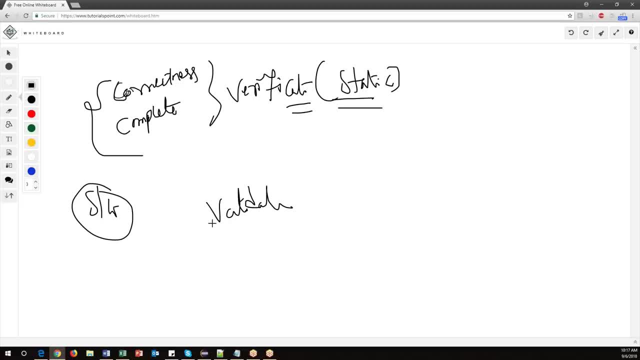 So whether the software is working according to customer requirement or not, that comes out of the validation part. So as part of this validation, we will contact the system testing okay, and you UAT testing and these things comes under the validation part. This is a dynamic testing technique. 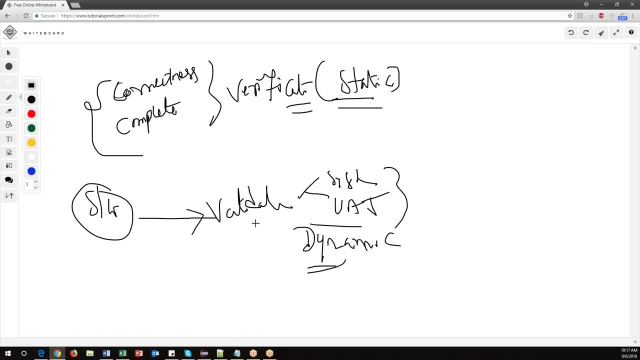 So validation comes under the dynamic testing, because we test the software. we test the software according to customer requirement. So this is the difference between verification and validation. So verification checks the documentation part before delivering the software or before software is developed. and after software is developed then we do the validation: whether the software 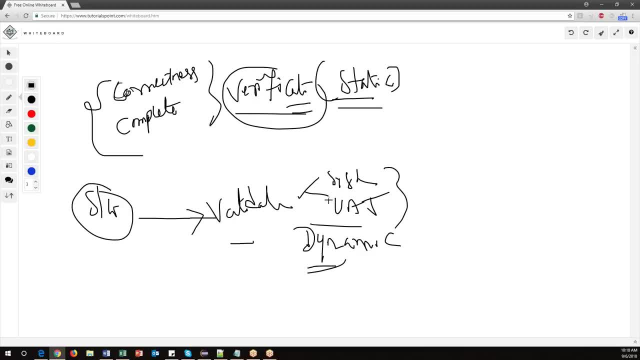 is working according to correct working, according to customer requirement, or not, Okay. So if you simply say here, Let us say this is a process, Okay, And in this point of view, the software is ready here, Okay, So to develop this software, what are all documents we've created, each and every phase. 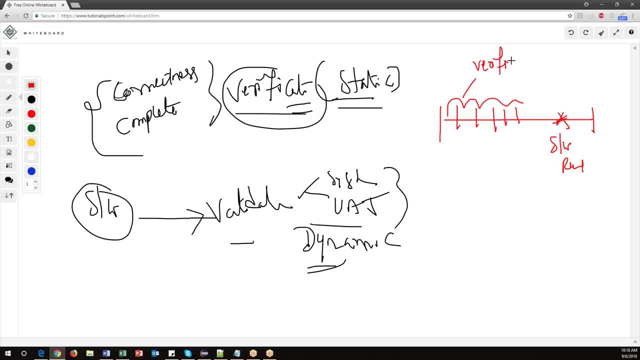 if I check those document that comes on the verification. So this verification comes here. So once the software is ready, we don't verify any documentation partner, So we will directly test this software. So here the validation part will come into picture. So verification done before software is development and the validation will done after software. 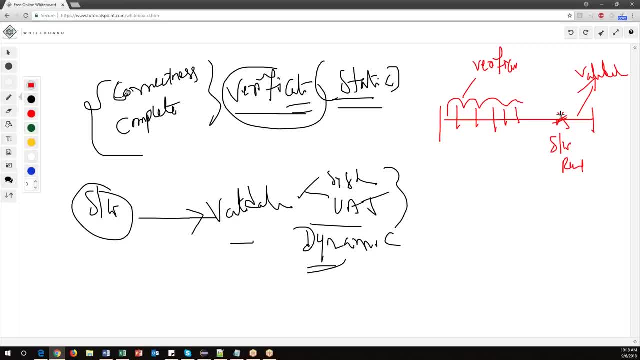 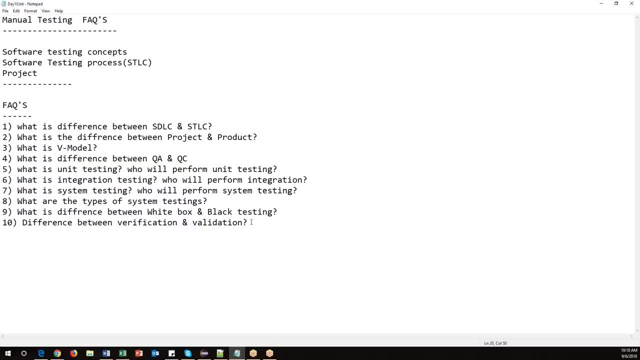 is completed, whether it is working according to customer requirement or not. So that is the difference between verification and validation. And next question is: what is GUI testing? what is GUI testing? So what are the different items or what are the different components you will test as 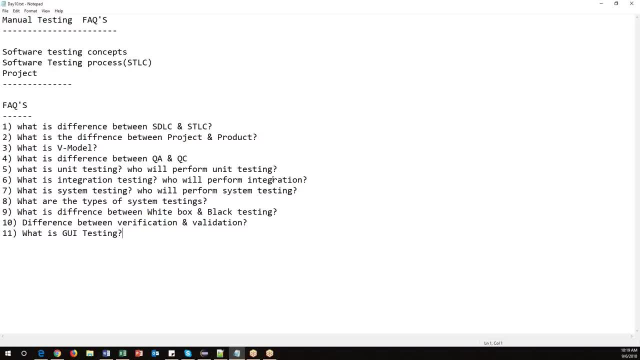 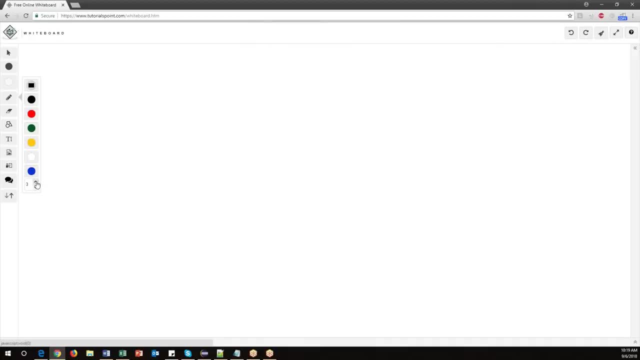 part of GUI testing. So GUI testing means graphical user interface testing. Graphical user interface means whatever the elements or text boxes, radio button, check boxes, images, links, these are, all comes under the graphical user interface. So graphical user interface testing means we need to test the behavior of these elements. 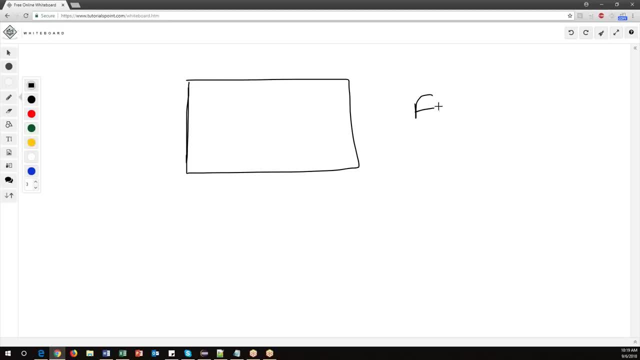 whether the font is correct or not. especially, we need to focus on few things like font is correct or not and spelling mistakes are there or not. and then alignment of the element. alignment should be properly and then font size, font color and size, both So font color and size, and spellings of the labels and text and alignment of the element. 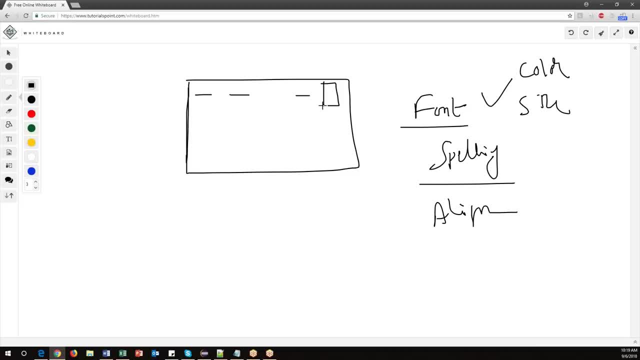 some, all the links properly aligned or not, all the images are properly displayed or not. So especially, the main focus of GUI testing is look and feel of the application, So how the application will look and feel of the customer point of view or user point. 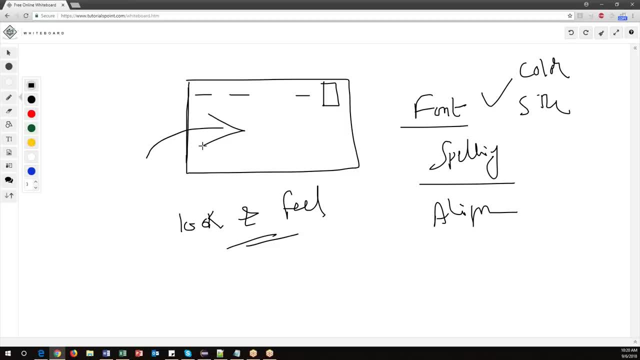 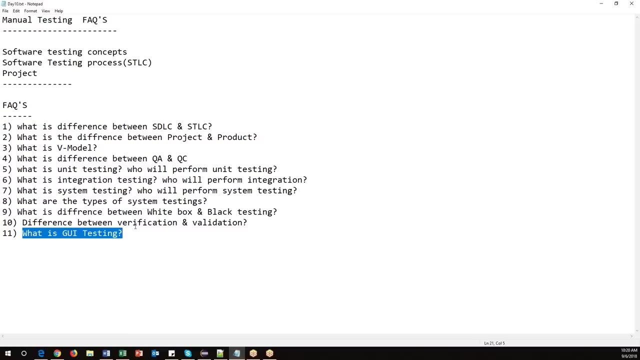 of view That how much the application is attractive, Attraction, Attractive the user. So there we need to more focusing on GUI testing, graphical user interface testing, So testing the application UI is called as a graphical user interface testing. Now the next question is: what is input domain testing? input domain testing and what are? 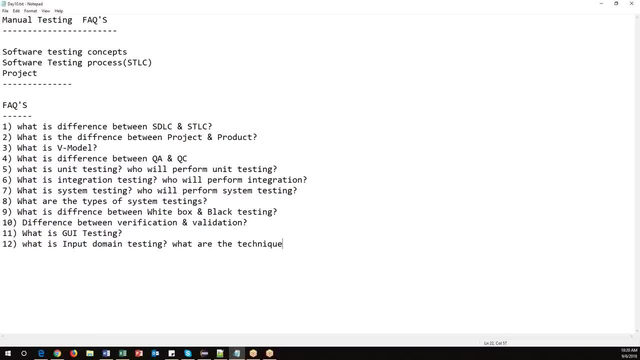 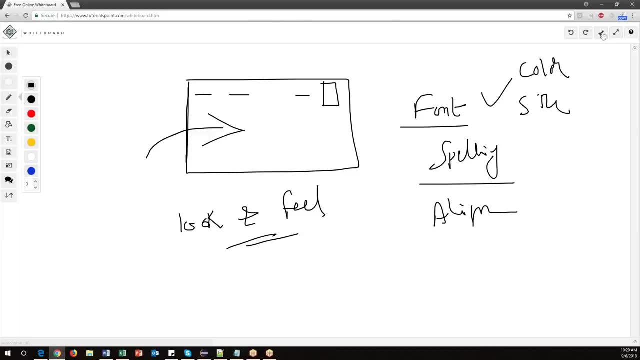 the techniques you have used. Techniques will be used in input domain testing. So what is input domain testing? What are the different techniques will be used in input domain testing. So input domain testing means so, for example, if you have a text box, something like this: 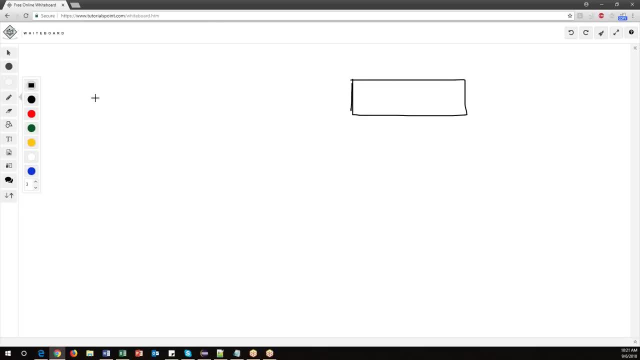 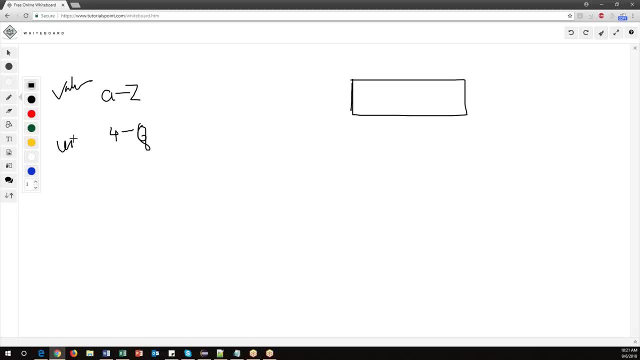 Okay, so this is a value prospective and this is called length prospecting. So, based upon this requirement, I need to test this text box, which is allowing the small letters are not, and it is allowing 4 to 8 characters are not, So this is called as input domain testing. 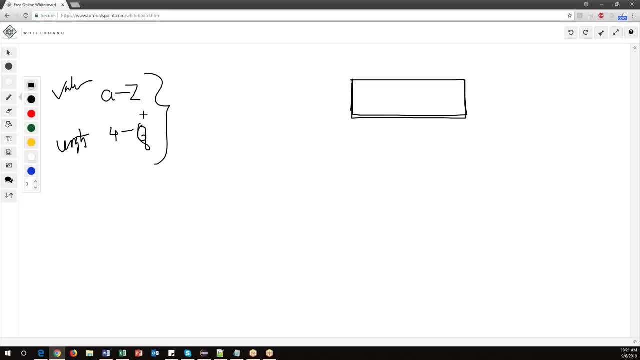 Input domain testing. Verifying the input boxes with respect to the requirements is called as input domain testing, And here we use two techniques. One is the equivalence class partitioning, The other is the variable process. The other one is boundary value analysis. 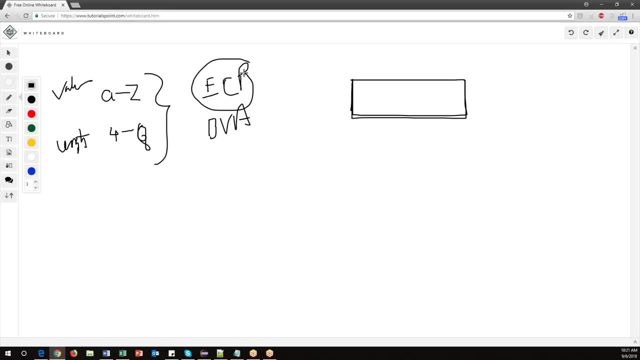 So equivalence class partitioning means we need to verify whether what is valid data, what is invalid data. So if you want to test this, what is a valid data here, A to Z is a valid data. Let's say we need to prepare small table like this: 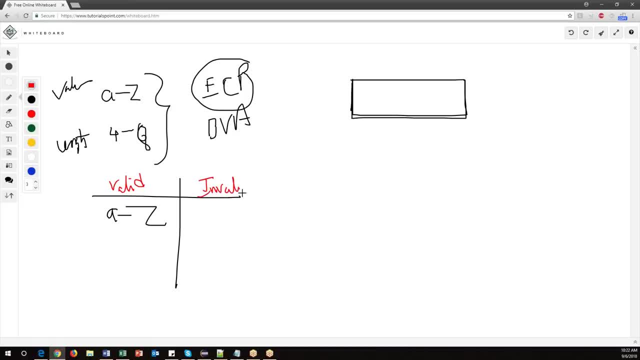 This is a valid and this is a invalid I. so only A to Z is a valid data and uppercase letters invalid. 0 to 9 invalid. special symbols invalid and spaces also invalid. So we need to prepare small table like this and based on this, we need to test this one. 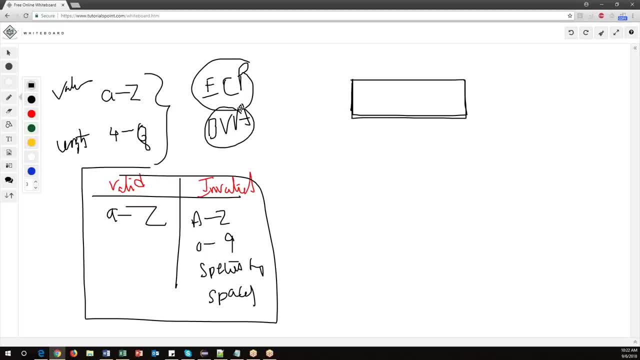 So that is called input domain testing and there is another technique called as a boundary value analysis. It will basically talk about the range, So how much range we can give these values here. So let's say 4 to 8. we are saying 4 is a minimum, 8 is a maximum. 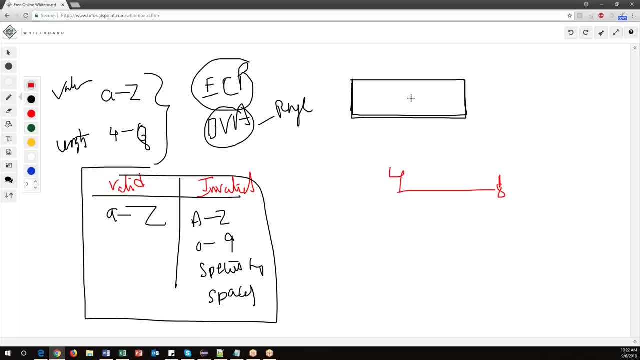 So we need to test the boundaries, like if I say four characters is working or not, So it should work. If I say 8 character it is working or not, It should. also should work. and 4 plus 5 should working or not. 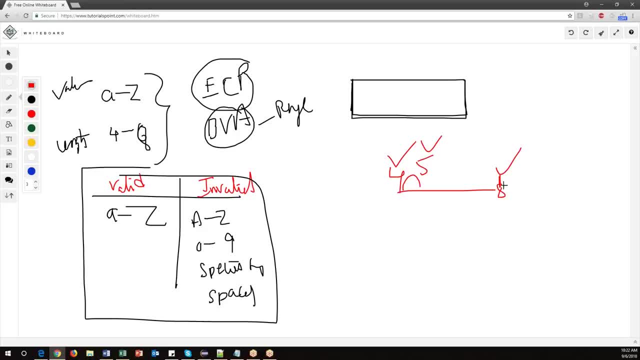 So 4 plus 5 should work. So 5 is also should work and 8 minus minus 1, 7 should also should work. and if 5 and 7 works, between all the numbers will work obviously. So if I say 4 minus 1, if I test this, 3 minimum minus 1, 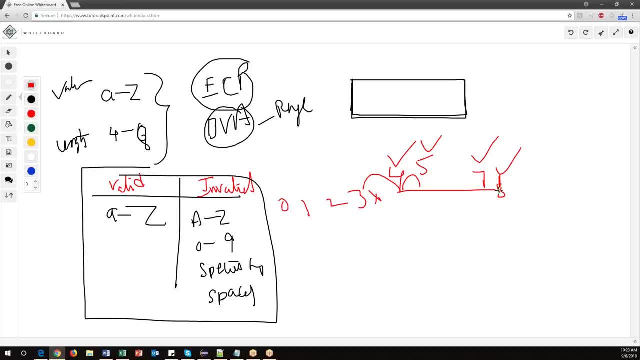 if it is failed, obviously 2, 1, 0, everything will fail. and if 9, we verify. so if 9 is failed, after that 10, 11, everything will be, everything will be failed. So, instead of testing with all the numbers, all the ranges, 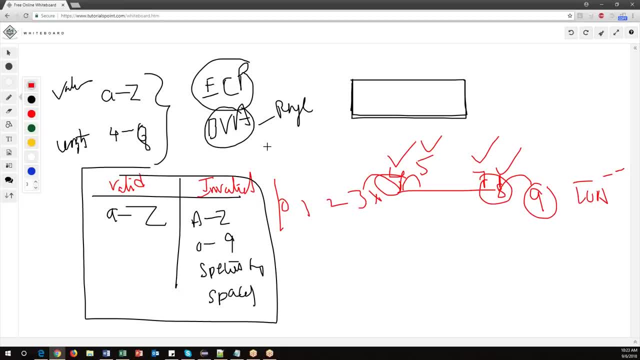 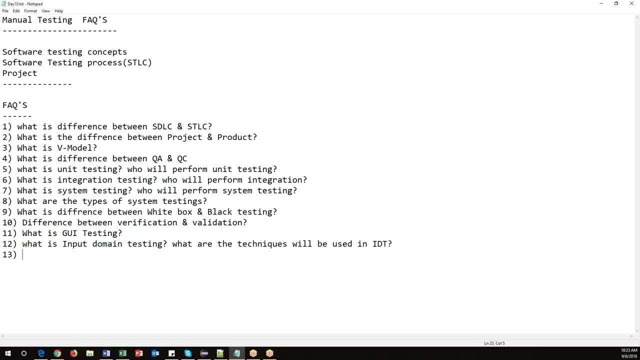 we can just only test the boundaries. that's called as a boundary value analysis, ECP, and boundary value analysis or input domain testing techniques. Okay, the next question is: What is database testing? What is database Database testing? So database testing means testing the DML operations with respect to the database. 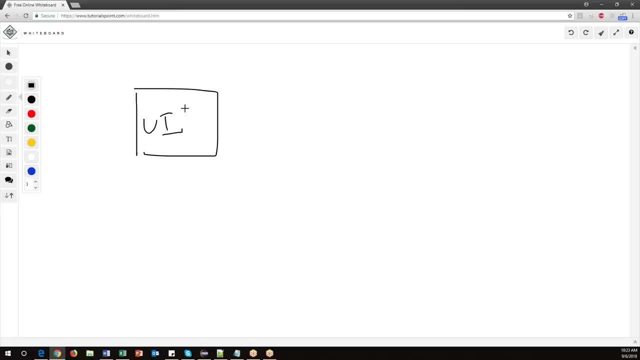 So you will have a UI part here. This is your user interface and let's say you are submitting some data here and your click, once you click on the submit way, that is, data is exactly present in the database back and database in the form of tables. 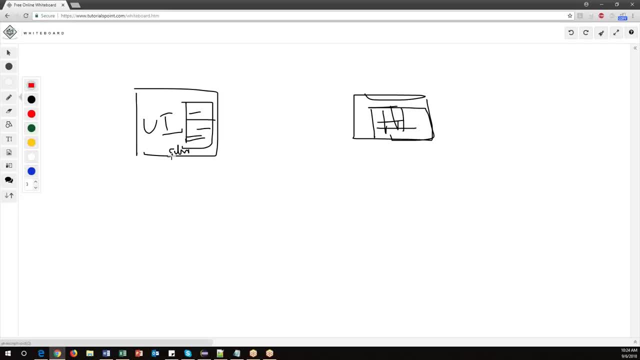 Now we need to test this scenario. So sometimes when you submit the data maybe the network is not fully connected, So maybe the database is down and because of some reason you data will not be affected in the database. So sometimes you will get acknowledgement properly. 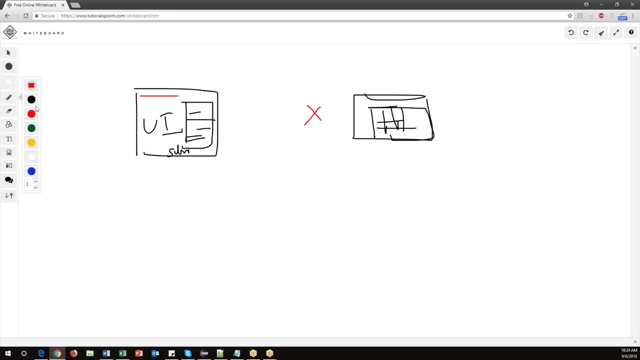 but the data is not getting updated in the table. So here we need to test the database testing. You have to perform transaction from the front-end application. whether this is affecting the database table or not, We need to verify. So this is called database testing. 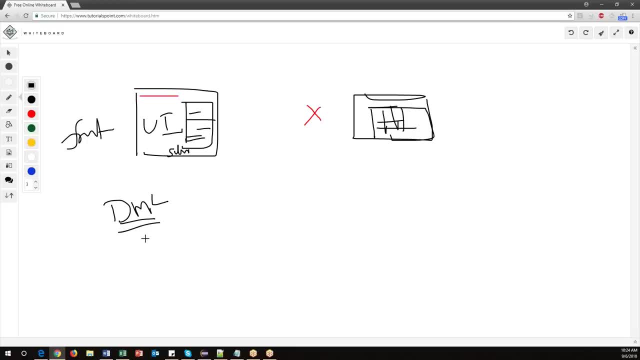 So testing the data manipulation language means here We will have a few commands called insert, Setting the data and updating the data and deleting the data, selecting the data. These are all comes under the DML operations and user is normally perform these operations. So when you perform DML operations from the front-end application, 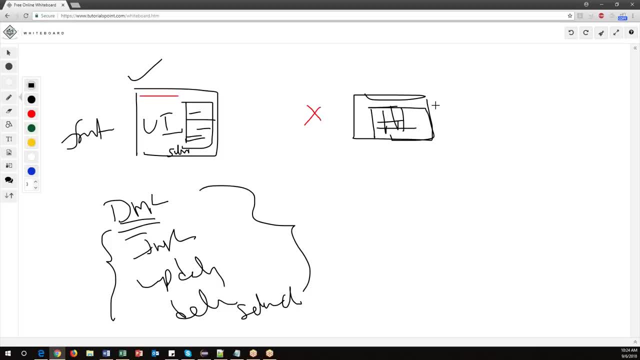 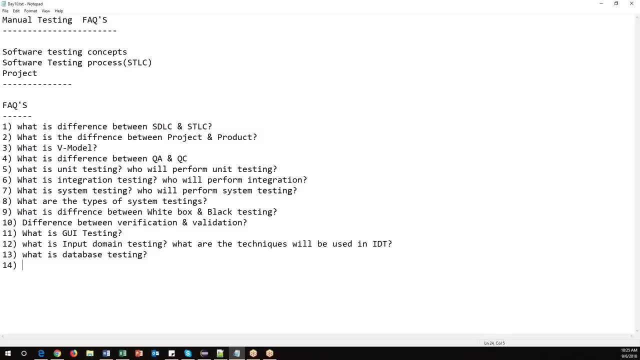 we need to verify whether they are affecting the tables or not. So that is all about database testing. Now the next one is: What is load and stress testing? So what is the difference between load and stress test? What is difference between load and stress testing? 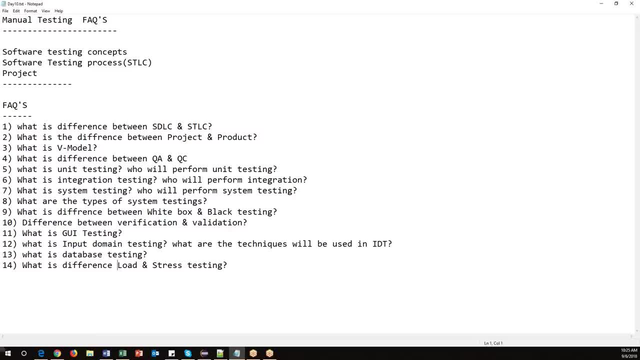 So in the load testing will gradually increase the size and then test the service, then test the speed of the application. So both are related to speed or comes under performance testing. in the load testing will space, will check the speed of the application while gradually increasing the speed. 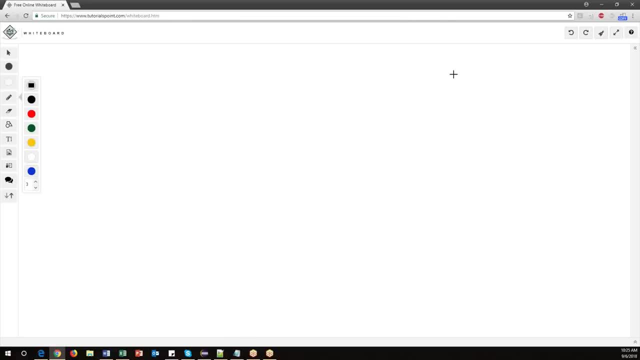 Let me just give you the scenario. So in the load testing, suppose the customer says hundred people are accessing the application, right? So here what we will do is the load testing. We will gradually increase the size. the first will access application with 10 people and then suddenly increase to the 20 people. 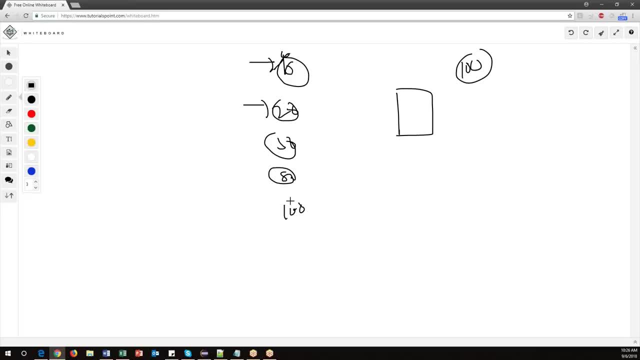 and then 50 people, Then 80 people, then finally hundred people and in all the cases the application is stable or not and the application is responding in the proper speed or not. So that comes under the load testing. So increasing the load gradually on the system. 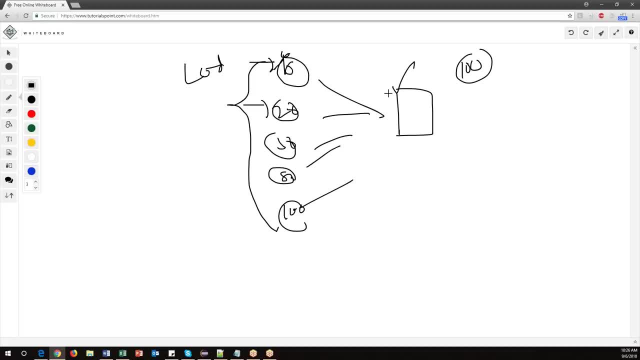 and test, verify the functionality or verify the speed of the application. But in case of trust, stress testing, what we will do is, let's say, customer saying, hundred users. So first we will access with the 10 users, immediately increase 20 users, again directly increase to the 90 users, like this: 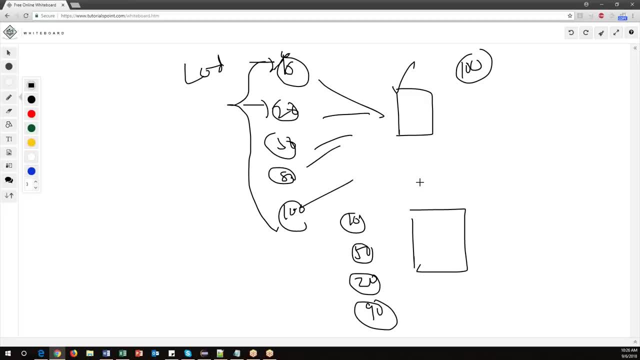 So sometimes we need to make huge, huge request and sometimes immediately will reduce the request again. make it huge request and reduce the request. So in all the cases, in all the cases, our application should be stable. Okay, you should not broken anymore. So this is called as a stress testing. 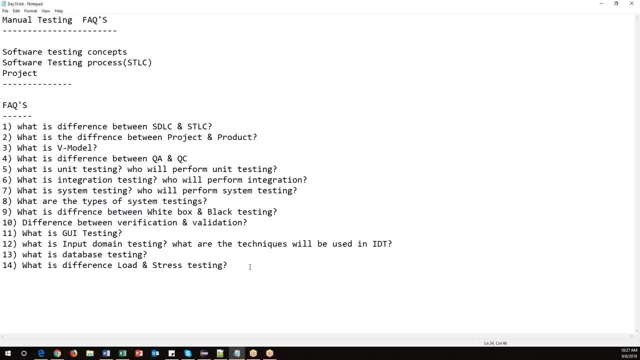 Okay, so load testing and stress testing- And these two are performance testing techniques. and the next important question is related to the test design techniques. Okay, so what are our water tested design techniques used while creating test cases? So what are the test design- water test design techniques used while creating? 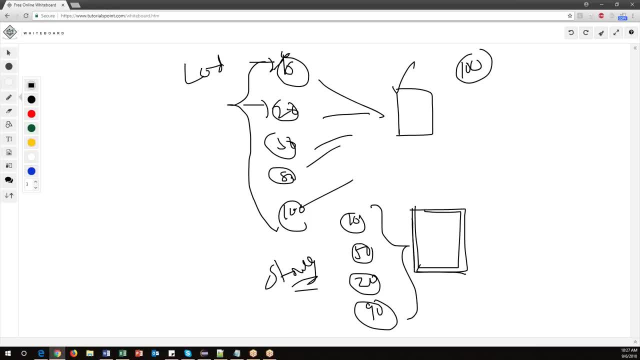 The test cases. So we already discussed a few techniques. So what are those techniques we have? So we have boundary value analysis technique, We have equivalence class partitioning technique. We have a decision table technique. using decision table technique, We have transition diagram. 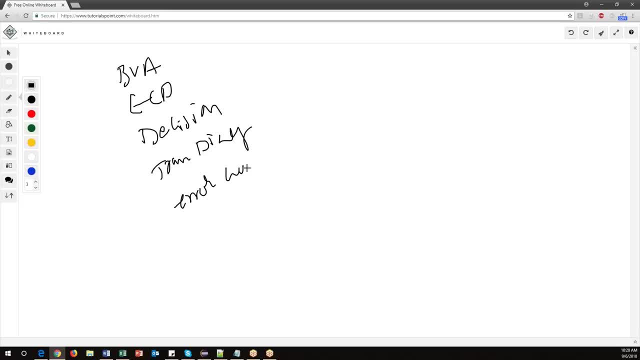 This is also one of the technique we have error-guessing technique, error-guessing technique. So these are all comes under the techniques to use To perform by testing. So tested design techniques: BVA, ECP design decision decision table- state transition diagram. 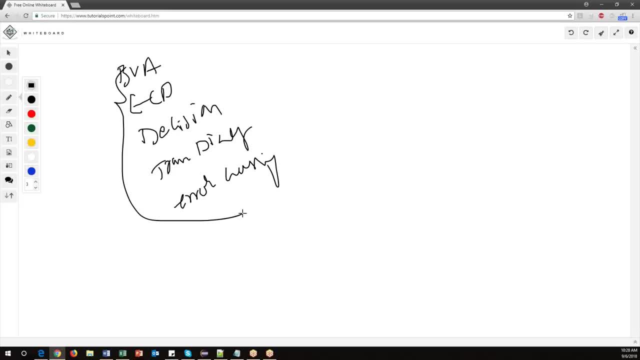 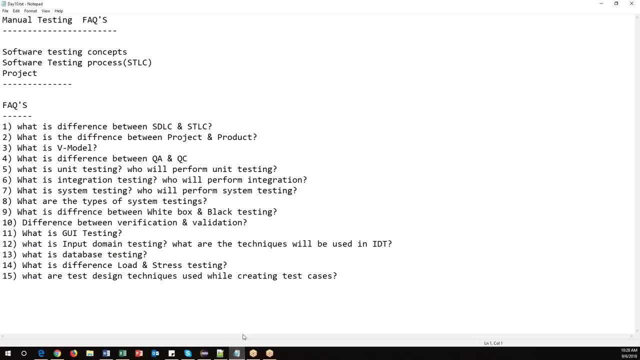 and error-guessing. So by using these techniques, we can prepare the test data at the time of creator creation of test cases. Okay, so we have to tell this. now They are. they are the tested design techniques used to while creating the test cases. 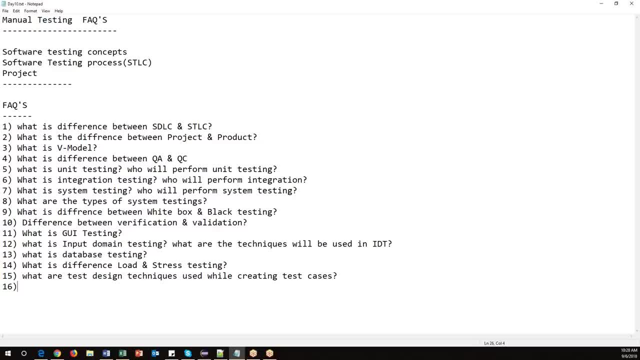 Now next question: So what is again? You will get the all the question like: what is decision table, What is state transition diagram? So can you give me some examples like this? So just remember this, Okay. you will get question like this: 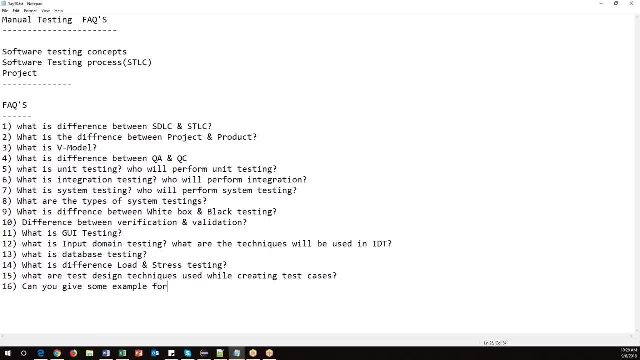 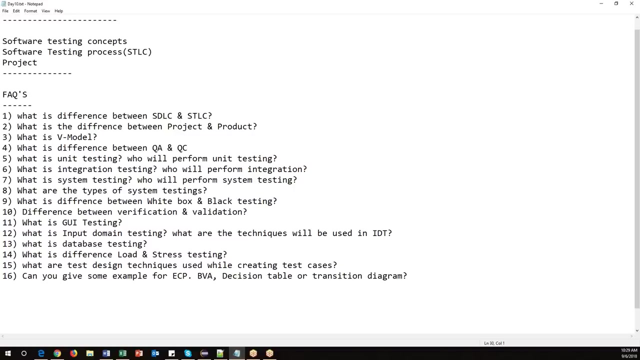 Can you give some example For ECP or BVA, or okay, BVA or decision table For transition diagram, Okay, so these are the techniques. people will ask you some kind of exam. So in the previous sessions I have explained very clearly with some use cases and some examples. 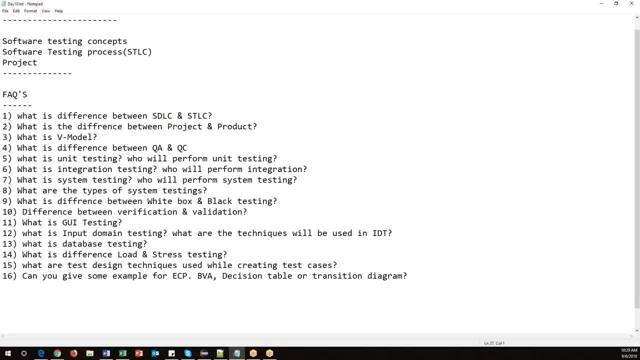 So just you need to remember those examples, at least one example. If you remember, you can easily explain this. so: equivalence, class partitioning, boundary value analysis, and then decision table and state realization diagram for each and every technique. you should remember one example, Okay, because immediately somebody will ask you. 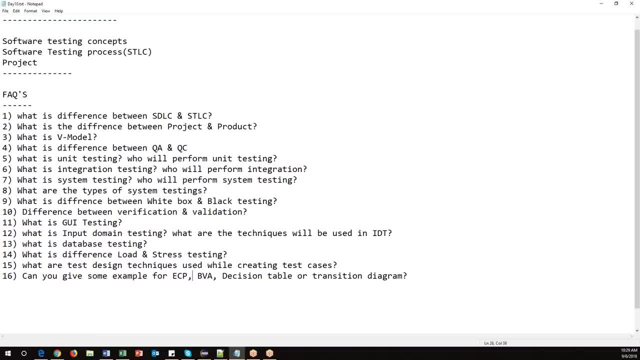 So can you give, can you try, a decision table? that means you have to take one scenario and you have to draw the decision table. and, similarly, somebody give you one scenario and ask you to create the transition diagram, You should able to create the transition diagram. 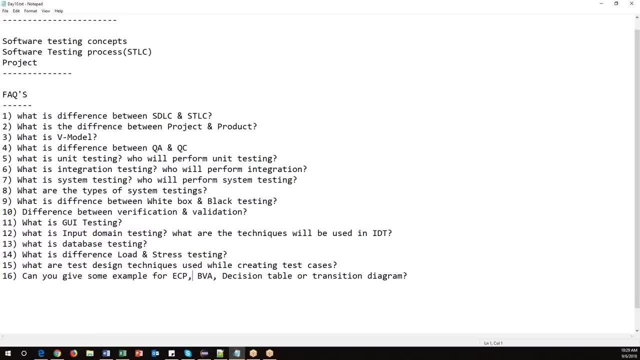 So please watch my recording, previous recordings and I have already explained this and very important question. And the next question is regarding the terminologies like: what is ad-hoc testing, what is ad-hoc testing and when to perform. when to perform ad-hoc testing. when to perform ad-hoc testing. 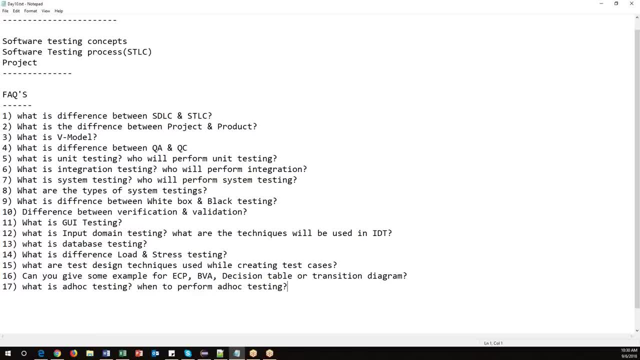 So ad-hoc testing means randomly test that application by knowing the functionality. You already know some functionality, Okay, so you already know the functionality, but you don't have any proper documentation. You are testing our application randomly, So that's comes under the ad-hoc testing and when to perform ad-hoc testing, suppose. 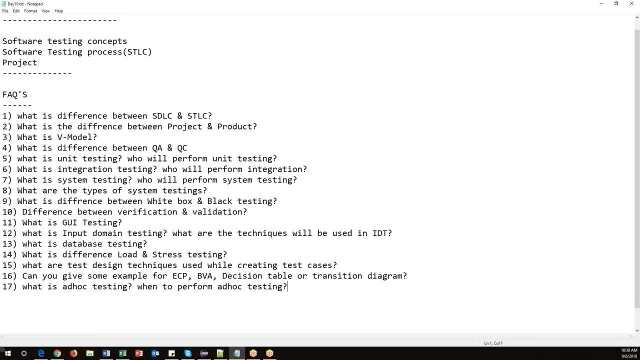 if you have some time. still you have almost completed all the testing, but still you have some time to do, and that time so you can just do ad-hoc testing to find out the corner scenarios or corner defects in your application. Okay, So in other way they can ask you question in different way. 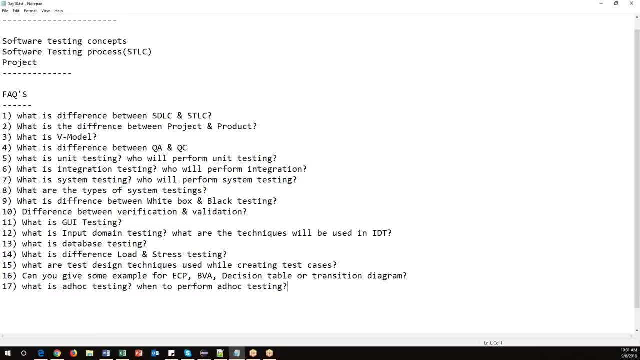 So they don't tell the name directly, like what is ad-hoc testing? They don't ask like this. They will ask you in different way, Like, for example, if you don't know the functionality, if you know the functionality but you don't have, okay, any documentation. 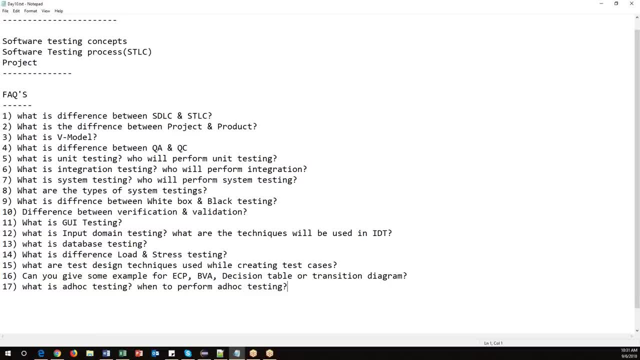 and you have some skills sometimes. So what kind of testing you will do, So what you will do. so in that case, you need to perform ad-hoc testing, Okay, and you will get one more question like this: So, for example, I have to complete my test in 15 days. 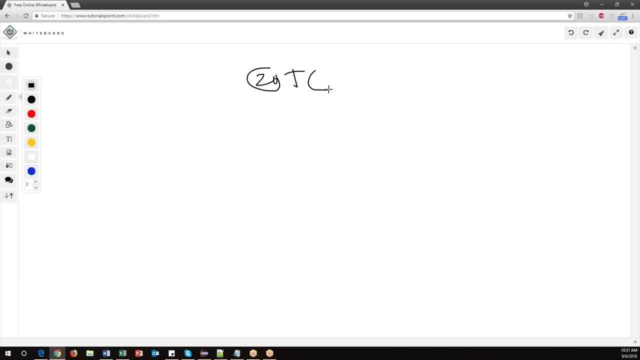 Let us say I have a 20 test cases overall in the 20 test cases. I have to complete them within 10 days. So 10 days I have to complete all the 20 test cases. So I have reached till 9th day. 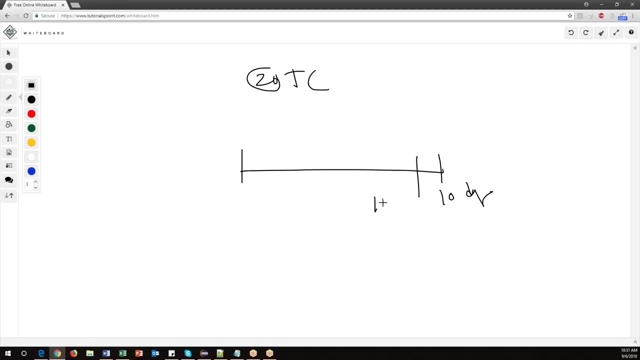 So in the 9th day- okay, I most almost- I completed 15 test cases. Let's say these are all complex test cases. Let's say a big number. Let's say hundred numbers, hundred test cases. So within the 10 days I have to complete hundred test cases. 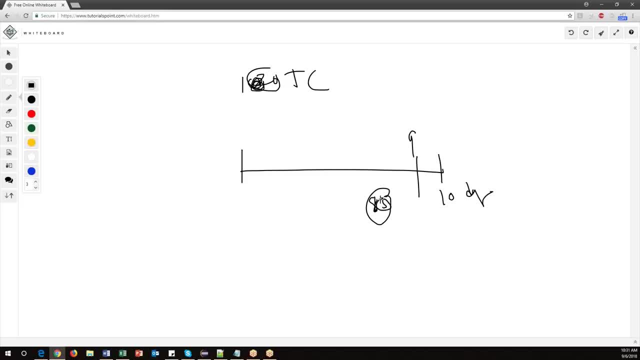 So the day of 9, almost I have done 80 test cases. still, 20 test cases still not completed, and within one day it is not possible to complete all 20 test cases. So what you should do now? So in this cases, you know all the 20 test cases, whichever functionality we have. 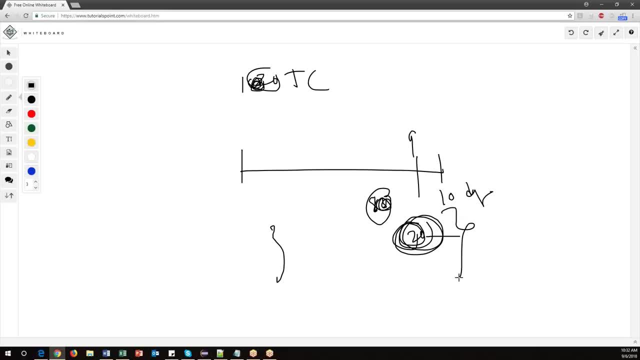 So we, on that particular functionality, instead of executing these 20 test cases, we will perform the ad-hoc testing here, because whatever time you have, this time is not enough to complete all 20 test cases. So if you do the ad-hoc testing, it will cover almost all the scenarios. 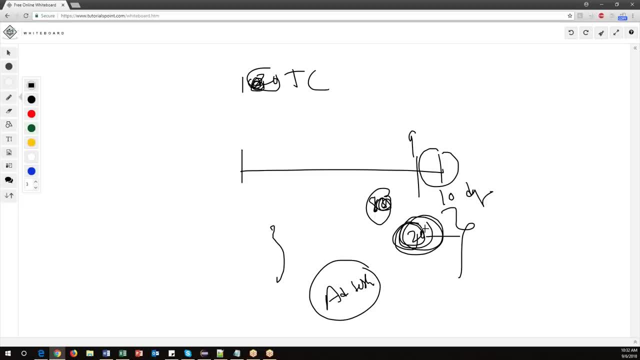 which are described in 20 test cases, So that we need to have before knowledge. Okay, all the 20 test cases. What are the different areas are covered in the 20 test cases and in ad-hoc testing. we will cover all those 20 areas, or 20 test cases mostly. 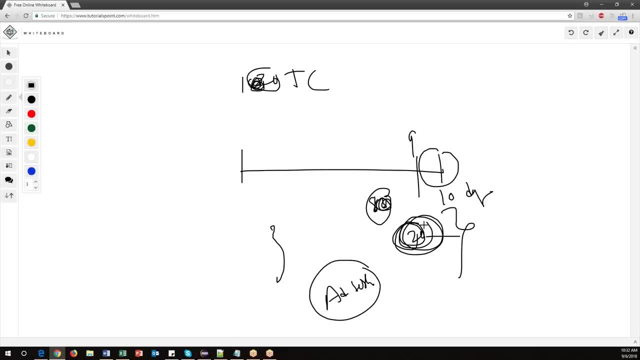 but not in detail, but at least very high level. we can verify it whether they are working fine or not. Okay, but that is comes under the ad-hoc testing. So these are the different ways. people will ask you the same question in different ways. 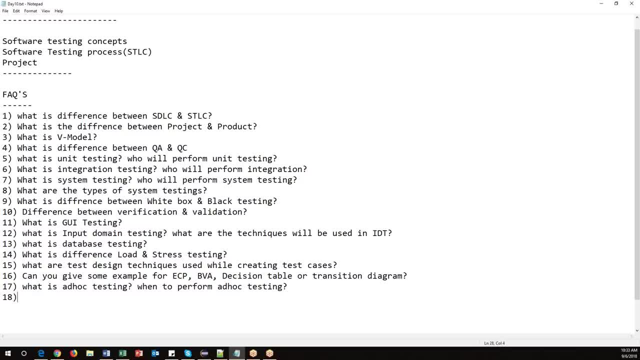 And what is ad-hoc testing, when to perform ad-hoc testing. and then the next question is: what is exploratory testing? When we need to perform exploratory test. So what is exploratory testing and when to perform exploratory testing? So these questions are almost similar. 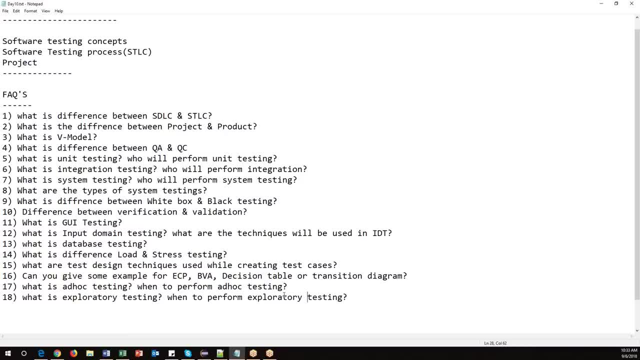 but a small difference we have. so exploratory testing means so we don't need or we don't have knowledge and application, but we are exploring the skills on the application. We're exploring the knowledge and application by working on with application. So we'll just randomly go through all the screens. 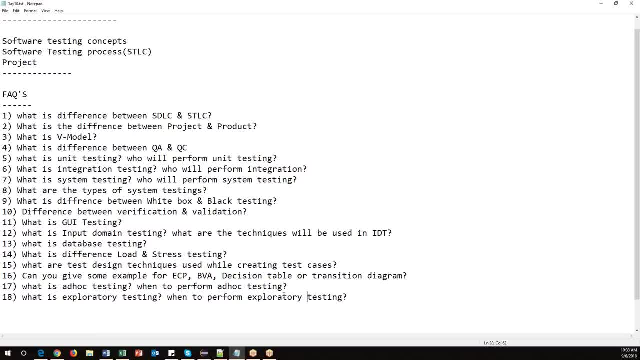 And all the links and all the functionalities and get to know the functionality that's called exploratory testing and when we need to perform this exploratory testing. we don't have any documentation, for example, and we don't have any test cases and build is ready. 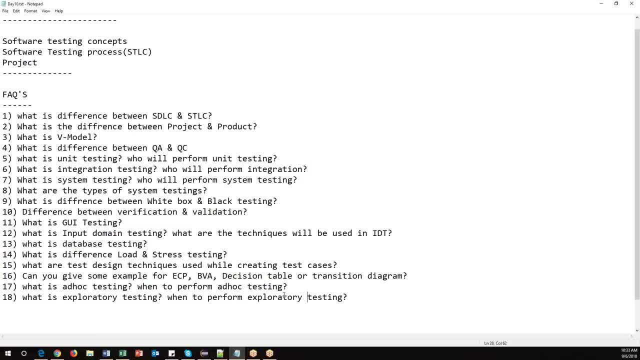 But at the time we don't have any test cases are written and those cases we can do the exploratory testing to explore the function, especially for the new joiners. So they do exploratory testing for a few days to understand the product completely. 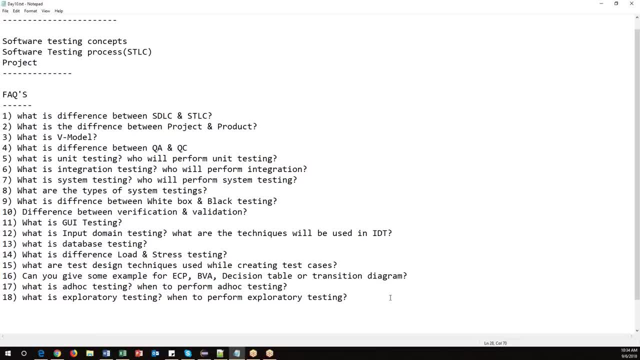 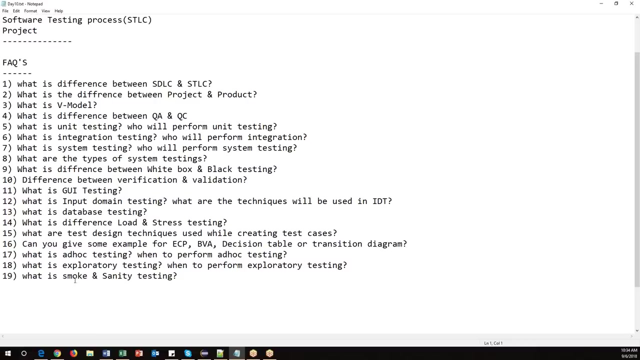 Okay, So that's all about exploratory testing, and the one more question is: what is, what is difference between our what is smoke and sanity testing? What is more kind of sanity testing? So this is also one more question people will ask: What is the difference between smoke and sanity testing? 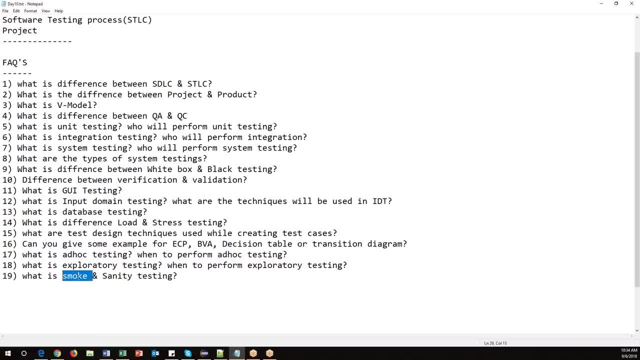 So smoke is at the initial level of testing. Okay, So in the smoke testing mainly focusing on the installation path, So build is properly installed or not, or somewhere it is broken or not. So that's called a smoke testing. And once the build is installed properly, 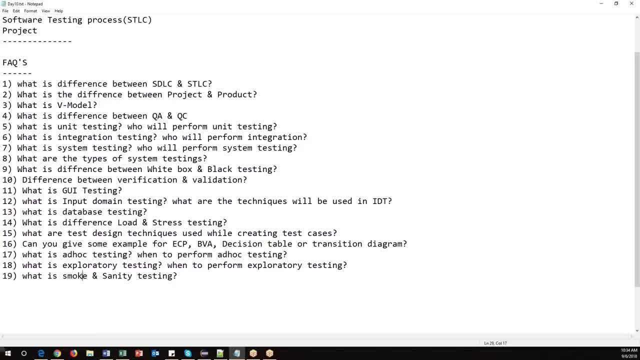 and a very basic scenarios we will validate, like login is working or not, like on the UI page all the elements are properly displayed or not and pages navigation from one page to another page is properly going or not. So very basic test cases We will execute there. that comes under the sanity testing. 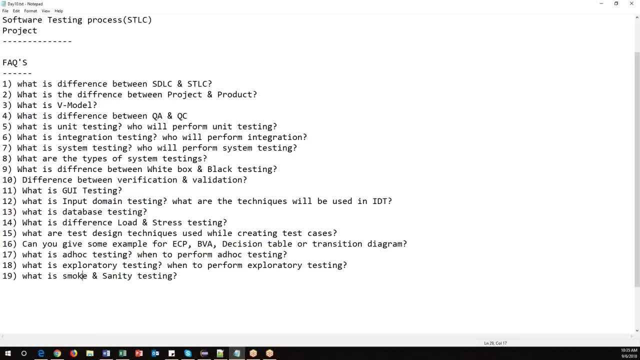 So smoke testing Make sure the build is stable or not. So sanity testing verify the test cases, the very basic test cases, and they are p1s until unless the sanity test case has passed, We cannot proceed for the test. So those test cases will be part of sanity testing. 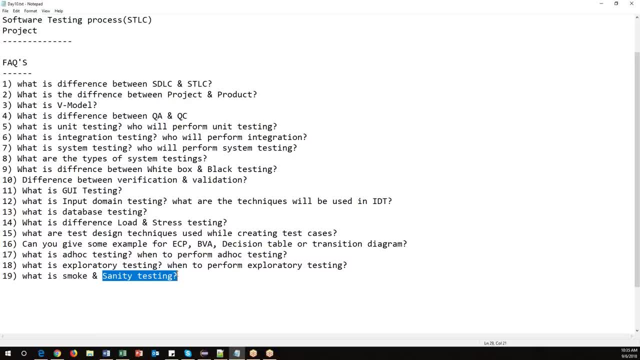 Okay, smoke testing and sanity test. So smoke testing will conduct first and sanity testing will come into the next. So in the smoke testing will make sure the stability of the build, whereas in Sandy testing the basic functionality is working Or not, so that we will verify. 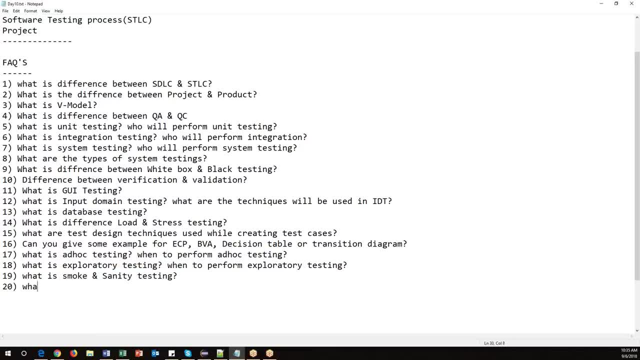 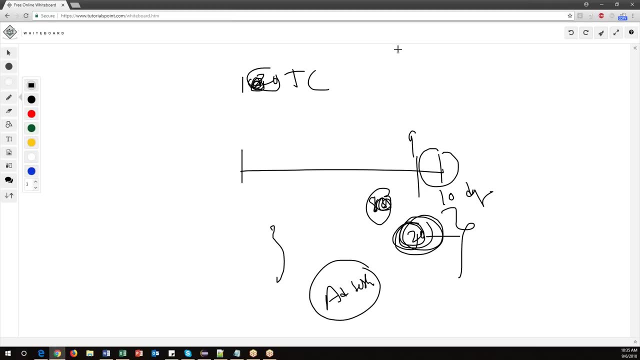 And then the next one is: what to end-to-end testing? What is end-to-end testing? What is end-to-end testing? So end-to-end testing means the complete functionality of the application. So the complete functionality of the application we have to test. suppose 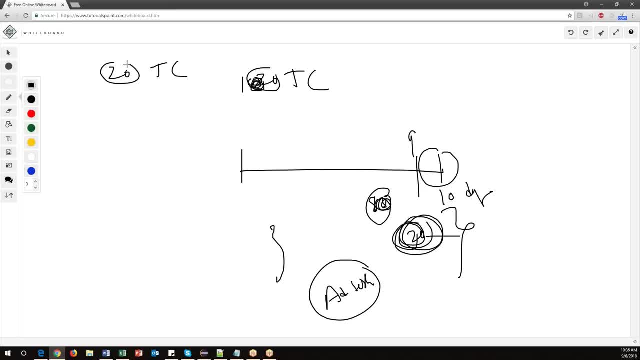 we have a 20 test cases created for the application, So each individual test case is different, but there are some test cases we should create which will Cover the end-to-end functionality. Okay, for example, I want to log in here after login. 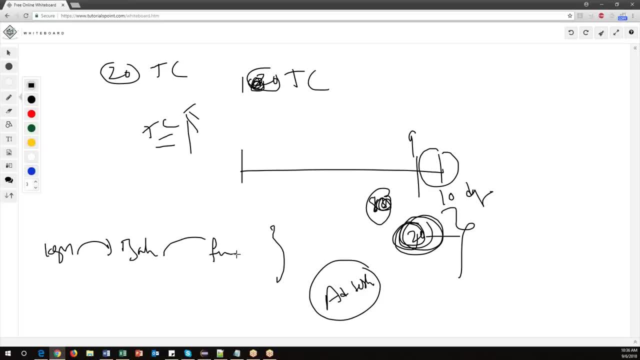 I need to verify the balance inquiry and after that I need to do the fund transfer and after fund transfer I need to check the mega balance inquiry. So this is all end-to-end flow. So individually this is all different functionalities, But if you want to cover all the scenario, 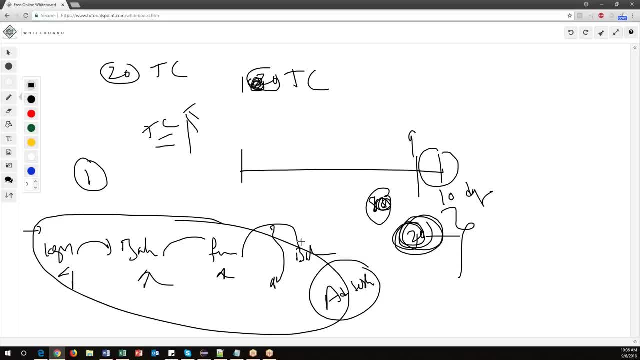 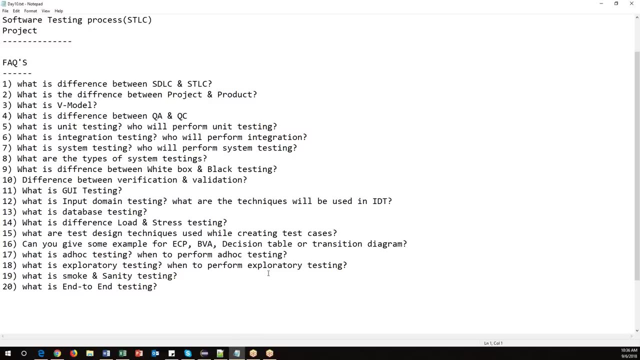 you need to write one test case and which will cover end-to-end functionality. So end-to-end is testing, is nothing but testing the complete application with respect to customer requirement. So those test cases will cover the complete functionality, end-to-end functionality. Okay, so that is end-to-end testing. just a moment, guys. 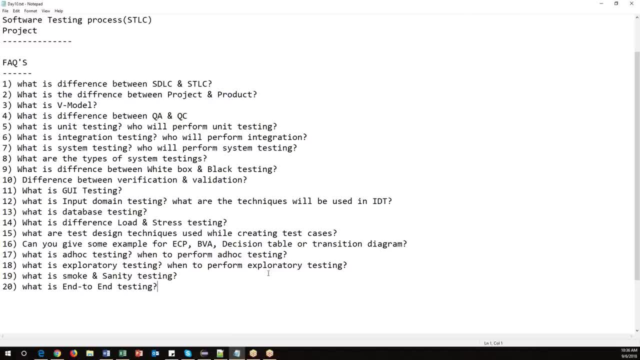 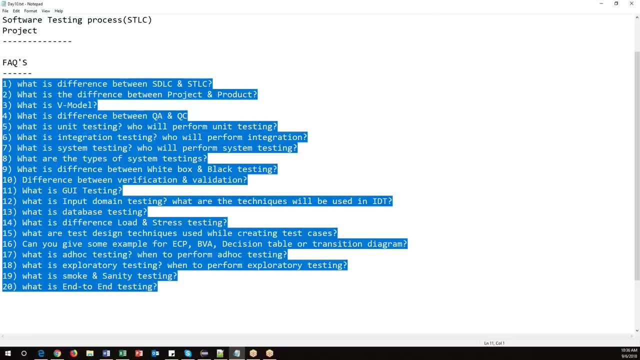 Okay, so that is all about end-to-end testing and then. so these are all comes under the testing concepts. testing concept: All these questions comes under the testing concept. very basic questions regarding the testing. So how the interview will happen Is first. interviewer will verify. 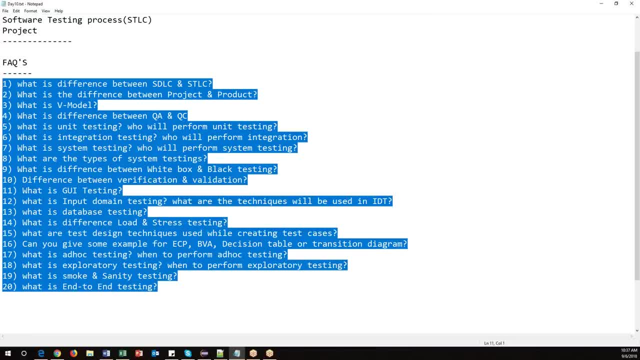 or check whether you have the basic skills or not, or you know the basic terminology, testing terminology- you know or not. so that is, they will test and once you are very familiar with the basics and all the terminologies, if you know it properly answered and then they will enter into the process. related questions: 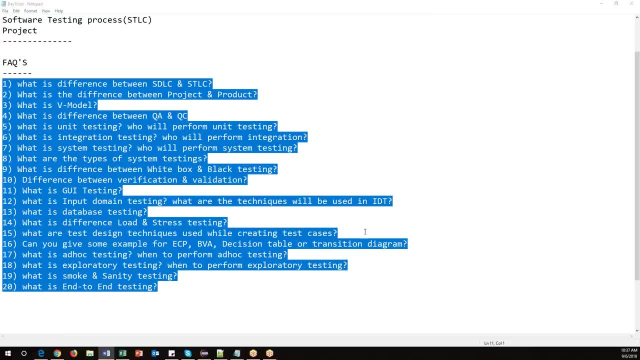 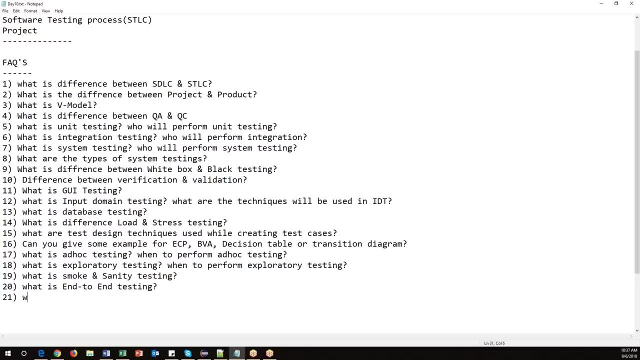 Okay, So let's discuss a few more questions under the testing process here 21.. The next question is a very important question- is: What is use case? What is use case? So, what is use case? use case is a requirement which is described by the product owner or business analyst over is responsible. 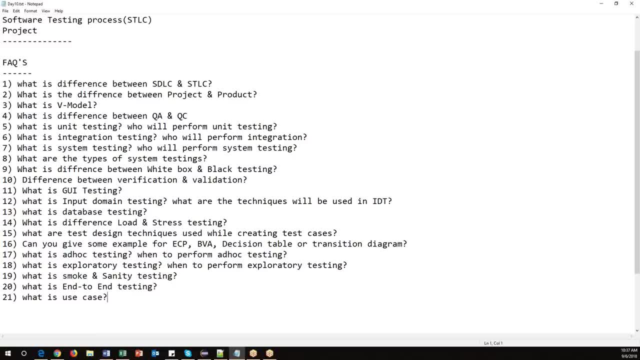 for giving the requirements. they have to create the use case. So use case describes the requirement, But what is test case? What is test case? test case describes the how to test, and here there are multiple question like: what is the Difference, What is the difference between test scenario and test case? 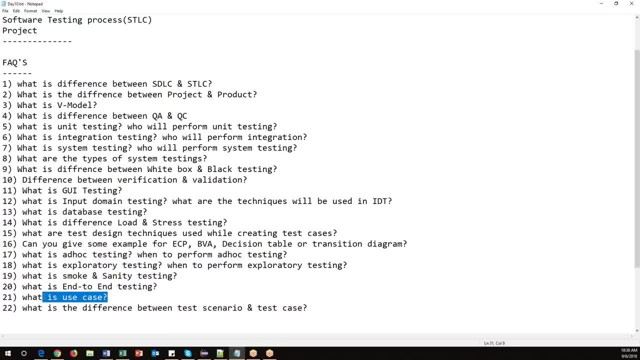 So use case is completely different. It describes a requirement, But what is a test scenario and a test case? test scenario describes of what to test, what are the different areas to be tested, and test case describes the how to test those scenarios. So test scenario will take care of what part. 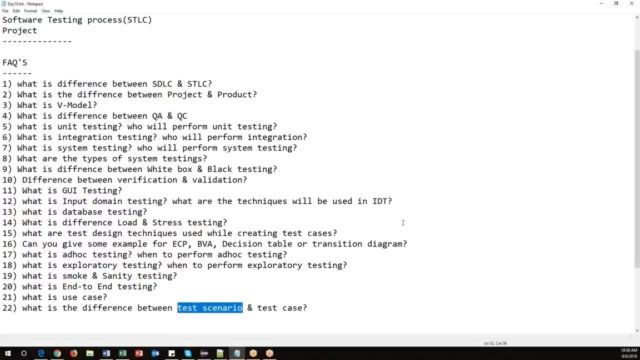 and test case will take care of how, part. how is nothing but in detail steps, step-by-step process. We will write the test cases. So, based on the use cases, we will prepare the test scenarios. for those test scenarios will prepare the test case. and use case is prepared by the product owner or business analyst. 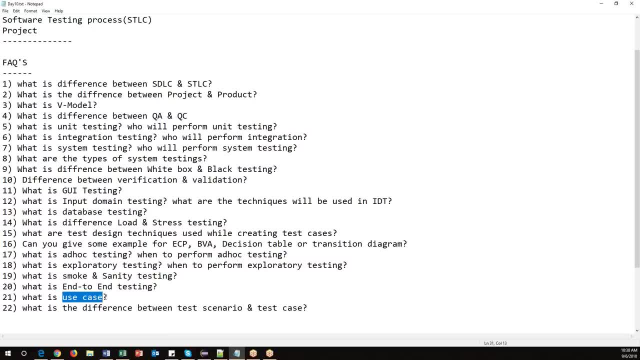 and over is responsible for giving the requirement. They will prepare the use case and test scenarios and test cases are prepared by the test engineer. So that is the difference between use case, test scenario and test case. Okay, And these are all comes under the testing concept: testing. 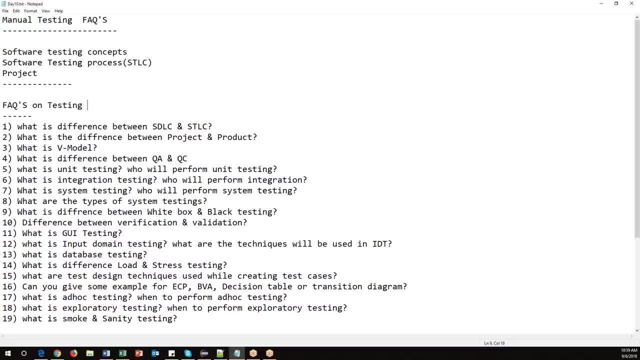 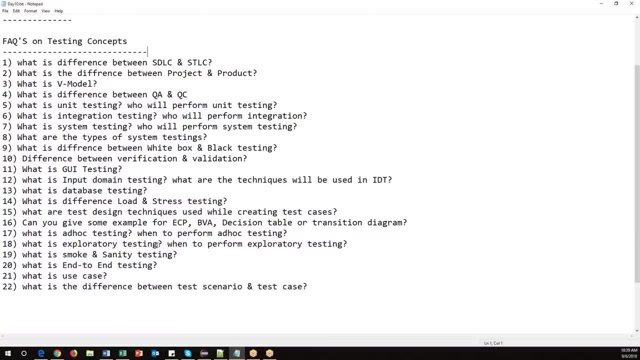 concept related questions. So if they give some testing concepts, if they give very frequently asked questions, okay, testing concept very basic. So once you are familiar with these questions, okay, then go on to the next level of questions. So the next level is if they give us our testing process. 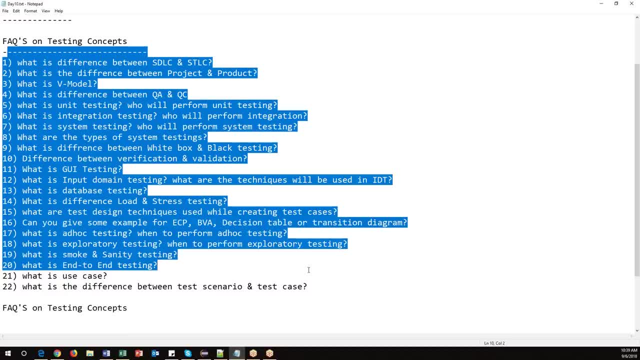 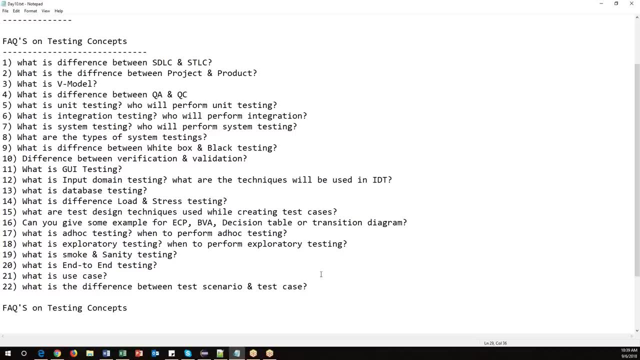 So if you go as a fresher, they will mostly focus on these questions. Okay, they don't ask any really questions on related to the process and the real-time environment related questions. Okay, So if you go as a fresher, for these questions are enough. 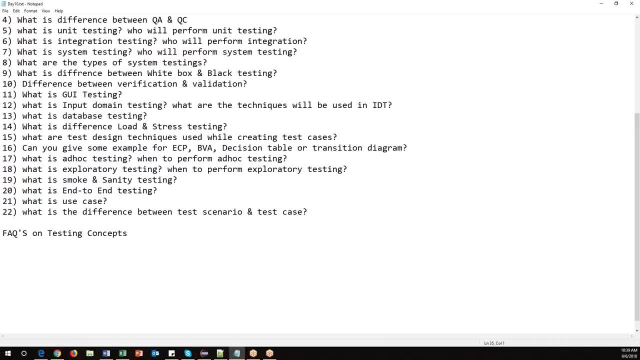 and if you go as some experience- okay hard, if you already done some project, they will expect more skills and then they will come to the next level: testing concepts. FAQs on testing process in real time. Okay, so they will ask you questions regarding testing process in real time. 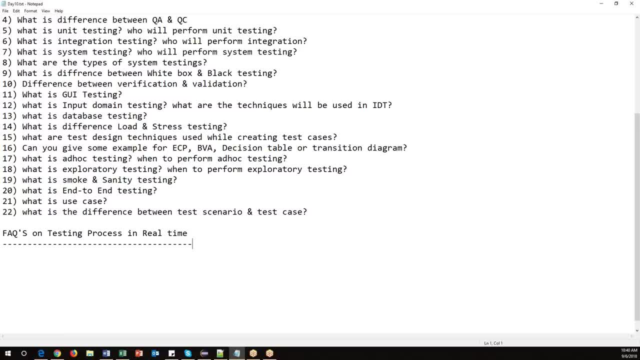 So when you're working on company, the people will follow certain process. So what is that process? how it will happen, What is your role in this process? What are, what are the different activities you do on day-to-day basis? Okay, so these kind of questions you will get as part of this category testing process in real time. 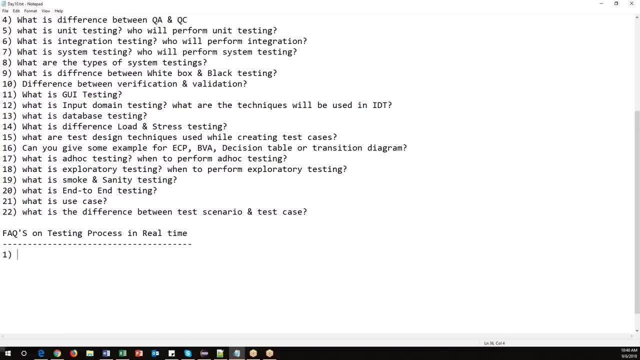 Now let us see What are the different questions you will get here. So the first question you will get here is: what is the process You will fall in your company? What is the testing process followed in your company or in your project? 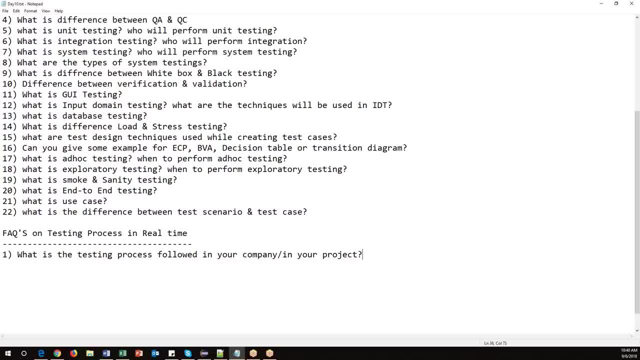 What are the testing process followed in your company or in your project? So normally, 80 to 90% of the companies nowadays are following Agile process. Okay, there is no traditional process nowhere, So you need to more talking about the Agile process. 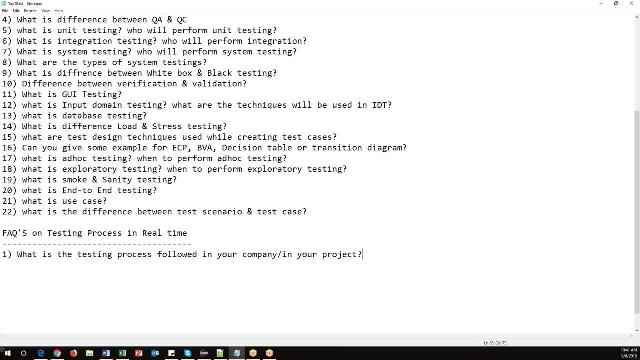 So we have to follow the Agile process. So we need to say the Agile process. So what is the testing process? means we follow the Agile testing process, Okay, and then they will ask you to explain the complete process. explain about the process in your company. 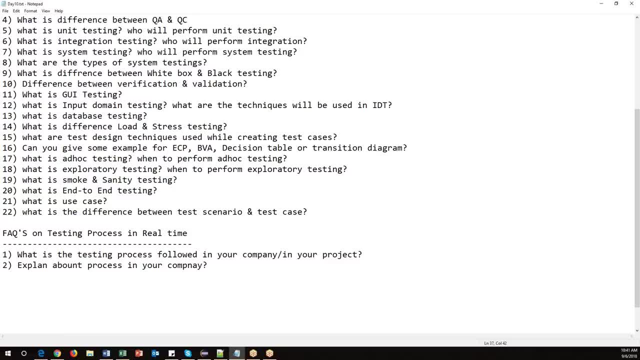 So this is another question you will get. So once you tell what is the process you are following, then they will ask you to explain about what is the different process. you will follow the company and then you have to explain the end-to-end process, like where Agile will start. 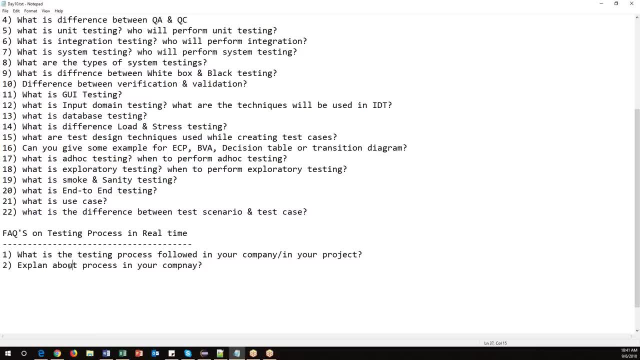 So the product owner will prepare the backlog and then sprint planning meeting, selecting the stories for the sprint and then sprint cycle will be created, estimation will be done and then we'll add the story points and we'll pick the stories for the sprint and developer and QA will create the tasks. 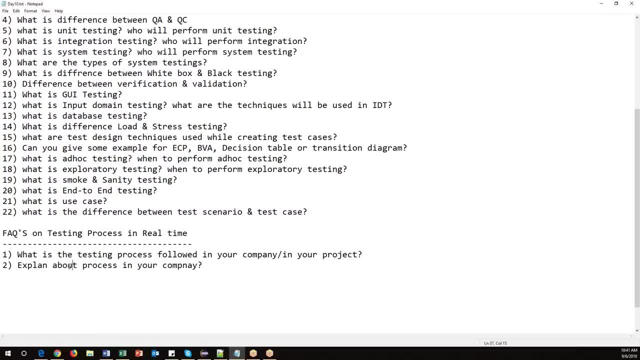 and the task will be completed between the sprint duration and after completion of this, will have a sprint review meeting, tele-scrum meeting, So all these activities we have to explain clearly. Okay, So This will give the confidence to other interviewers. 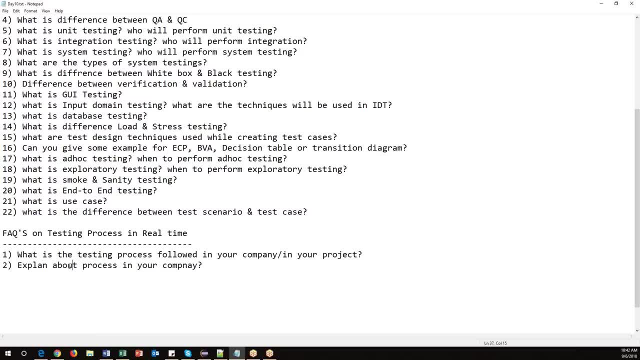 Okay, you have followed certain process. Okay, so explain about process in your company means you have to talk more on Agile process. Okay, so I already explained in the last session, So please go through that. They already have uploaded that video. that is all about process rate. explain about process in your company. 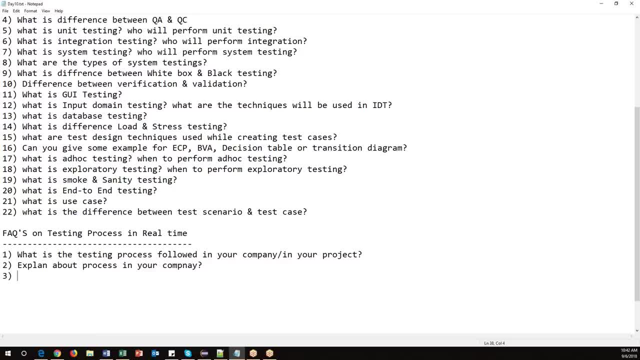 And now here you will get one more question: So how to report bugs? What is a bug reporting process? How to report a bug? Suppose, if you find a bug or if you find a defect, how we will report that. So how to report a bug? 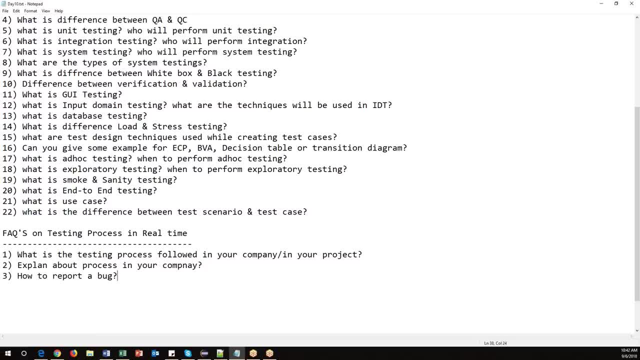 So immediately what you do, What are the steps you will follow. So immediately, everyone will tell. answer like: as soon as we find the bug, we will report to the developer. So that is a direct and straightforward answer. But you should not tell like this. 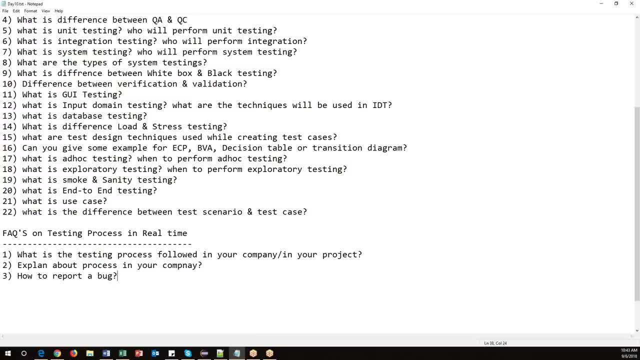 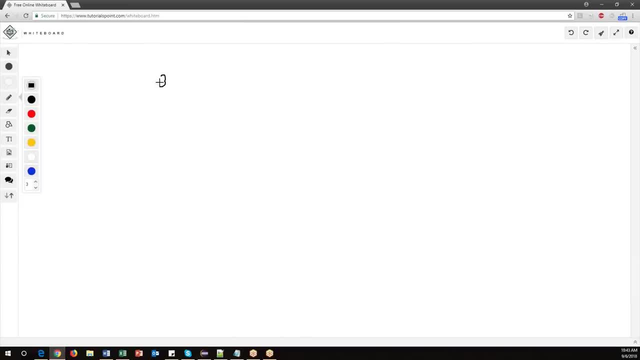 You need to just give some information in detail. So as soon as you found some defect, The first thing is you should not immediately report to the developer. So at least minimum three times your defect is able to reproduce in your environment or not. that you need to verify first. 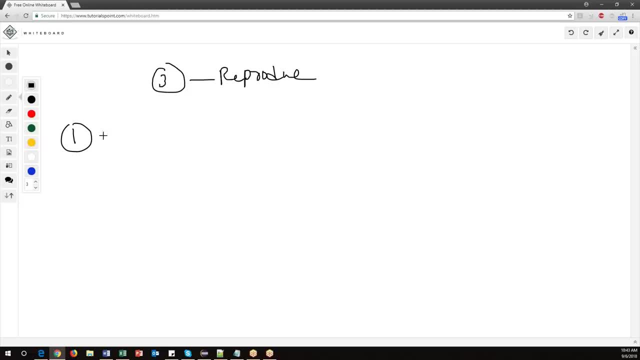 Okay, So first time you are getting the defect immediately. should not rise this into the developer? Maybe that, if it comes because of environment issue or because of invalid test data, right and because of actual real issue in the application. There are multiple reasons. 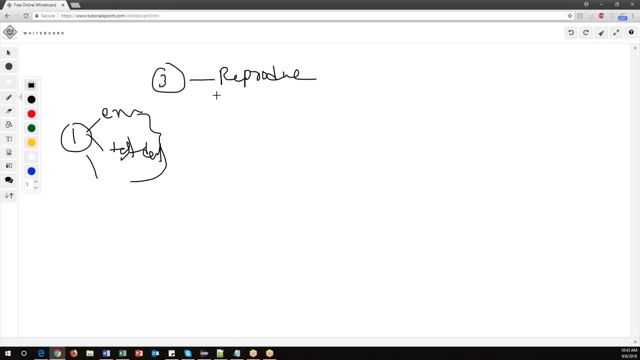 We have. so that is the reason we need to test at least three times, minimum three times- at least two environments in your system And if you have available, in some other peers, so you need to verify the same test case in other system, because whether it is related to environment error or not, we will confirm that. 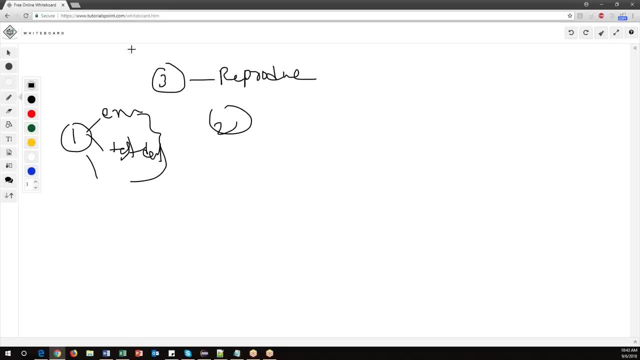 So as soon as you've identified the defect, as a first step, at least three times we need to reproduce the issue and if every time comes, in every environment it is comes, and then we will decide And the priority for that issue and then report the issue to the developer using a Jira tool in Jira tool itself. 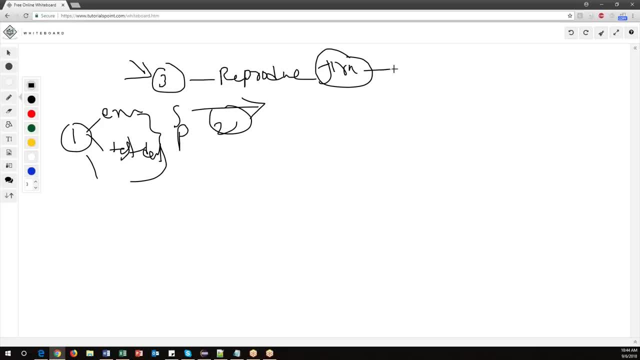 We can file the bugs. So we have seen in the previous session. right, So in the Jira tool itself we can file the bug, or some companies will use separate bug tracking tools like bugzilla and bug tracker. Okay, so our dev track. 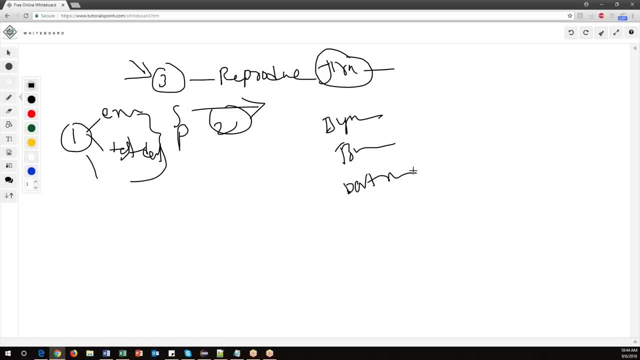 So there are multiple tools are available, only specific for bug tracking or reporting the bugs. So you need to tell all these things As soon as you found a bug, first need to recheck whether this bug is reproducible multiple times and multiple environments, and then we'll assign the severity prior to that and then report that bug to the developer by specifying screenshots, reproducible steps or all other related information. 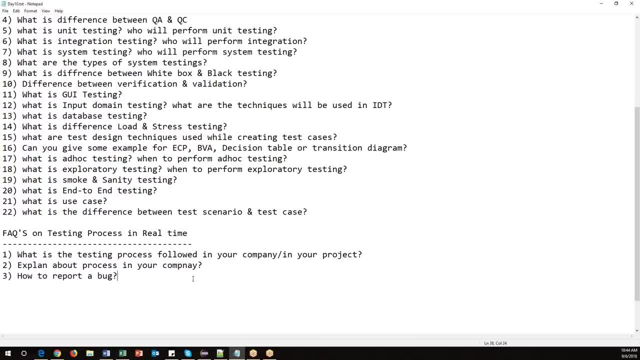 Okay, so this and all you have to tell clearly, but you should not answer, You should not give the direct, straightforward answer to that. Okay, so that is how the defect processing- If I reporting process, how to report a defect- means you have to do all these things, have to tell all these things. next question: 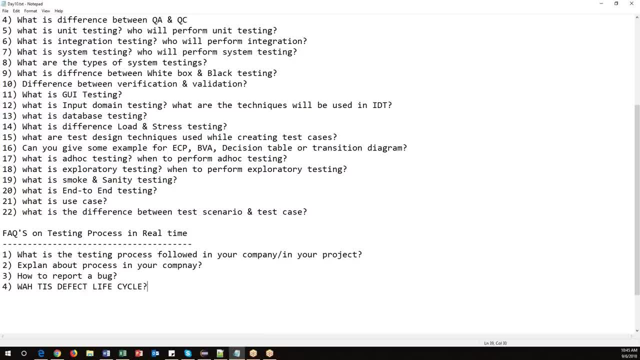 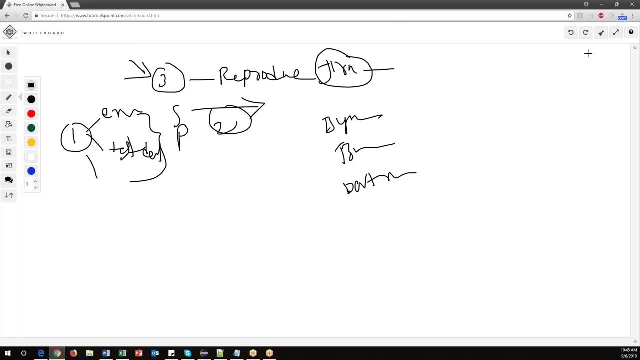 You will get: what is defect life cycle? What is defect life cycle? What is defect life cycle? So in the defect life cycle means you have to explain everything. So from the beginning the defect will be like this. So you can just explain by taking piece of paper and draw some background. 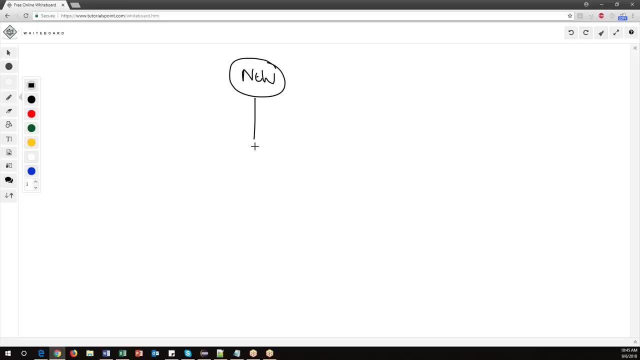 So whenever You find the defect it will be the new status. So when it is every time it is reproducible, Yes, then you will report as a defect and here the developer developer will work on the defect and reproducible: Yes, then developer fix this issue. 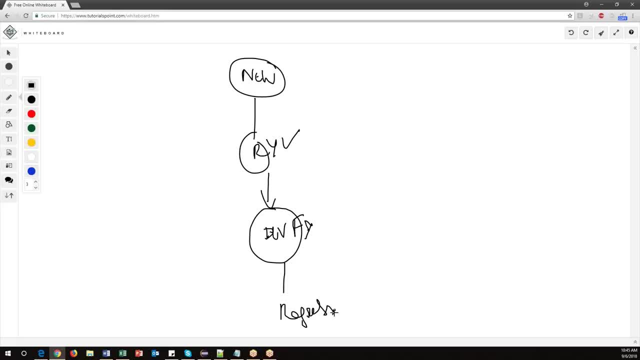 So once he is fixed, we have to perform the regression testing on this or retesting on this, and if the retesting is passed and then we have to close the bug and if again retesting is failed, again we need to reopen the defect. We need to reopen the defect. 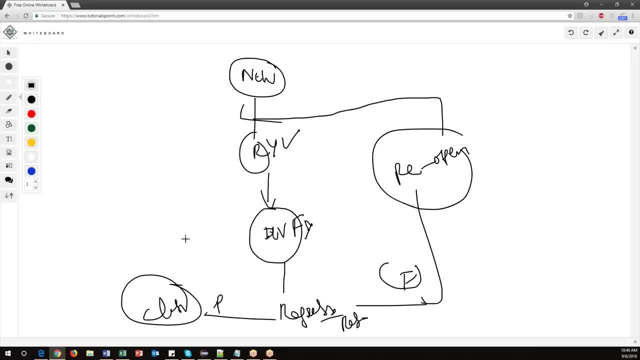 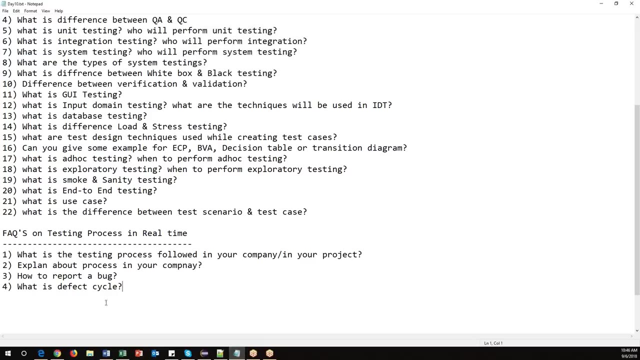 and again we need to report the defect to the developer. Okay, This is a cycle We have to form. this is called as a defect life cycle or bug life cycle. Okay, So, from the beginning to close the bug, how many cycles or how many statuses it will go through, that's called as a defect life cycle. 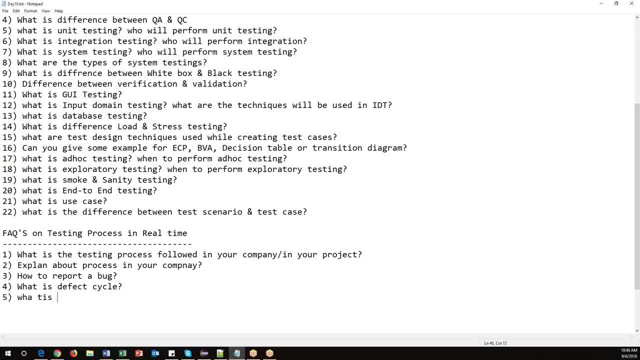 So what is defect life cycle? and next question will get: what is So what is priority And severity? So what is priority and severity? So priority means importance of the defect, whereas severity is a seriousness of the defect, How well the defect will impact the system or impact the function. and that is basically severity, how seriousness it is. 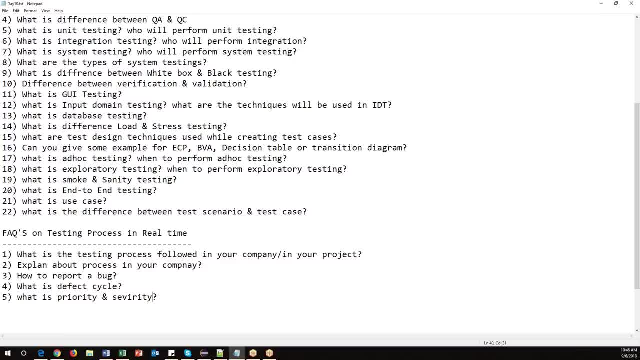 and priority means, in part of the importance of the defect, how early the defect should fix, So that will be taken care by the priority, Whereas severity means how well the application is crashing your, how well the defect is crashing your application. So that is about the severity. seriousness of the defect, importance of the defect. 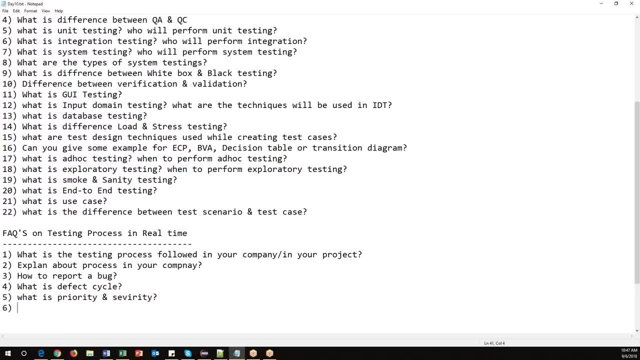 Okay. so you have to give clear idea on this. and one more question you will get up: Give me an example. Give me an example, Okay, high severity And low priority, And also high priority and low severity. So these questions you will get so low, high severity, low priority and high priority in the low severity. 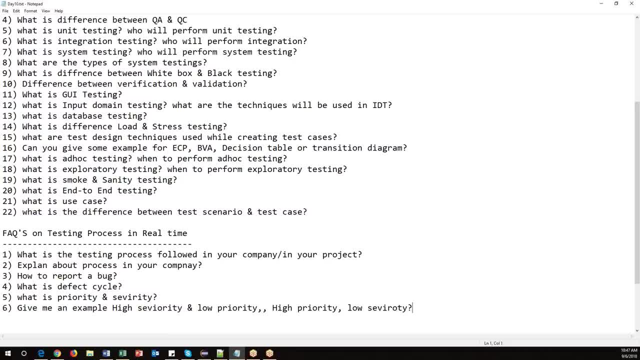 So give me a few examples So you should able to answer this question by giving some examples. So I already given a lot of examples in the previous session in the presentation. So you can just go through that, just remember one or two examples and then you can easily answer this question. 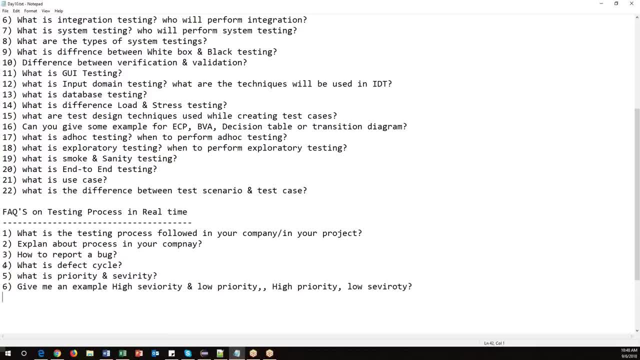 Okay, So severity and the priority. And the next question you will get is related to And the priorities and test case. So how to write test cases, How to start writing your test cases. These are all real-time experience equations: How to start writing your test cases. 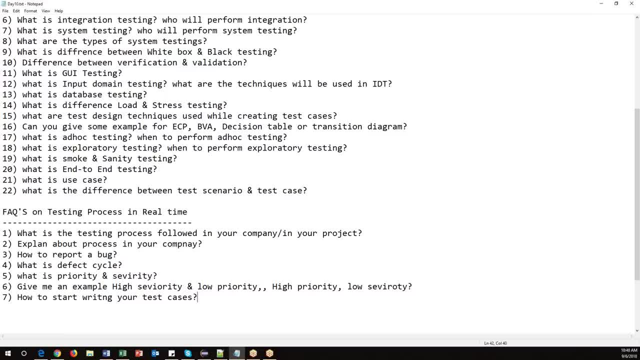 So what is your prerequisite? You have to tell everything here. So as soon as we get the requirements or as soon as you get the stories- and if you are talking about Agile process, you should not use these kind of terms of the requirement- test planning, test designing. 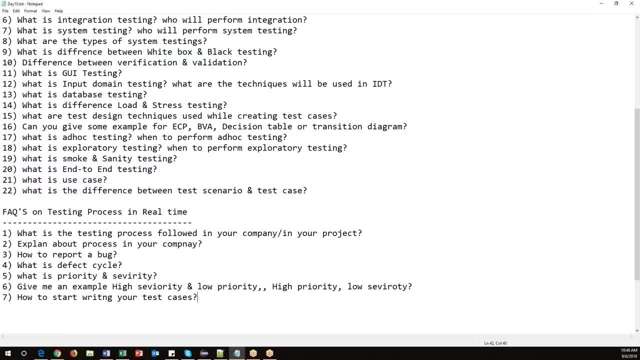 Okay, So these terms please try to avoid it. Okay, So in Agile process we always talk about story or epic sprint. Okay, scrum master, scrum team, So just use these words. So how to start writing your test cases means as soon as you are getting the stories. 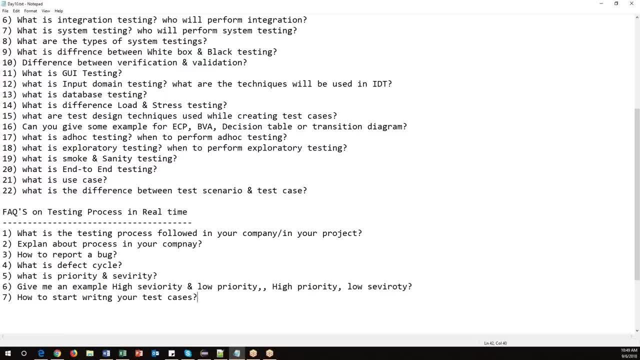 and once it is reviewed, and then you will start writing us to test cases for those particular story. Okay, And what is the input here for writing the stories? writing the test cases, stories or the input document, and stories are the input for you. So even in the stories also, we have a clear use cases, the based on the use cases. 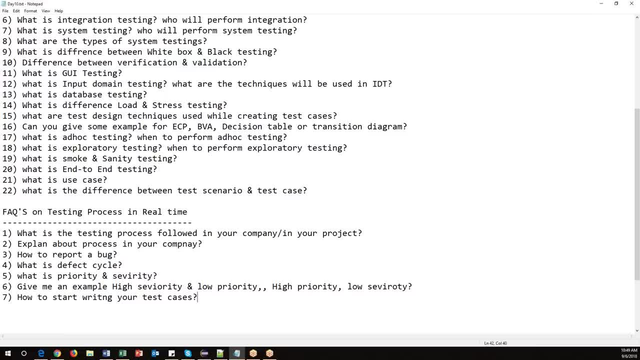 while reading the stories. we can just create the test case, and sometimes the developer will also provide the vice. greens ice cream means the UI screenshots, some model screens, Not so. based on that Also, we can write a word: test cases. So once we have to write your test cases, 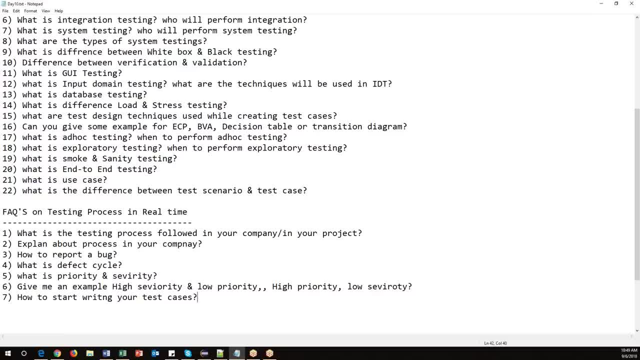 we need to review them with your team and then finally get the approved by product owner. Okay, So that's how, what? how to start writing your test cases means you have to tell all these things and, in other words, people will ask the same question in different way. 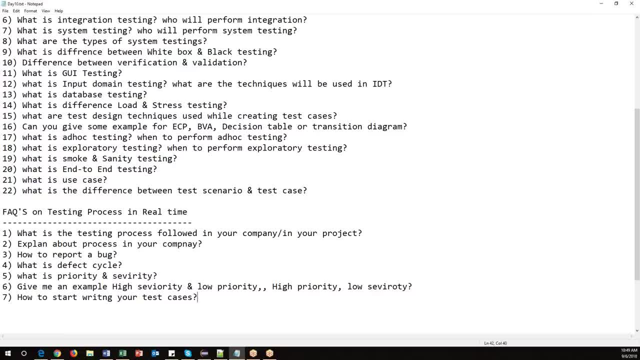 So what is the, what are the inputs you will refer while you are creating your test cases? What are the inputs you needed for writing your test cases? So we have to tell user stories And why screens are use cases. So these are all input documents to creating your test cases. 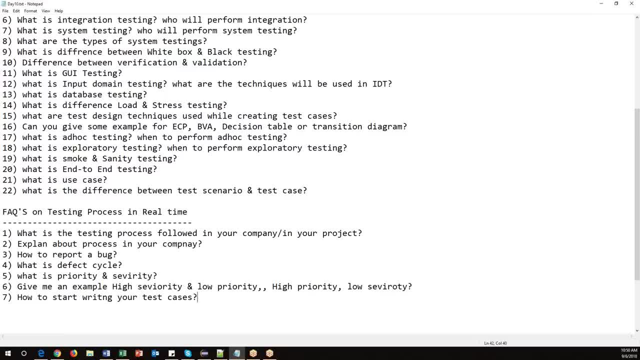 How to start writing your test cases. We have to tell all these things, Okay. So these are all process related questions and sometimes they will. people also ask you the questions like: what is your role? What is your role? or you can say, what is, what are your responsibilities? 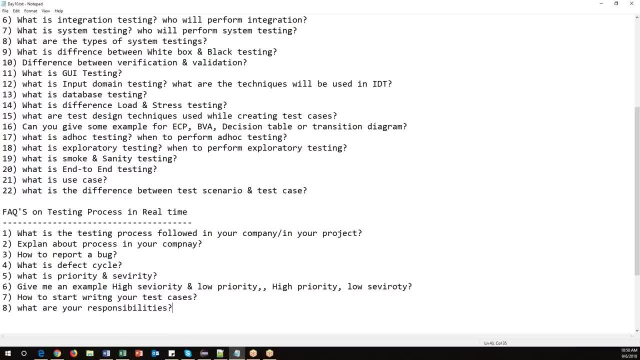 What are your responsibilities. or you can, in other words, They can ask what are your day-to-day activities in your project. Okay, you have to tell all the things like what is your rules and, day-to-day, on regular basis, What you will do. so you will normally write the test cases. 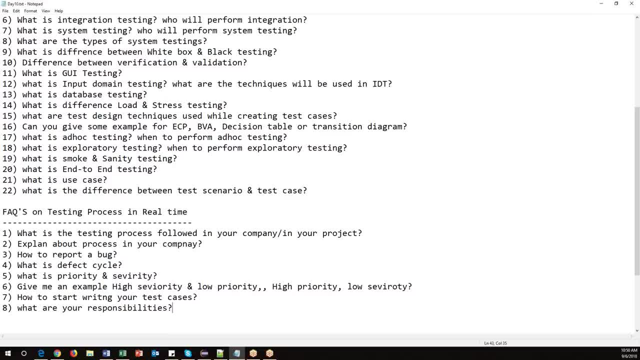 and sometimes you will execute our test cases and sometimes you do retesting and regression testing and sometimes you will participate in the review meetings, Okay, and team meetings, all these things we have to say, but if you are working on six to eight hours of time, so all six hours, eight hours time. 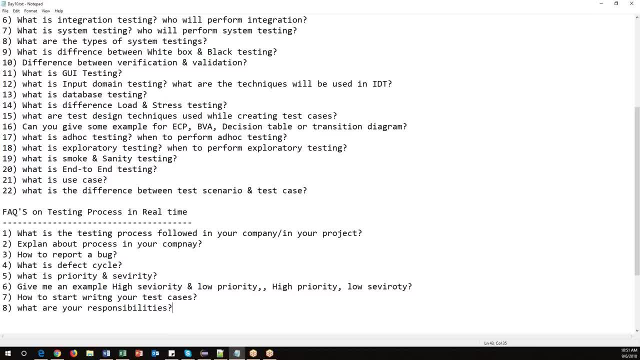 you don't do writing test cases, You don't execution to. all these things will be done on hourly basis. Like, suppose, if you're working on six hours, all six hours you don't spend on writing test cases, like all six hours You don't spend to review meeting. 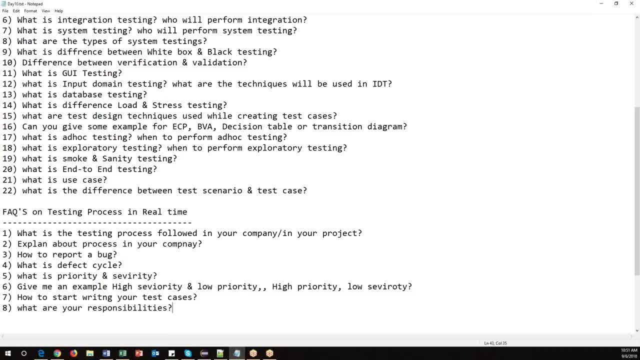 So some hours will spend to something like almost six hours, You are suppose. if you count eight hours, almost four to five hours will be execution part and two hours will be documentation and one to one and a half hour will be attending The meeting and other stuff. 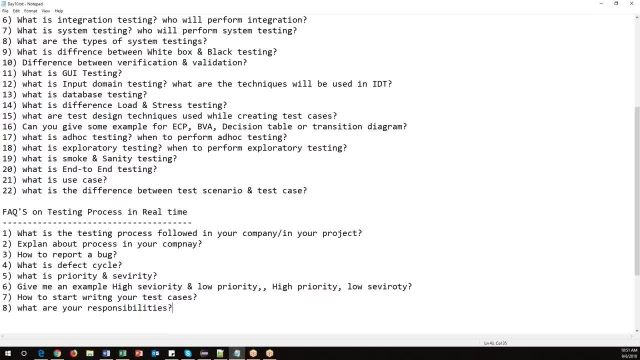 So you have to divide the your entire day in different tasks, You have to allocate your time to different tasks, Okay, Fine, So is it clear? everyone? so the nature? can you hear me now? Okay, Okay. So these are the few questions you will get related. 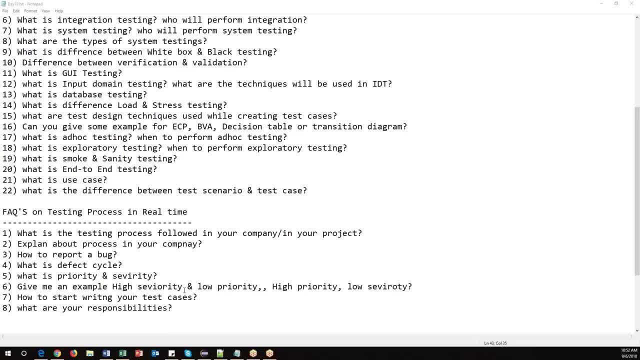 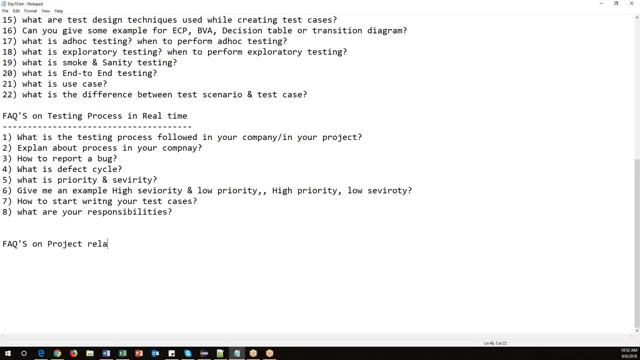 to the testing process related. What is the process you are calling? What is a? all the stuff? Okay, and then let's move on to the FAQs on project related. FAQs on project related. So what are the different questions you will get on the project? 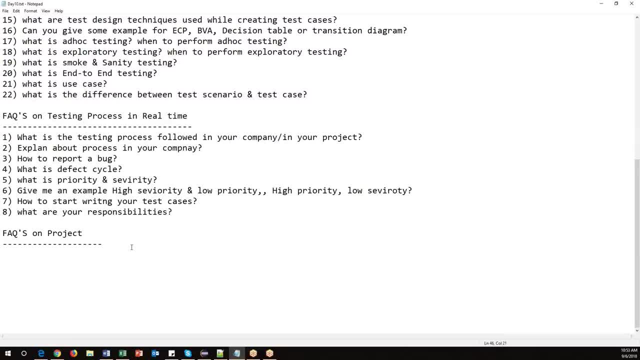 So on the project. so you will get different questions. If you have some experience on the project, if you show your showcase, up some project in your resume, then you people will ask you some questions related to your project. Okay, the first question you will be getting is explain your project. 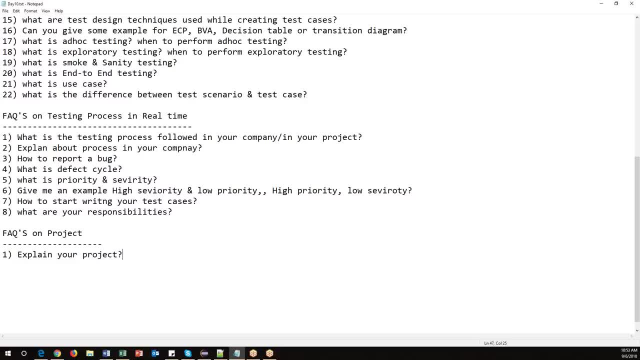 Explain your project, Then you have to start All the stuff regarding your project. first, You need to tell about what is the domain of that particular project, whether it is e-commerce project or healthcare project, or it is a portal, or it is a some different kind of domain or banking project. 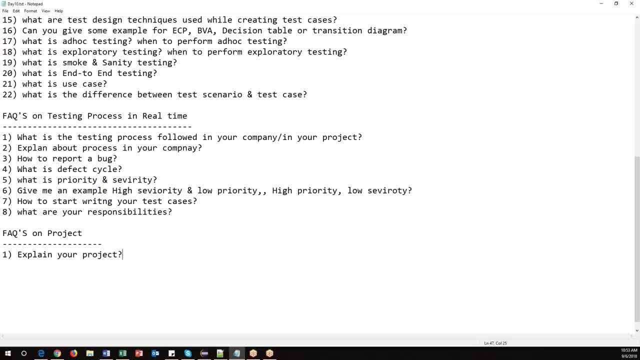 So these are all different domains, or it is insurance project or financial project, So what kind of domain it belongs to, so that you need to tell about. so explain your project means first You need to tell about the domain, what kind of domain it is. 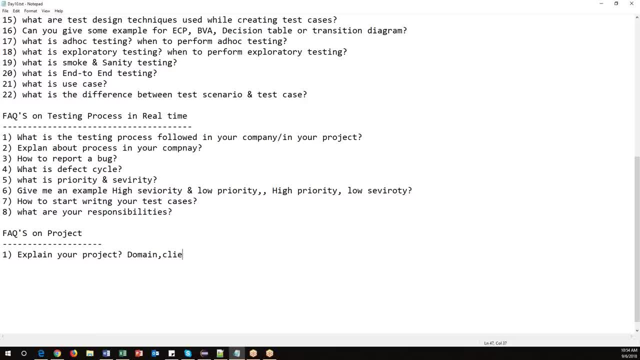 And the second thing You have to tell about for which client you have developed this project, for which client you have developed this project. Okay, so this is one more important: the client name also. you should tell, so for which client you have developed this project. 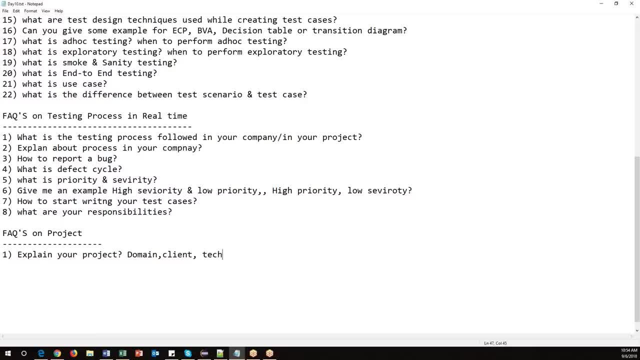 The client name is important. And the second thing is: what are the different Technologies we have used in this project? What are the Technologies? the Technologies in the sense of developer point of view. If you say he can say like Java and web services, I think our back-end has like my sequel. 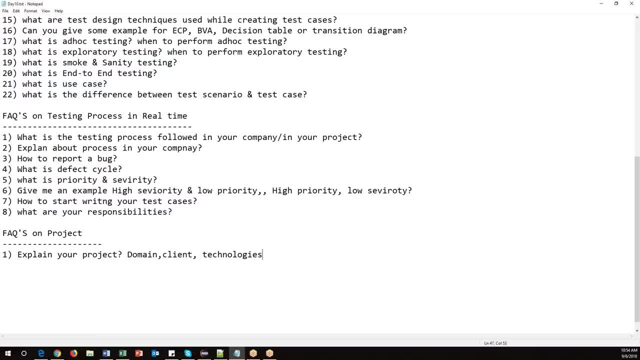 So they will tell those kind of Technologies and, as a testing point of view, along with those Technologies We need to also tell about what are the tools we have used. So, for writing the test cases, we have used templates or we have used Jira tool. 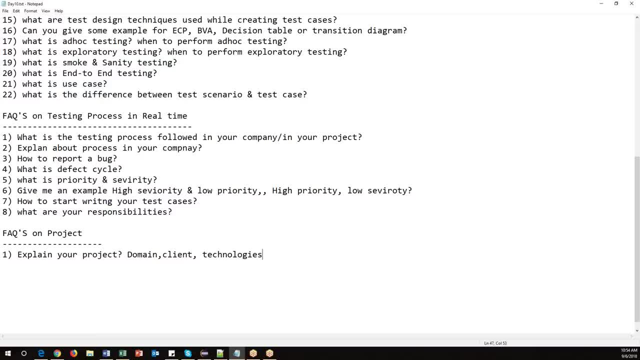 and specifying the stories, and for agile process, We have your Jira tool. and for writing test cases, We have used templates, and for bug reporting, again We have used Jira tool. So all these things we have to tell. Okay, so these are all about the project first. 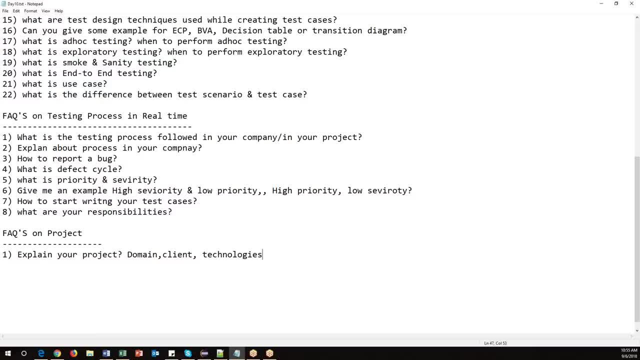 We need to talk about the domain, and then we need to talk about the client, and then we need to talk about the different Technologies used in using project. So that is about one more important thing. So, and how much team? so how many people are worked in this team along with you? 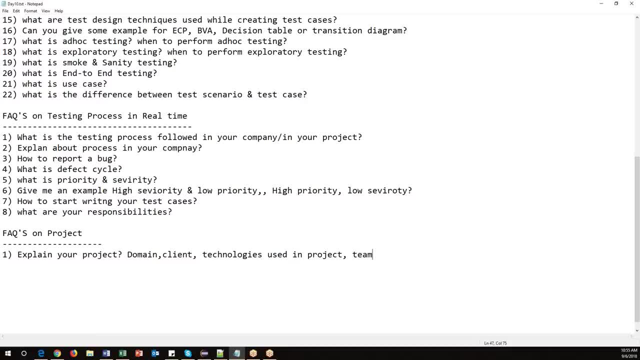 How many, how many other people or work together, So that also you have to tell. so, once you tell these items, and then you need to start explaining your project, Like how the flow will be, What is the functionality of your project, What are the different inputs. you have to be 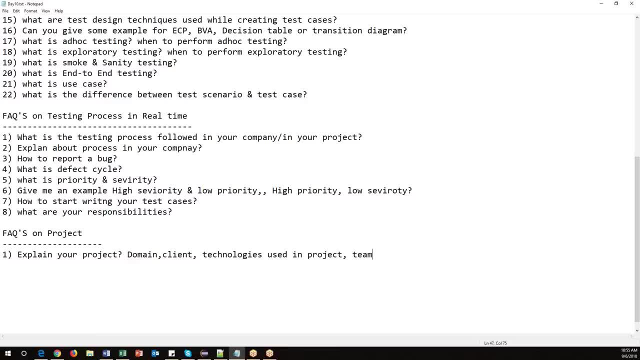 and what is, or what is the outcome of your project, What are the different functionality you have tested. So all these things you have to explain by taking some paper and pen. you can just start some, draw some pictures and you can just explain end-to-end flow of your project. 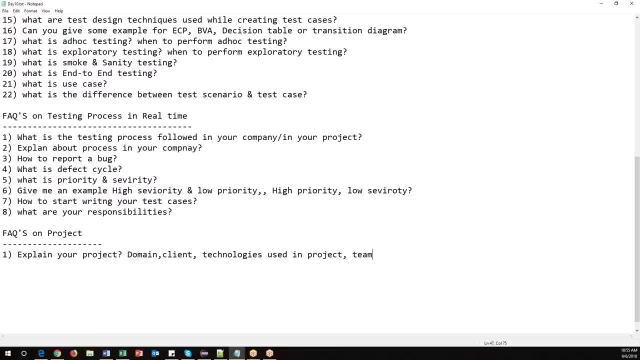 and whatever areas you have worked, all the functionalities, how you have tested, how many test cases you have written for that. So all these things you have to explain, Okay. So first you need to start with the domain of the project. Who is the client? 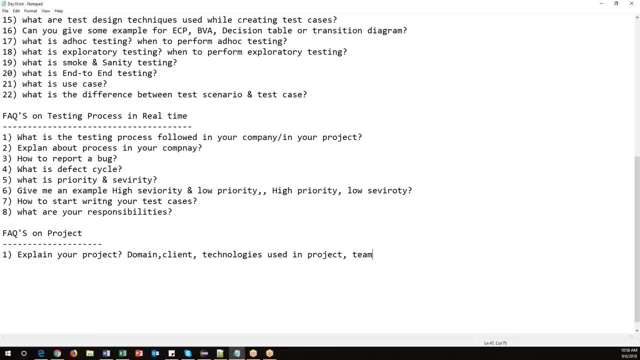 You have developed technologies used in your project and then team size. So once you have explained this, then you have to start it about the functionality. So explain something, or else talk something about your project. Talk about your project or some functionality, Okay. So that's how we need to give the explanation about your project. 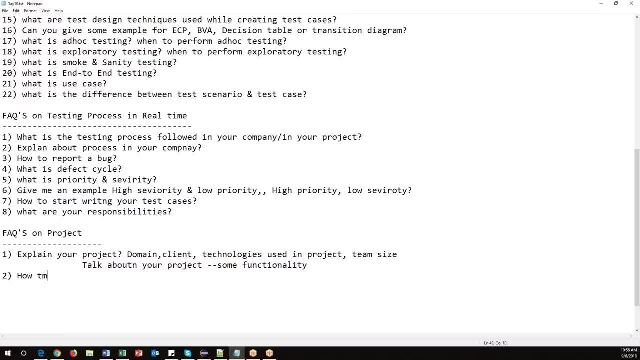 and then you will get question Like how many? how many test cases have you written? or how many test cases have you written for your project, For your project? So how many test cases have written for your project? So normally that again depends on the size of the project. that depends on the size of the project. 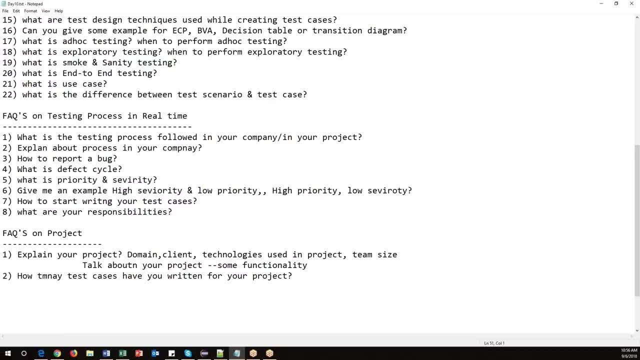 So, for example, let's say: let me take the three sizes. So for this is small project. Let's say it is. Let's say this is a three months project, three months. and let's say one more project like medium-sized project. Let us say this is our six months project and large-sized project. 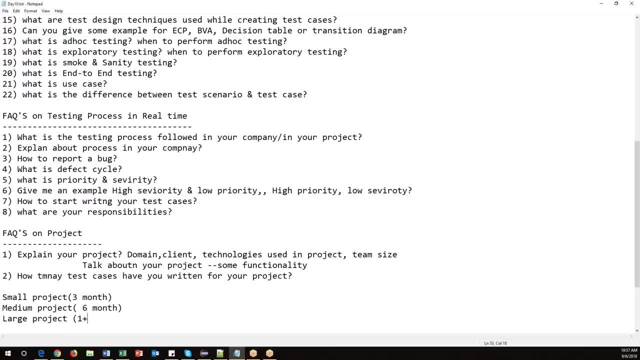 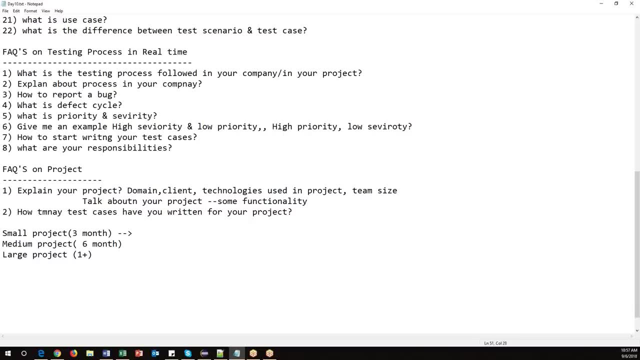 So large project or is that suppose is a product, So let's say one plus years. Okay, let's categorize three different kinds of project for three months: project approximately, If you think about, if you write at least 10 test cases per day. 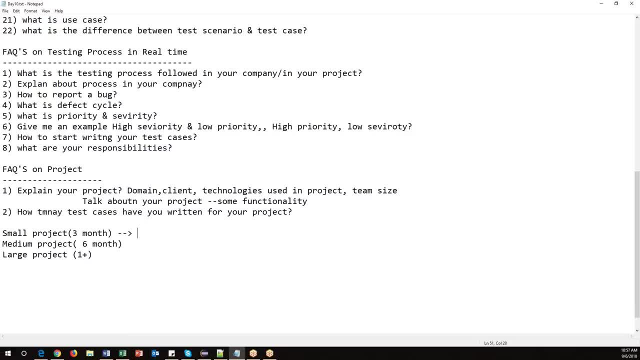 Okay, For three months every month. You just assume that. only 15 to 20 days, not more than that, and the leaves and everything is just cut out of, just take it only 15.. So 15 into 10. Let's say 150 test cases. 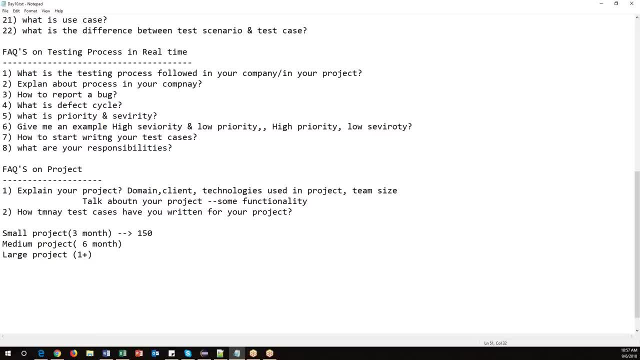 You can write for one month, So 150 into three. So how much you will get? so we can just say approximately that those many number of test cases you have written for the project. So you need to always tell approximately, should not give the exact number. 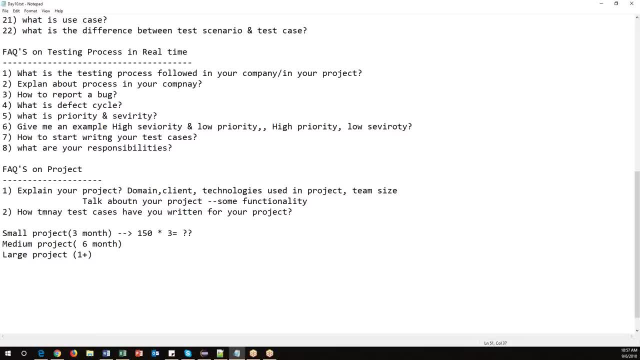 You should say approximately. We have Created these many test cases for your project and you need to decide based upon the size of your project. Okay, suppose if the six months it will be doubled and again it is a one year, again This will be double, tripled. 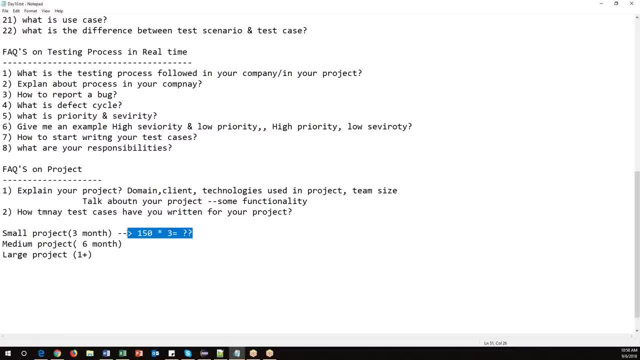 Okay, so you need to tell like this and per day, on an average, How many test cases will you able to write? means you have to tell like this: more test cases means small in one, four to five lengths of s case with a small test case. 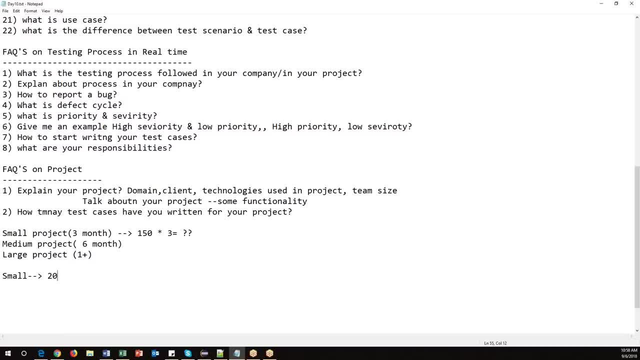 You can just write almost 20 test cases. 20 to 25 test cases. You can write If it is very small and if it is a large test cases, like if it is more than 10 lines of test cases. mostly you cannot write more than five test cases. 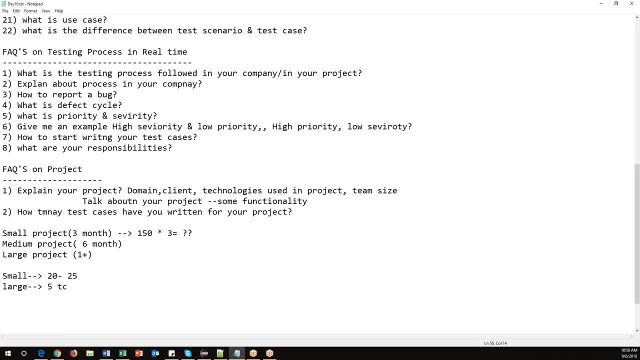 Okay, So this is just approximate number You can just provide at the time of injury. these things you have to prepare before itself. Okay, before going to interview, We have to prepare all these things. and then you will also get one more question, like how many defects you formed, how many defects you reported? 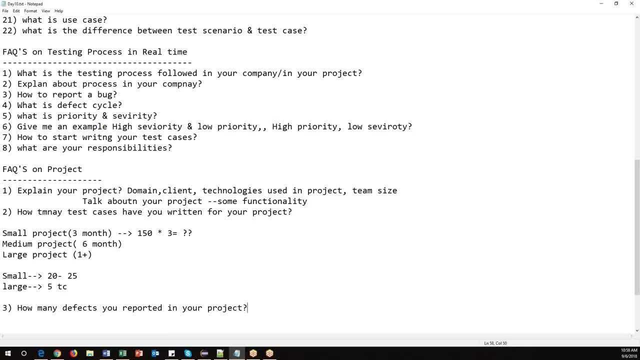 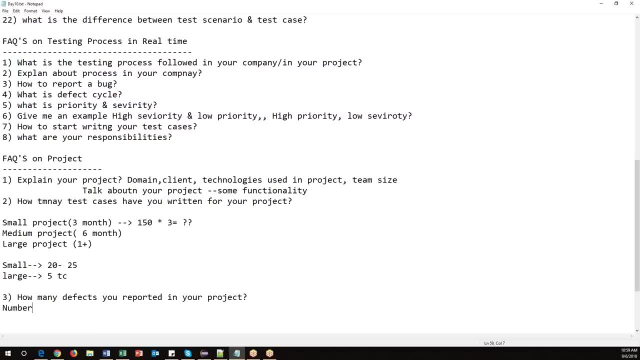 In your project. Okay, how many defects before you reported in your project, So that also you need to remember. So, how many defects you are reported? There's some number should be required, So that is not. we don't have any specific data like 1, 2, 5, 10, like that. 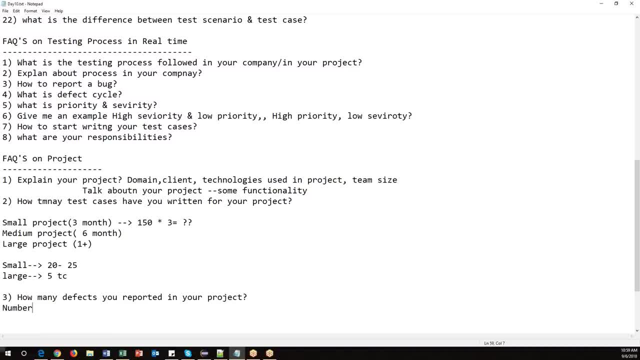 So we can just specify how many defects you reported in your project. Suppose, if it is three months project, you can just say 15 to 20 defects. you reported something like this. So this is not constant and this is not fixed. So that is again. 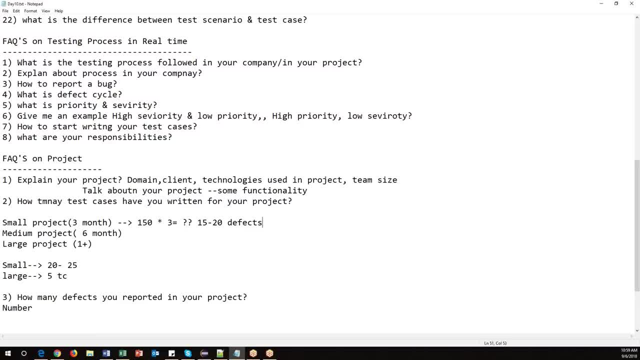 It can vary from project to project, based on the duration used, based on the tester efficiency. So there are a lot many factors We need to consider before telling this number, Okay, and how many defects you reported in your project. You have to give some number. 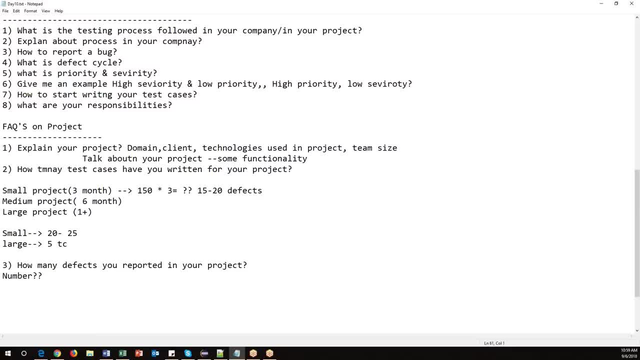 Okay, and then again, if you want, if the people want to ask, you say how many people's you have reported, How many people's, how many people's? if they want to go in detail, they can make them ask. these questions also related to the defects. 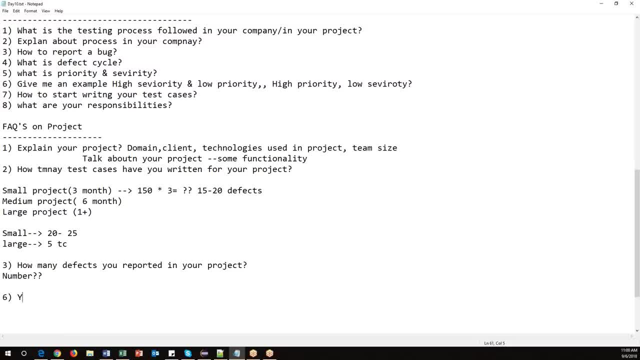 Okay, and one more important question They will ask you suppose you found, you found a defect in QA, but there is not able to reproduce it. not able to reproduce it Now, what you will do So? what you will do now. So you have reported a defect to the. if you found a defect in QA environment, you report it to the developer. 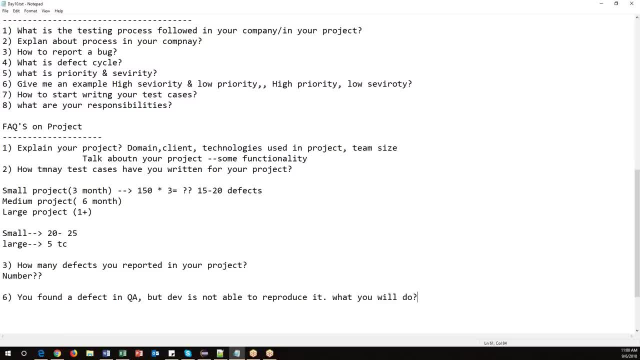 but developer Want to fix it, but before, if we want to fix it, he should able to reproduce it. So, but developer environment is not able to reproduce it. So what you will do? So that is the one question you will get. 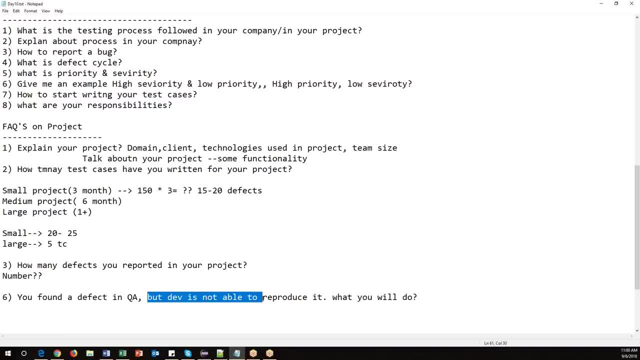 So what you need to get is: We don't know about developer environment, What, what environment they are working on, but we need to always consider about QA environment. So ultimate goal is: everything should work on QA environment. So, if it is working somewhere, if it is not working somewhere somewhere, 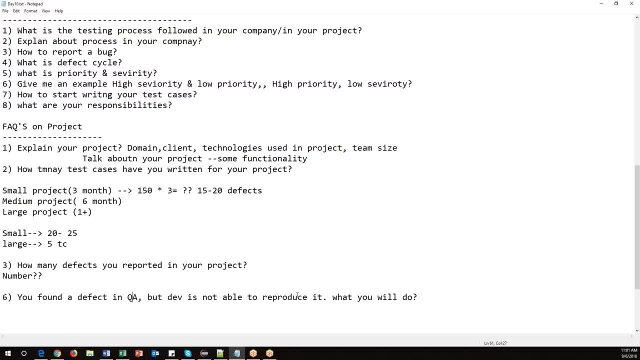 we should not care about it. So if it is not working in some environment, that is a final for us. Suppose, if it is working, QA, suppose. if you leave that bug, okay, development environment, is it working. so we can just take it as a light. 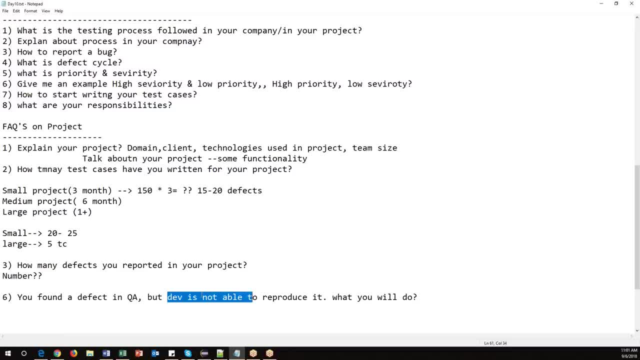 Then suppose the same issue will get customer customer also will get the same issue in their environment. So in these cases we need to take very seriously and we should not leave the bugs in the customer environment. Okay, so we need to approach the developer and not only one machine. 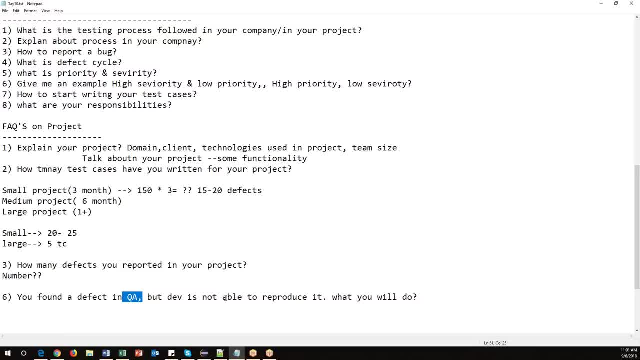 We have to try to reproduce this multiple systems And we need to in detail debug it. And what is the different criteria, What is the different root causes for getting this issue? Maybe the environment issue, maybe the data issue, or maybe the some memory issue or operating system issue? 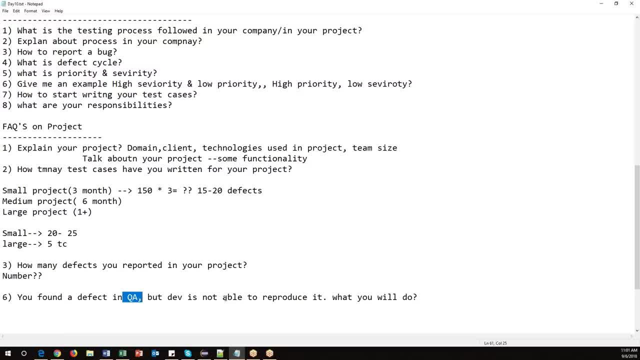 So our browser issue, So we need to always think about in different aspects. Okay, so there's a one question you will get and the one more question You will get, like you have a reported defect or you reported a defect to the developer. 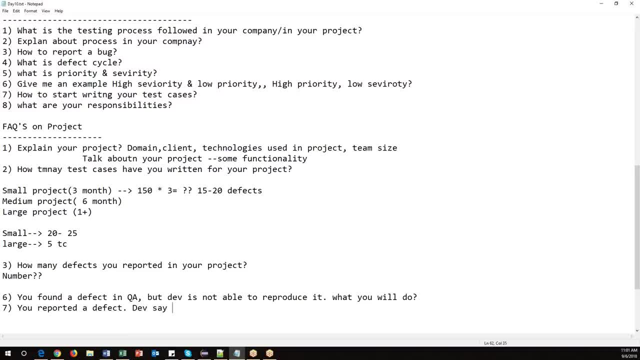 Okay, but Developer is not accepting. developer says it's not a defect. It's not a defect and it is. it is, it is as per as per requirement. So you found a defect, you think it is a defect, you report it to the developer, but developer is not accepting. 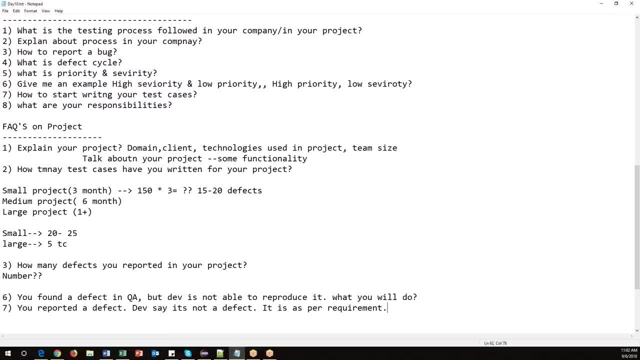 It is a defect, He says is a. it is not a defect, is working according to customer requirement. So there will be some conflict between QA and tester, QA and developer, right. So in these cases you need to just approach product owner, because he is the guy has to tell what is the requirement. 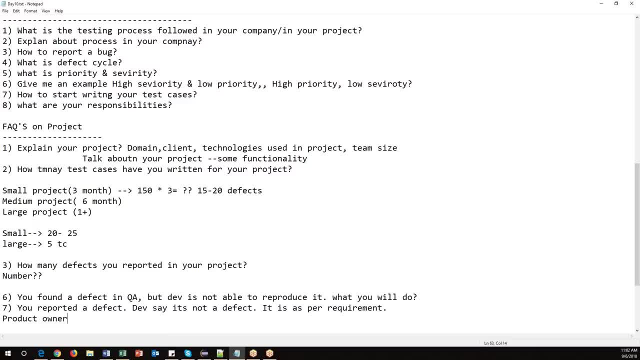 What is not exactly right, which one is correct and which one is not correct. because he is the guy we has to communicate with the customer and getting the requirements and stories for us, So he has to take the final decision, Okay. So suppose, if you say okay, 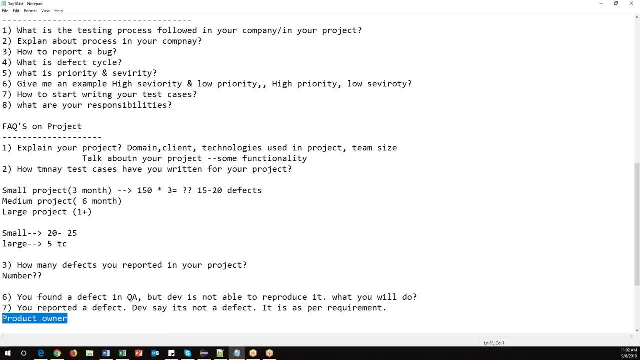 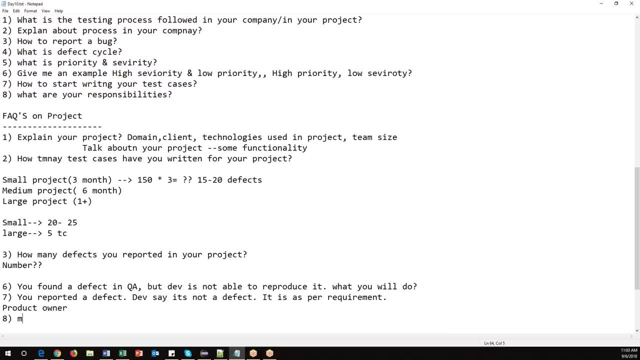 this is a defect means that is a defect, And if it's not a defect means we can just ignore it. Okay, So this is a very important and the other one. people will sometimes will ask you: what are the different metrics you will follow in your company? 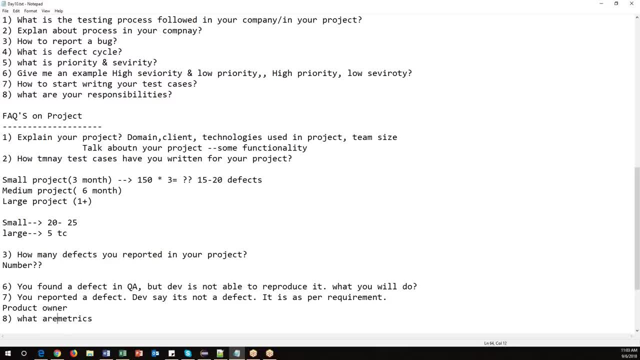 What are the different metrics? test metrics, What are the different test metrics will follow. So normally, test metrics means on the day-to-day basis report you will find, you will send like how many test cases have executed and always reported this matrix in the percentage. 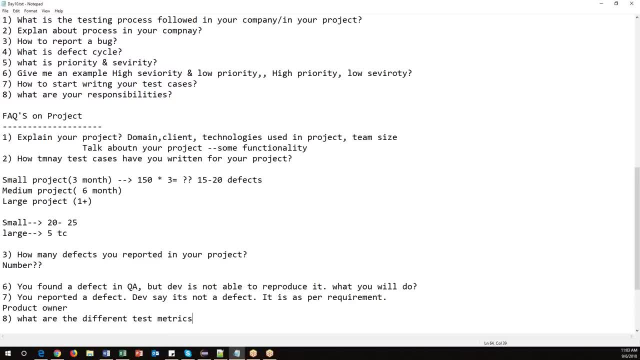 Okay, we don't give the numbers on this. So how many percent of test cases you have executed, How many percentage of test cases have passed, how many percentage of test cases failed? and, along with this, test efficiency- test effectiveness will be calculated by the management team- and defect density. 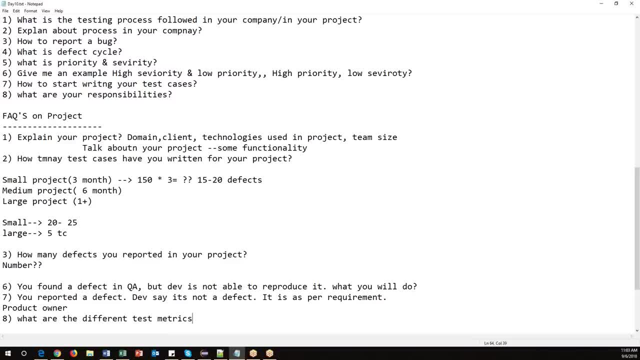 How many invalid defects we have reported, how many valid effects we have reported. So all these things comes under the test metrics. Okay, so I have a clearly explained all the test metrics in one session, So please watch that particular recording. Okay, So these are all related to project related questions. 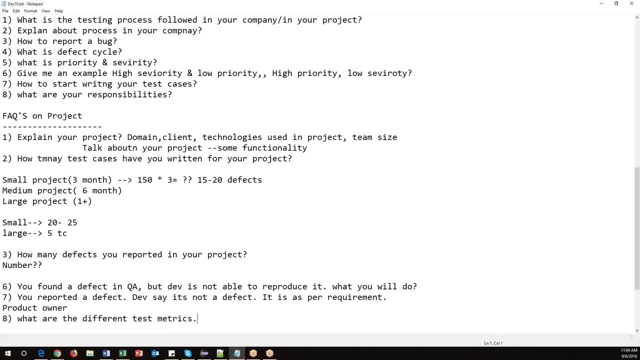 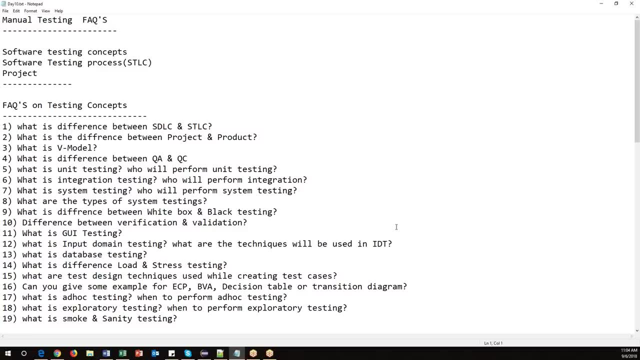 Okay, these are all related to project related questions. If you put some project in your resume, then you will get these kind of questions. Okay, So these are all purely related to manual testing, the related questions, but these are very high level. I have covered. 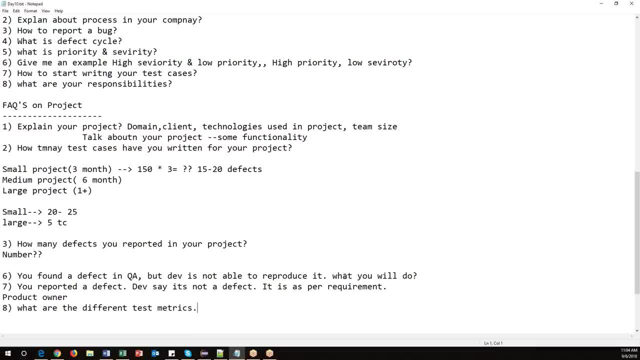 So along with this, I will also send you a few documents. Those documents are having hundreds of questions. You need to prepare all of them, but this is not finalized. I'm just Only very high level. very important, very crucial questions I have collected from many number of interviews. 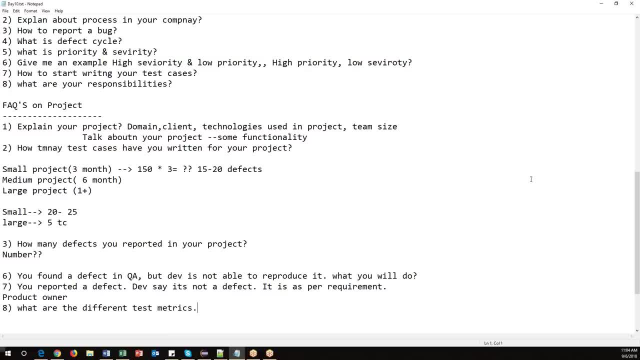 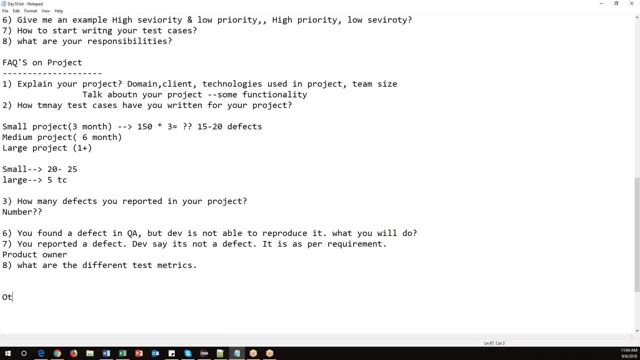 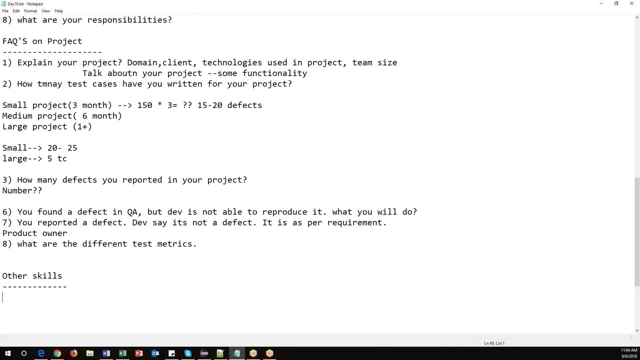 and then I have covered here, Okay, and, but along with the manual testing you should also have another skills, very important skills. So what are the other skills you require Along with the manual testing? so automation skills, anyway, will be there. without automation, manual testing alone cannot survive in the company. 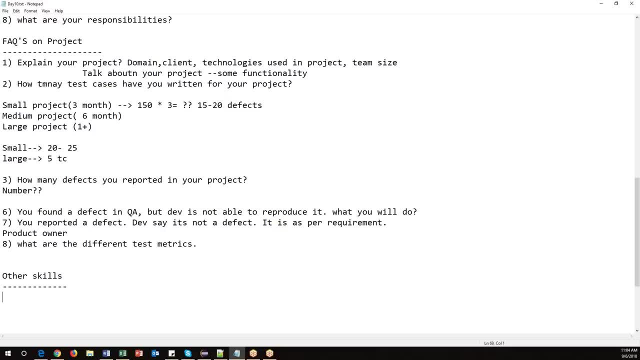 So you not get any cause with manual testing alone. So you must have automation skills, but additionally you should have a sequel. SQL knowledge is required. You should able to write all the queries. Okay And okay. the those is asking question: which domain is best for facing? any domain is fine. 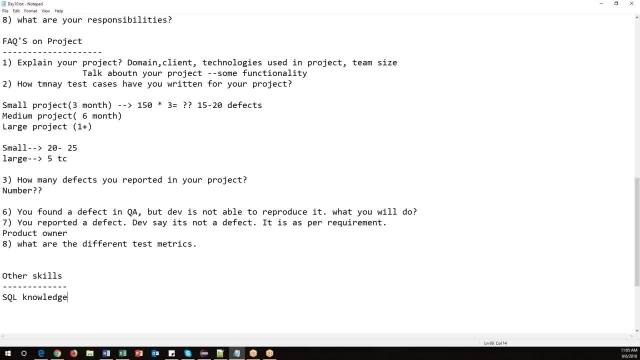 Tulsi, it can be banking domain or financial domain and e-commerce domain. Okay, any domain is almost equal importance. Okay, but the health care is little piece, a little bit complex, And the first domain when you come back with other domains. because if you want to put any health care related projects, 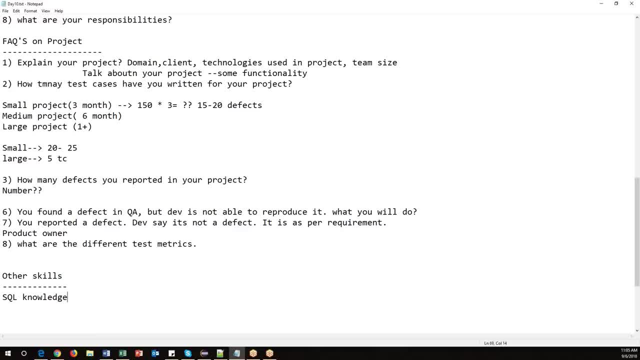 you need to know the complete, you need to have the complete medical background. Okay, so those terms you have to be very clear. So those terms are very difficult to pronounce. answer. So don't always prefer to go for either e-commerce domain or financial or banking domains. 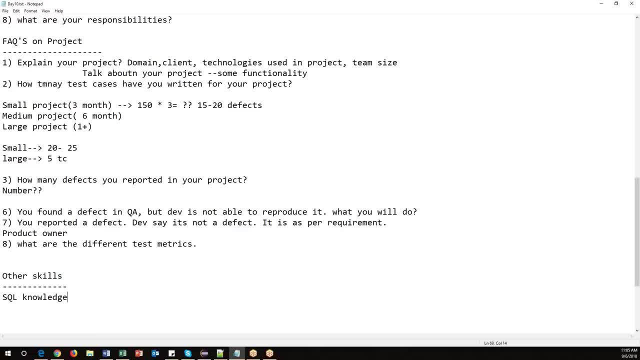 So will be very efficient. Okay, so you can easily get and you can easily answer those questions And especially banking domain is having more importance- e-commerce and banking domain, because nowadays all the applications will be either part of e-commerce and all financial banking companies, right? 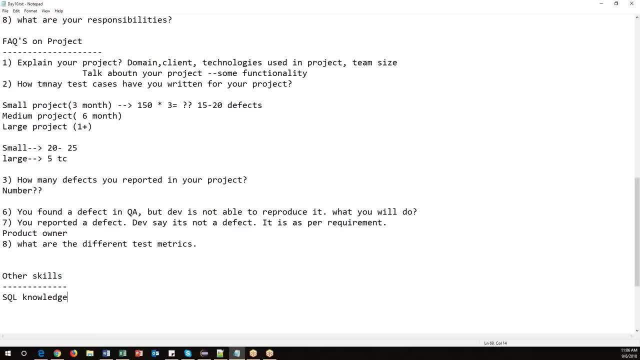 So just go for this. So, along with this normal manual testing skills, you should also have a sequel knowledge, So you should able to write all the sequel commands and if you don't know about the background of a sequel, so I have already uploaded videos in my YouTube. 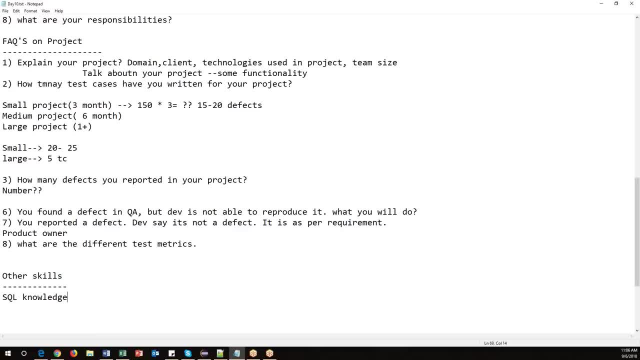 So you can just go through all the sequel videos. So almost seven to eight videos I have recorded and uploaded. each every video will be around one to one and a half hour, So they are live sessions actually. so I can just go through those videos and get the knowledge on this. 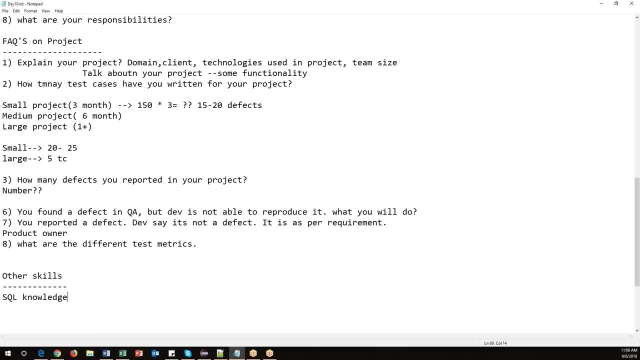 Okay, very important topic, So it's equal. also, you will get the questions on this and other things. like a Microsoft Office, You should able to do the documentation, So documentation also very important. So whenever some meetings and lap and review meetings and all, you need to able to prepare the presentations. 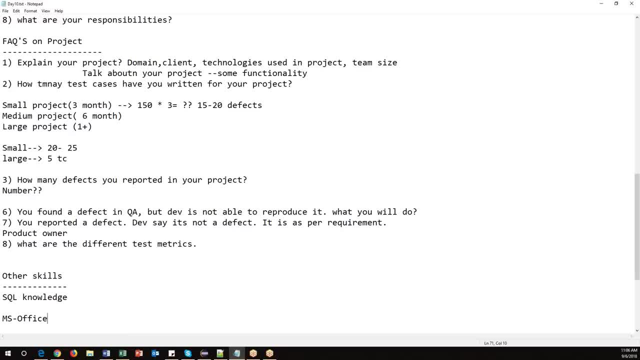 and unity, able to create some documentation like: whatever the job you have done, whatever tasks we have completed, You need to present that task to the team. So in those cases, you should able to prepare a proper presentation. So you need to also have the presentation skills. 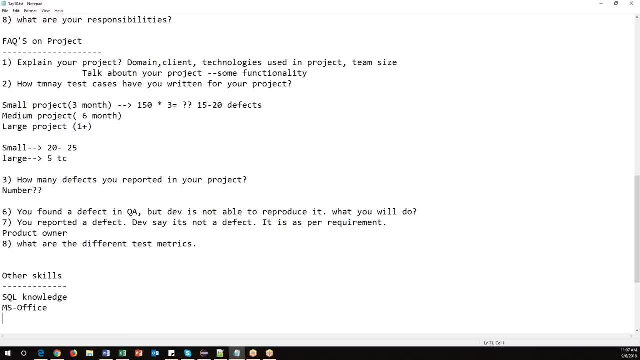 and documentation skills already. These are all things are required and you need to also have some knowledge and web technologies. So web technology in the sense, like HTML, all the web pages will be designed. Okay, HTML, HTTP, HTTPS, Okay, all these things. 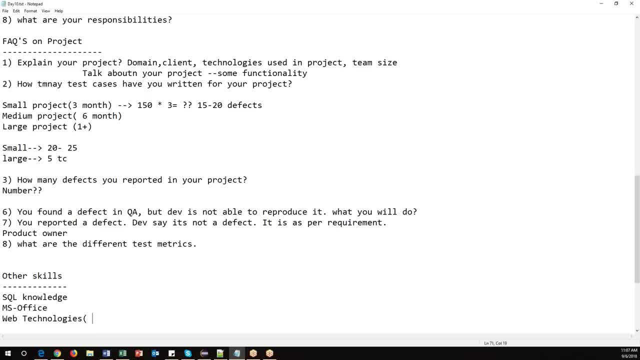 Be very useful. and website technologies in the sense web services, web services and the API testing, API web services, the back-end testing. So what is the web service? What is API? So these knowledge you should have, at least minimum Okay, even though if you're not working on those technologies, 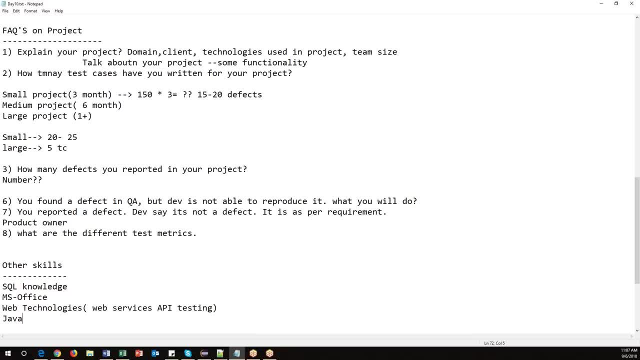 at least you should have some knowledge on this, and is a programming skills also mandatory? basic programming skill You should have, but if you go for an automation, the program is will play very important role. Okay, so these are all important things which we need to remember. web technologies: 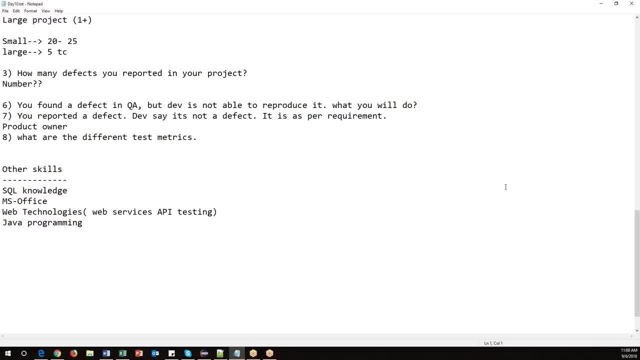 because whatever applications you are testing, they are all web based applications, right? So that's the reason you should also have the web technologies, because at the time of deploying your project in your QA environment, all they will use some web services, web technologies like Tomcat server and web logic server. 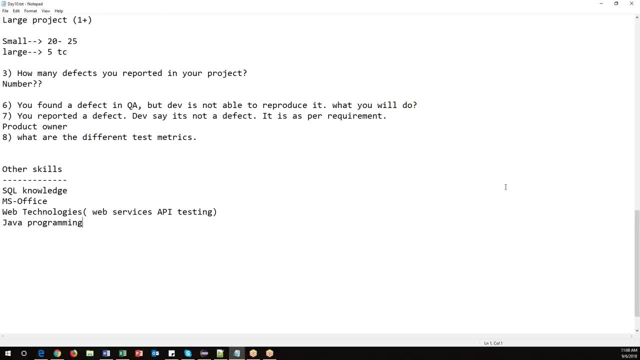 So those things they will use, Okay, so that's the reason you should also have knowledge on this, Okay, No, no, no, you should not think about: okay, your scope is, should not think your scope is very limited. Okay, Nowadays testing is not like that. 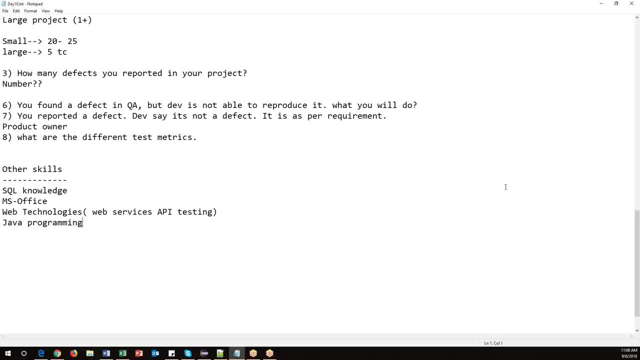 So testing is not only testing. you have to do a lot of things. Okay, you have to do a lot of things. So nowadays, testing means your scope is not limited. You should know the database side, You should know the web technologies, You should know the testing part. 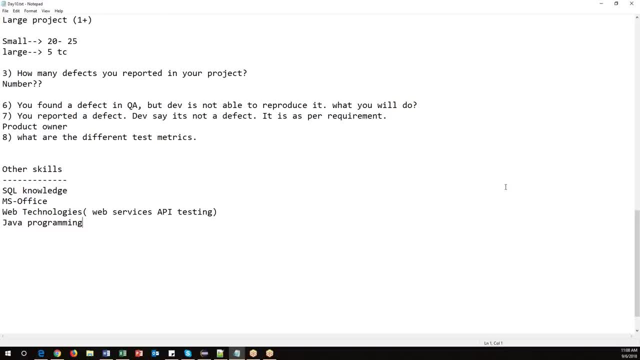 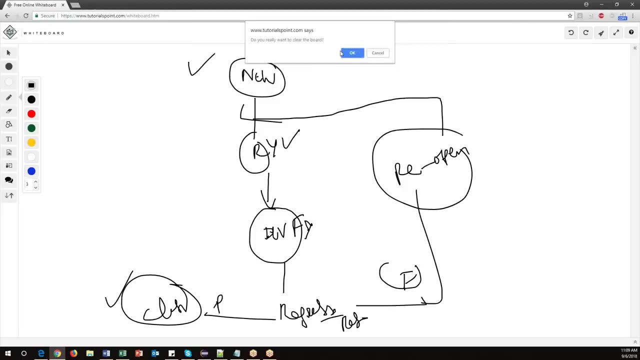 You should know also development. You need to know about Jenkins, maven, all the continuous integration process. Okay, you should able to automate your test cases. So almost nowadays, tester and developer is almost equal. Okay, So why I'm saying is agile team. 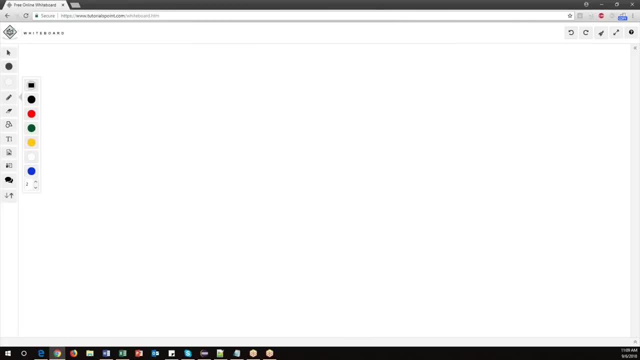 There is no testing, There is no development. Everybody will consider the same. but who is having their own skills? They will work on those tasks. That's it. Sometimes the developer will perform testing, Sometimes the tester can perform testing or tester can develop the code. 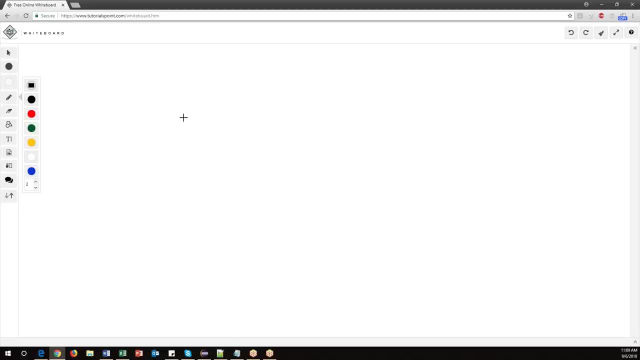 So these things will happen in the agile process. So here, Why I'm saying developer and testers almost same is because, suppose, if we take an, a product or software, So what the developer will do regarding the software, He will develop the right or he will develop or write the code. 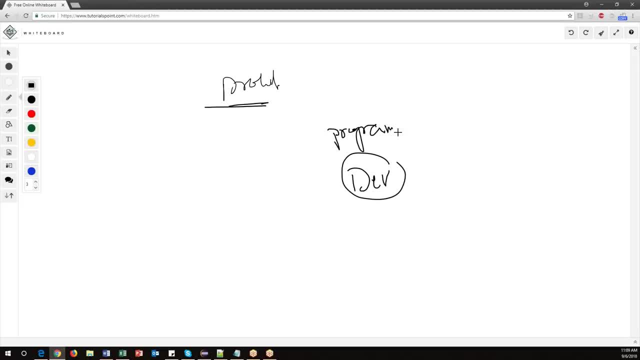 or writing the programs right. So why they are writing the programs to develop this software? Even tester is also writing the programs. What programs tester will write automation? So automation in the sense writing the code. So why we are writing automation code here? 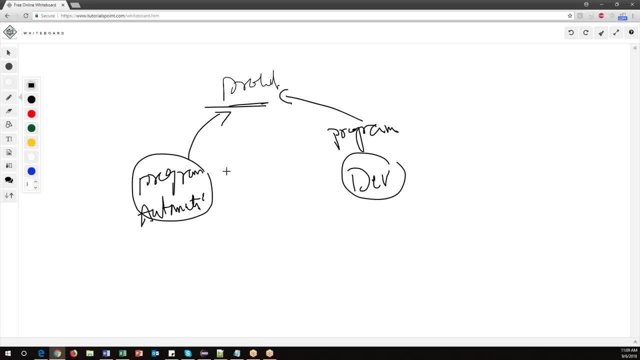 To test the software or test the product. So ultimate goal is same for both. So one is for developing the software, other is for testing the software. Both are writing the code, Both are writing the pro and both are learning the programming. So in this context they are coming closely together and going forward. 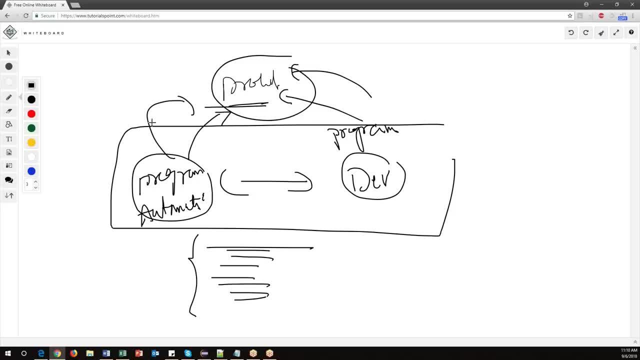 There will not be any specific positions for testing. Okay, everything will be considered as one umbrella and they are calling as a s-date. s-date is nothing but software Development engineer in test. Okay, so there is no manual tester, automation tester. You don't have specific roles like that in future. 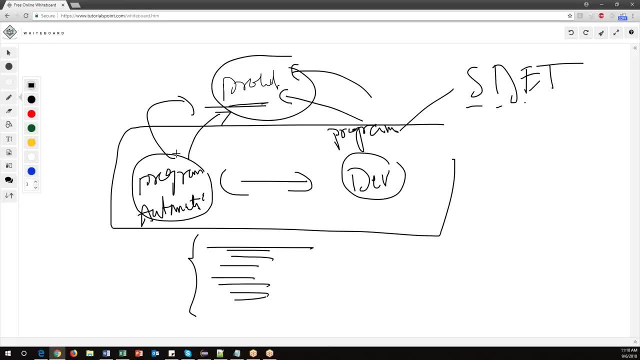 So everybody will consider as a one umbrella and everybody should be having the same kind of skills. Okay, So in the coming future this will be very. nowadays, No one is asking very less number of companies still asking for automation tester, senior automation testers, like this. 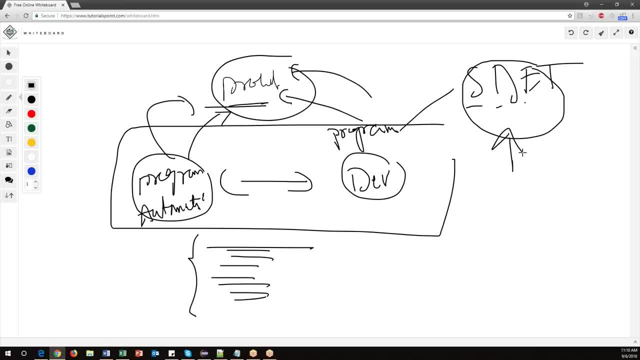 but most of the companies nowadays are moving to s-date. s-date is nothing but software development. So they should have all kinds of skills- testing skills as well as development skills- and they should have knowledge and programming: web technologies, database skills, with data, how to all the stuff- and web services- everything. 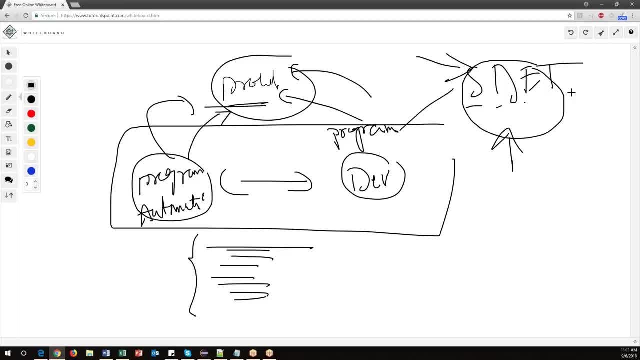 So people are marketing or expecting these range of skills nowadays. Okay so, don't limit your scope and always try to expand your scope. Okay so, so you should. it's very good to know all the stuff, but you should be very familiar in depth in one thing. 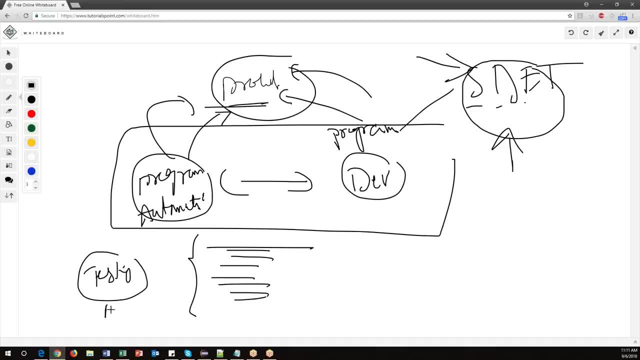 Okay, so testing your core domain, So you need to all know the manual testing plus automation, your core concept. You should know you should go deep in that. but other than this, you should also ever have other technologies, like web services thing. What do you pay? testing? 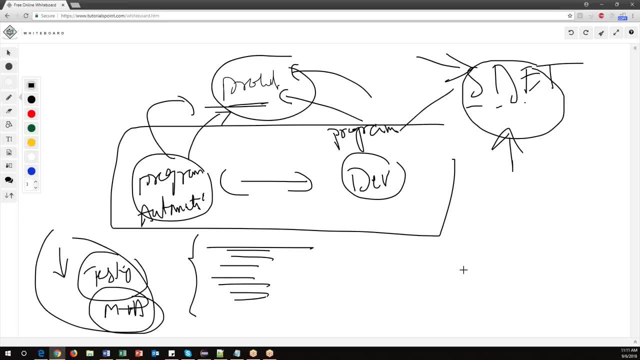 What is big data? What is ETL testing? What is mobile testing? So all these things you do have. you should have some idea at least, even though if you're not working on that, you should have some basic idea. but the main core, your working area, is testing with automation. 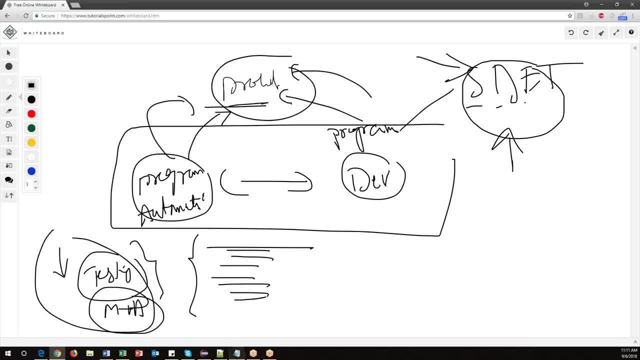 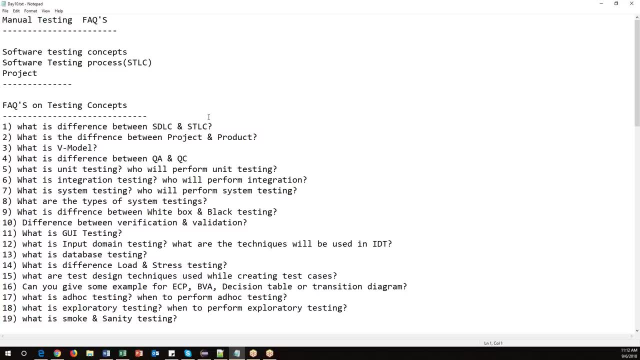 So you need to consider like that. Okay. So these are all about frequently asked questions in manual testing, So I'll just stop it here. along with this, I will also send you a few effect use document. Just please do that. Okay. so web services are. there are two types of web services. are there to see? one is 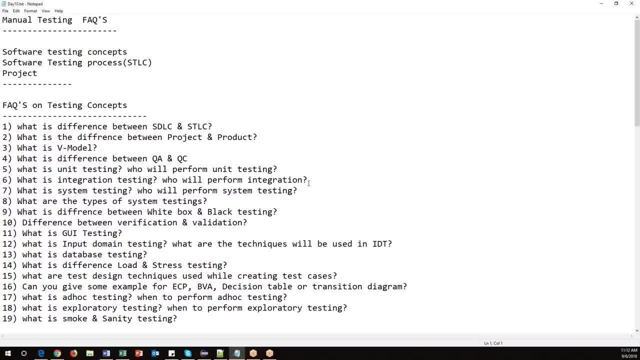 like a rest API or rest services and soap services, and to test those web services We have special tools called soap UI and rest API and postman. So there are some tools are available in the market. So they are completely the back-end testing, not a UI testing. 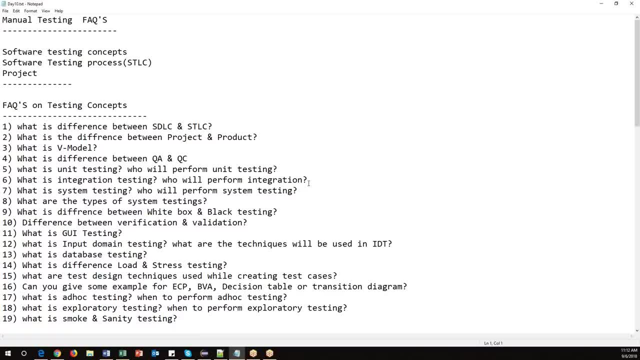 Okay. So whatever testings we are so far discuss is like: functional testing means a UI testing, all the web interface you will test. you need a browser, Okay, but web service is a back-end testing, but web services are not. again, database database is different. 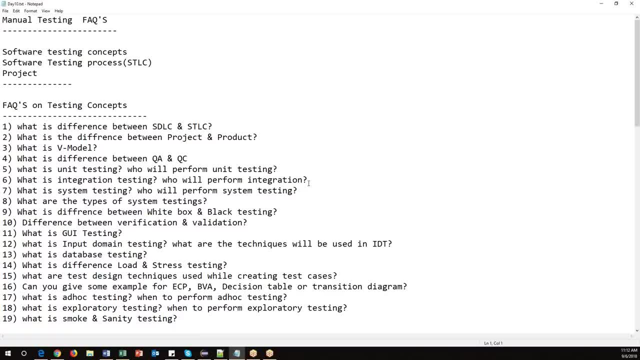 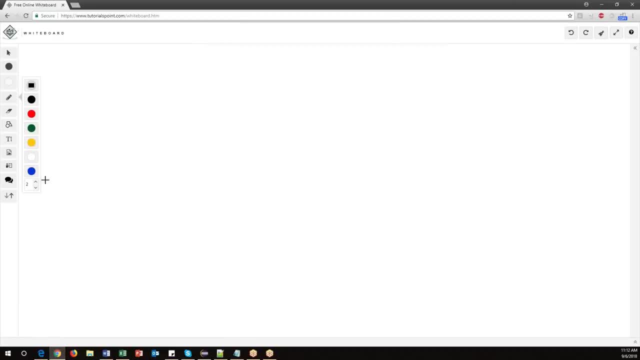 Okay, so there are different layers. We have UI testing is different, web services testing is different, database testing is different. So let me just give you over Very basic, over you, but I'm not going in deeply because this is a bigger concept. So currently all manual testers. 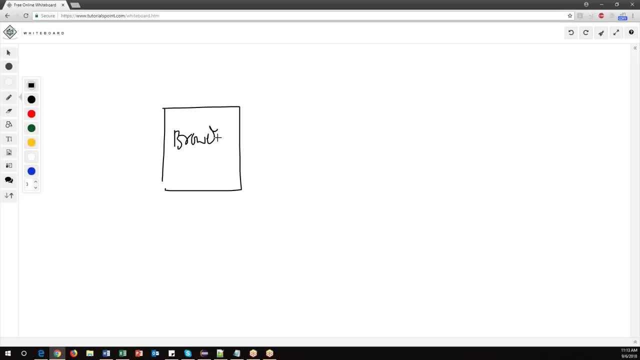 and automation testers on working on the browser. these we need because everything we can see in the browser only and these browser pages. where we are getting these browser pages? We are getting these all web pages from some server. There will be some server. Let's say this is a server. 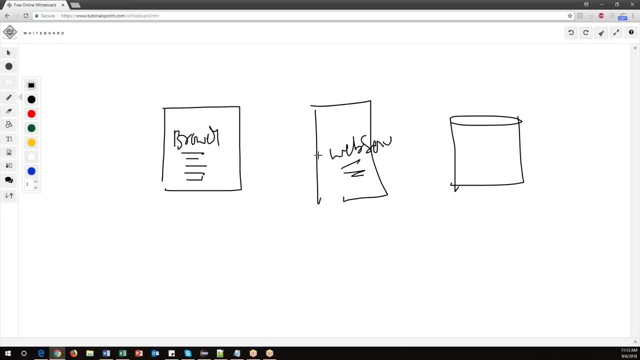 This is called as a web server, And from this web server all over actual pages are loaded here. They will install the web application. So by using this URL we are accessing the web pages which are already present in web server. right, But again, if there is any data present, 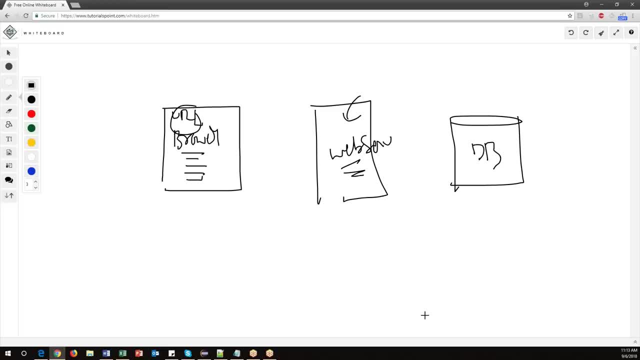 so where the exact data is present, data is present in the database layer. This is exactly, data is present And if you pull this data, there is a web services, written web service, internet in a small kind of program and this web service is responsible for pulling the data. 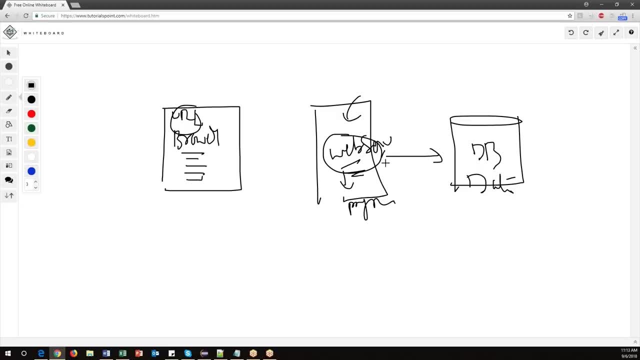 and pushing the data and do the updates and all these things will be Taking care of it and here, whatever the data you are getting from the database will be displayed on. the UI is understandable format. We are easily understand or identify all the images, elements, text boxes, links, everything. 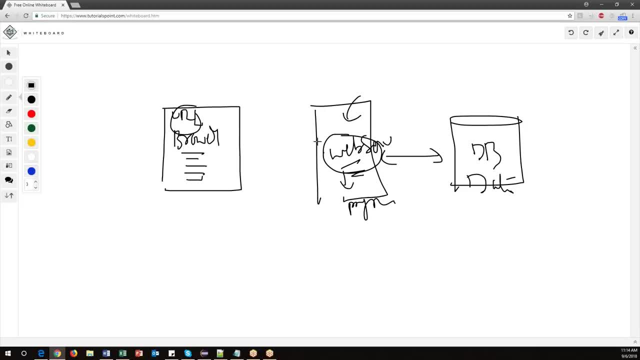 So whatever data this web service is getting from the database will be presenting in the UI. So currently we are working here in this area. This is called as a UI testing. So all the QTP and selenium, all the manual testing, will be done. 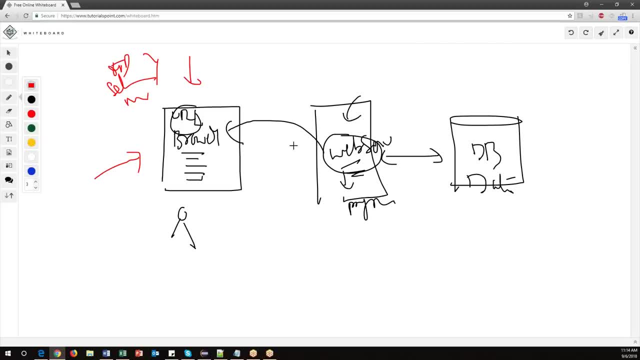 On the UI side. This is one area of testing And nowadays people are slowly going to API testing. So instead of testing this, this is also there. This is also much important because sometimes API is getting the data, but it is not properly presenting in the UI. 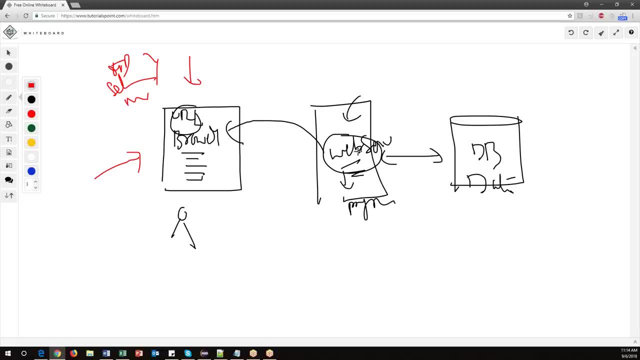 So those kind of issues we cannot find using back-end testing. So we must do the UI testing that should be there always. and there is another kind of testing called web services. testing your web services means these web services reset in the servers. So this is the actual component which will get the data. 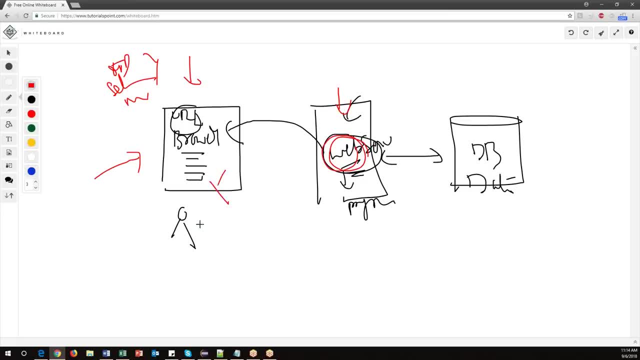 from the database and presenting to the browser. So instead of testing this UI, we are directly testing this web service. So what this web service will do is we will pass some input to the web service and it will produce some output here. So, while getting, this web service will get the data from the database. 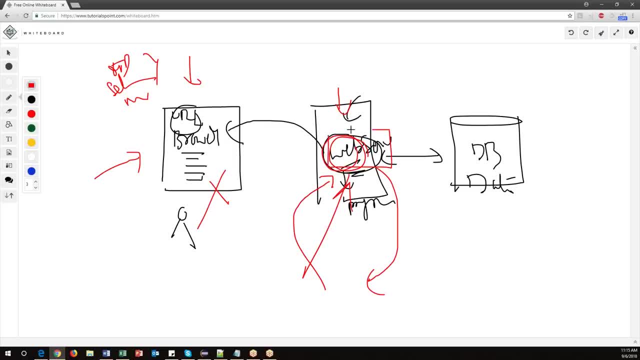 So here we don't deal with any UI thing. So we directly test the XML files and JSON files and to test this web service We have a number of tools called as a soap UI and we have a postman tool like a. let these kind of tools available in the market. 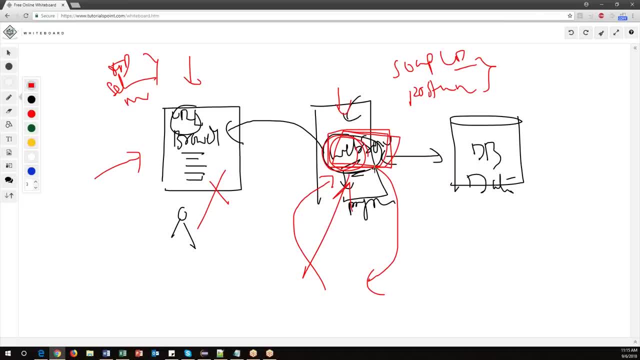 So just to test this web service- web service in the sense It is also an API application programming interface. Okay, it contains some logic inside, but we don't see the what is logic they have created inside by the developer. but we can test this by providing input and getting out.